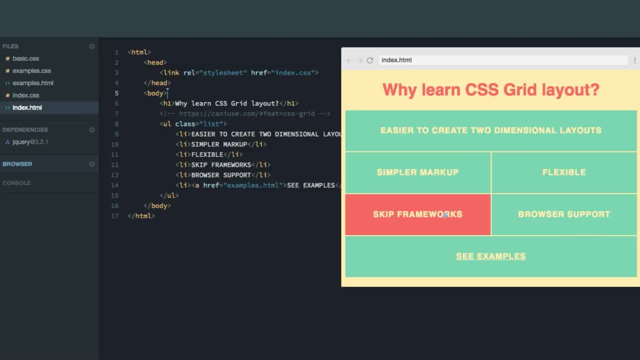 bootstrap, And it'll also enable you to actually skip frameworks like, for example, bootstrap. And finally, CSS grid is now supported by all the major browsers and the support amongst global website traffic is climbing quickly. To learn exactly how many percent at the time: 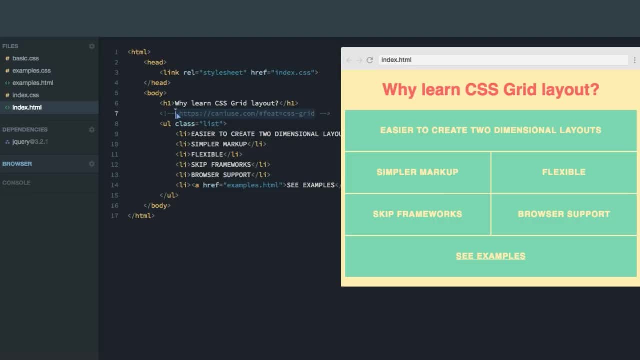 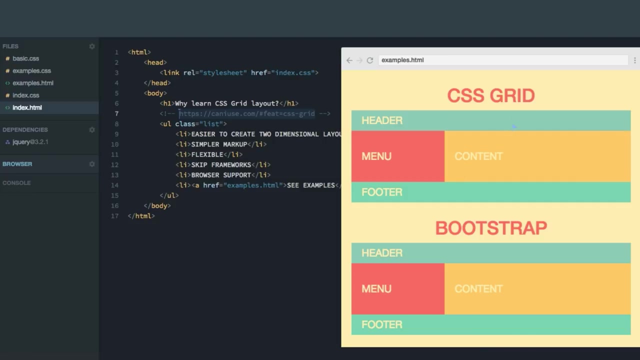 you're watching this screencast. check out this URL here. Now let's kick off the course by looking at the benefits CSS grid has over a framework like bootstrap. Here we have created two mockups for a website. This one is done using CSS grid And this 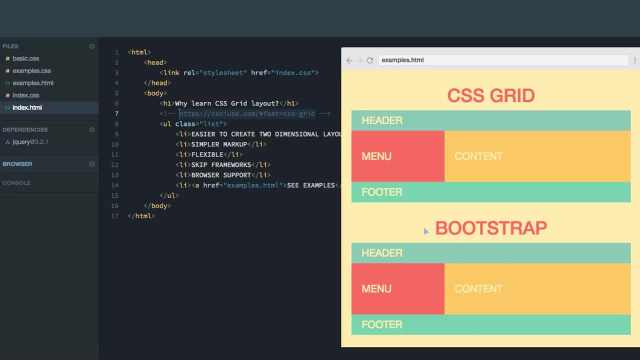 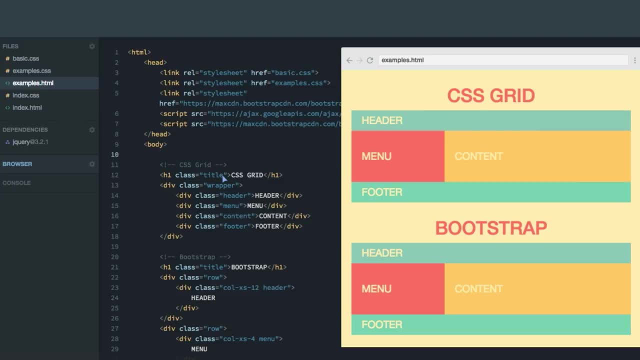 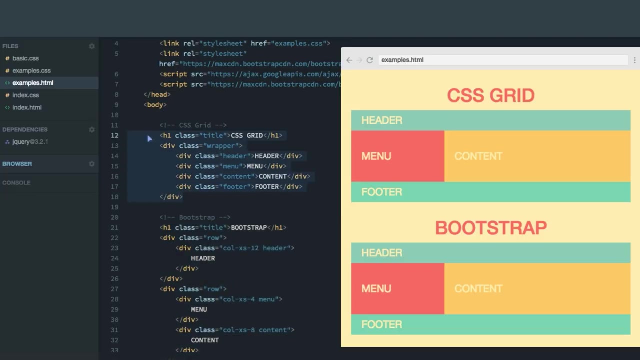 one down here is done using bootstrap. The layout contains a header, a menu, content and footer. The markup is found in the examples dot HTML. Here you can see the HTML for the bootstrap example And here we have the HTML for the grid example And we can instantly 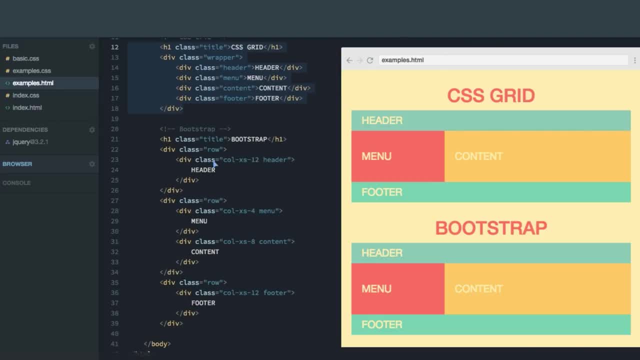 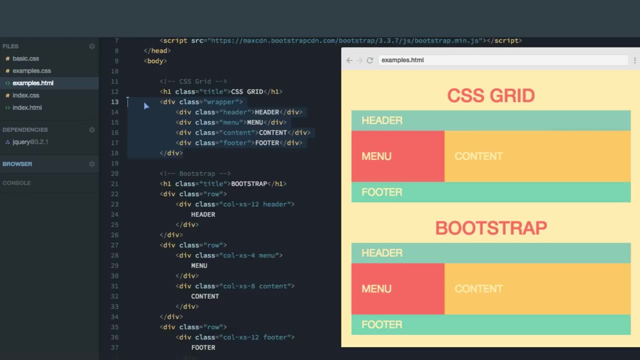 see that the CSS grid markup is significantly simpler- Simpler than the bootstrap markup Because gone are all the unnecessary row items and the ugly class names. So, as I mentioned, CSS grid will make your markup cleaner, benefit which, of course, would become much more apparent if we were to turn these two examples into. 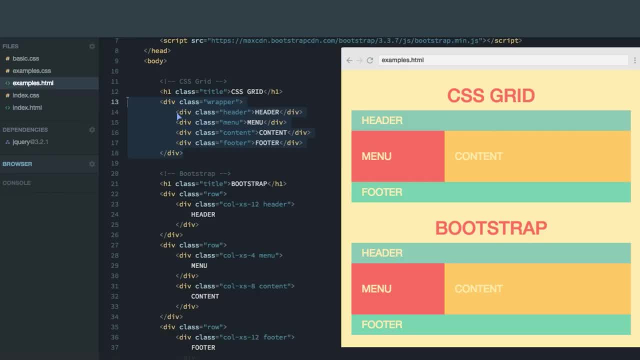 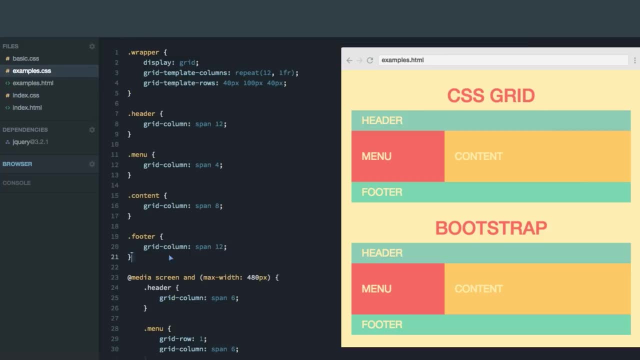 full blown websites. However, this, of course, doesn't tell the whole story, As the grid example of course needs CSS, which you can see here in the examples: dot CSS. Here is the CSS grid As needed to create our grid example Conceptually. what's happening here is that, instead of trying, 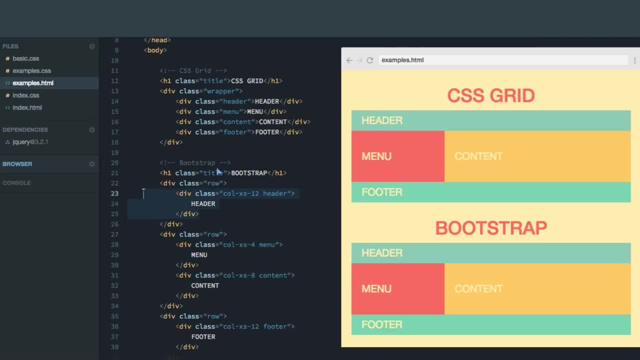 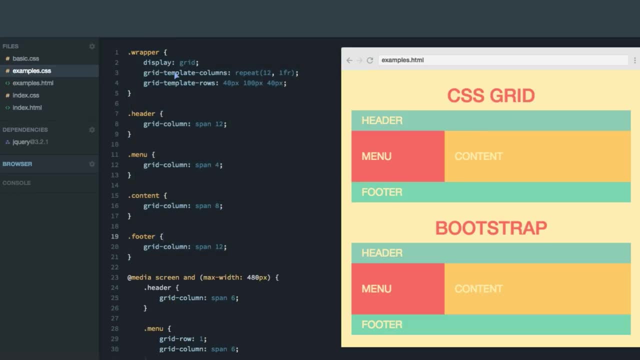 to define the layout, which is the columns and the rows in the HTML. we're rather defining everything in the CSS, And this brings us to our next benefit, which is that this separation gives you a lot more flexibility. Let's say that you, for example, want the menu here to 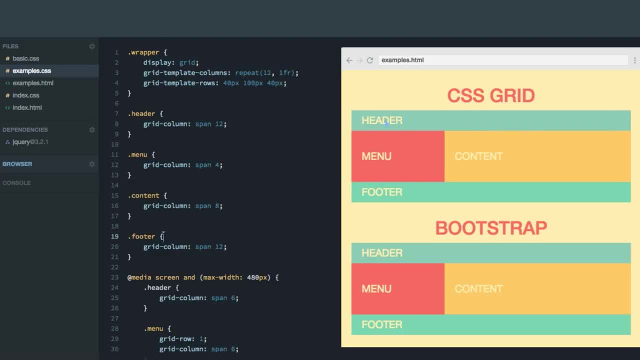 appear up besides the header when it's being viewed on mobile. To make this happen in our CSS grid example, we simply create a media query and then we target the items which we want to change according to the new layout, which is the header, the menu and the content, and then simply give. 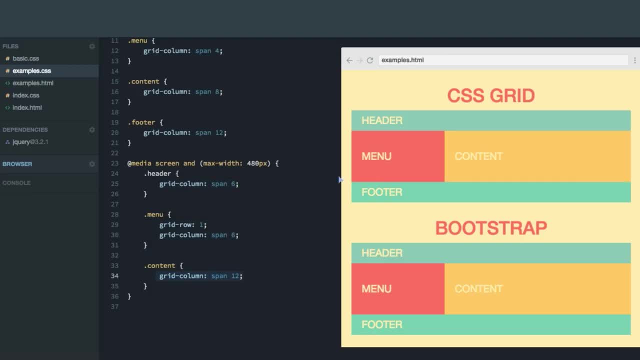 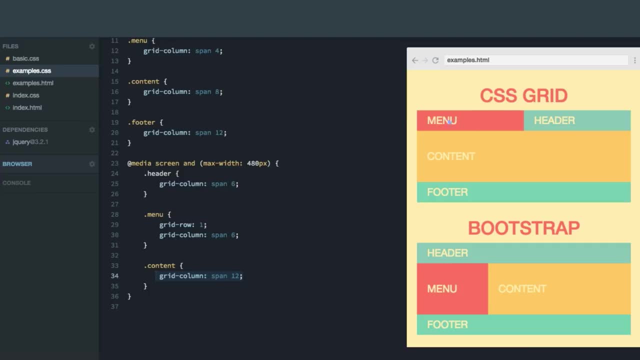 these their new values, And the result is that when we shrink the page and if you look at this CSS grid example, you can see that- boom there, the menu item jumped up to the top row, the header moves all the way to the right and the content took up the entire second. 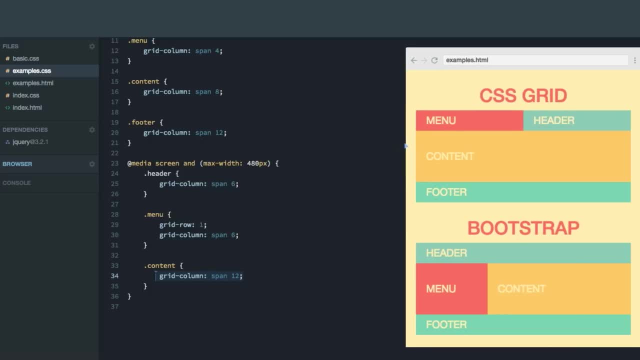 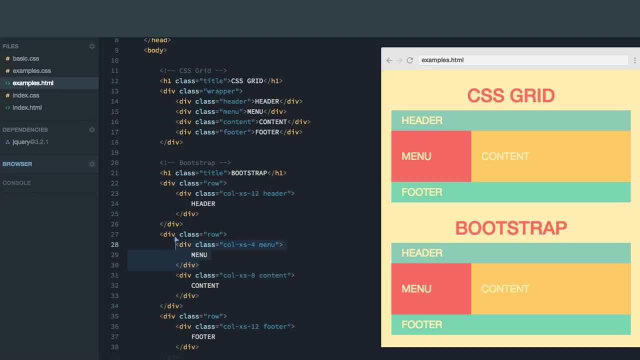 row we can change back. boom like that. Now, if we were to try this in bootstrap, we'd quickly realize the downside of having the layout defined in the HTML, because what we want to do here is to make this menu item jump up to the first row up here. However, that's not trivial, because the menu item 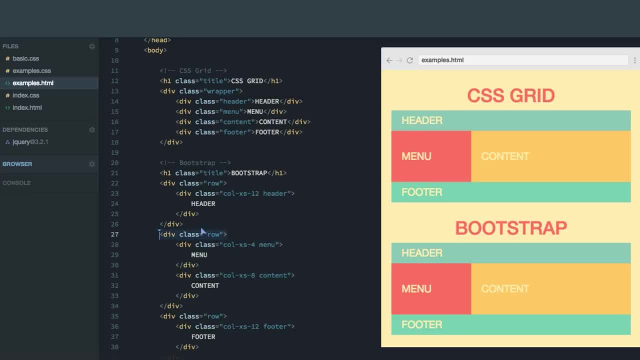 is already trapped in the second row down here, And in order to move it up to the first row, we actually have to change our markup. we have to cut away this element And then if we were to move it down here and paste it in up here, That's not something you can. 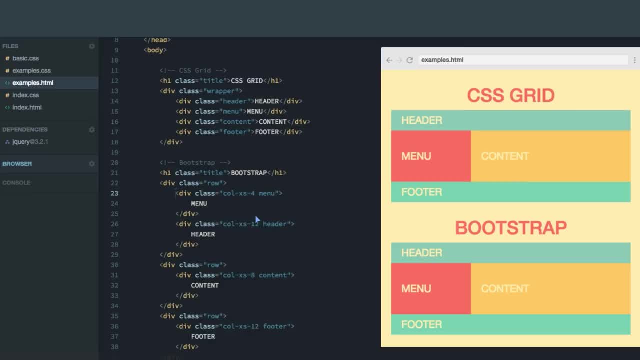 do based upon a simple media query in CSS. You can, of course, do it in JavaScript, but that's hacky and more complex, So what you want to do instead is learn CSS grid, And I'm going to teach you that in this course. So just sit tight and we'll start the next. 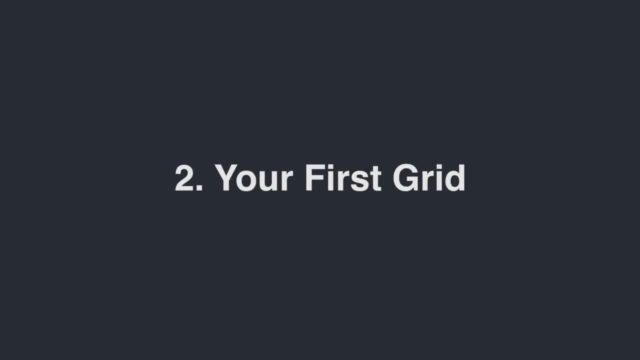 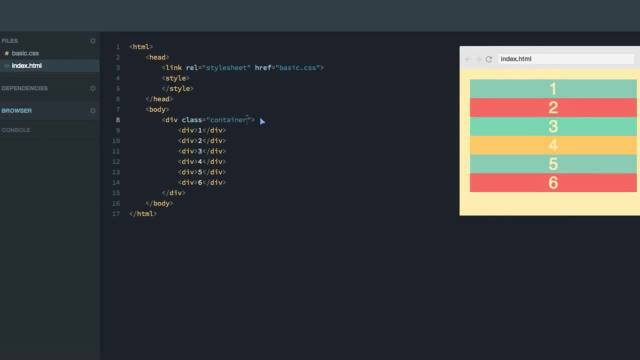 lecture right away. Hey, you're going to learn how to create grids through defining its rows and columns. A grid consists of two main elements. There's the container, which we have here, And then there's the items, which are the elements inside the container, in our case, six divs which display the numbers from one to 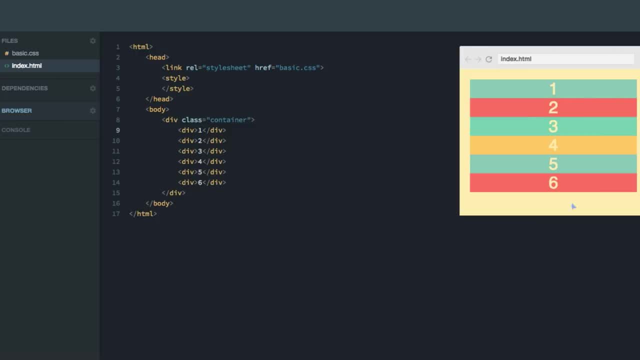 six Now, without any grid layout, this results in six divs stacked on top of each other. I've also given them a little bit of styling, but that has nothing to do with the grid layout itself. To turn this container into a grid, we're going to target it and give it a display of grid. 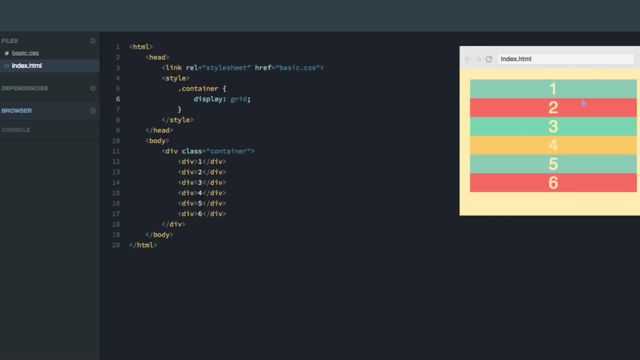 We run the code that won't result in any layout change yet, because we haven't defined how we want our grid to look like, So by default it only has one column, And thereby it looks like we've just stacked six divs on top of each other. In order to specify the columns, we'll give the. 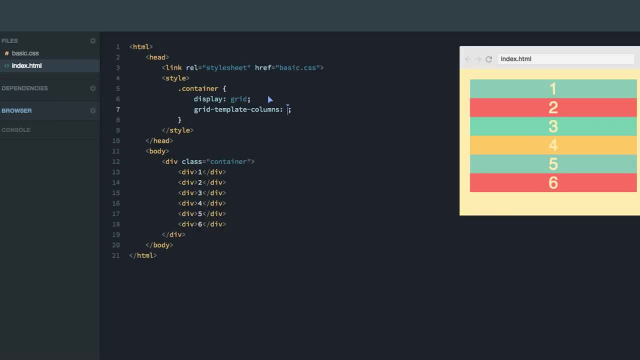 container, a grid, template, columns, And then we define how many columns and how wide we want them to be. Let's set the first one to 100 pixels, the second one to auto and the third one to 100 pixels as well. Auto in this case, means that 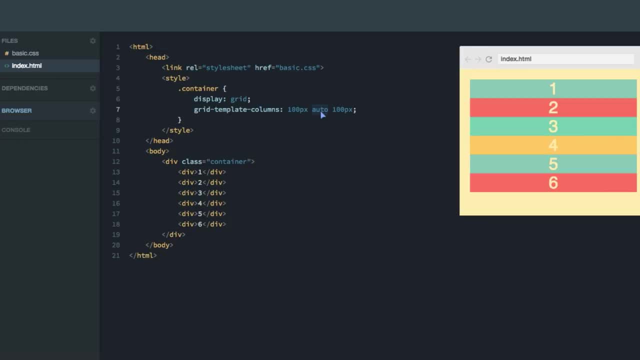 the column will take up whatever remaining space there is in the width. Let's also give the grid a couple of rows- template rows- and let's give both of them a height of 50 pixels. So in the grid template columns property we define the width of the columns And in the grid template rows to define the height of the rows. 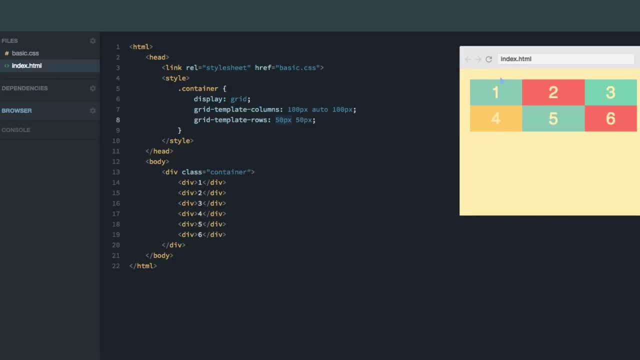 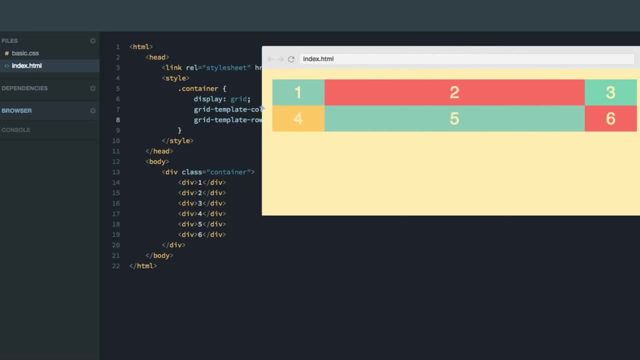 And, as you can see, we have a nice little grid here. As expected, it contains three columns going from top to bottom, 123, and two rows going from left to right, 12.. Since the second column here is set to auto, this grid is also responsive. In order to make the grid look a little bit nicer, I 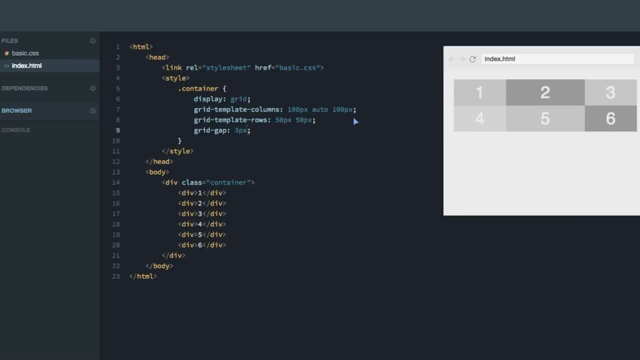 want to give it a grid gap property. Set it to three pixels. As you can see, that gives nice little gap between the items. Now let's say we don't want our grid to be three columns wide and two rows long, but rather two columns wide and 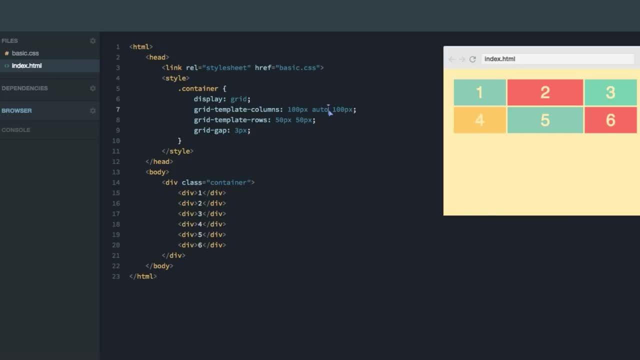 three rows long, then we simply need to remove a column. we can remove this last one here, for example, and add a row 200 pixels down here. If we run the code, you can see that we have a completely different grid: two columns. 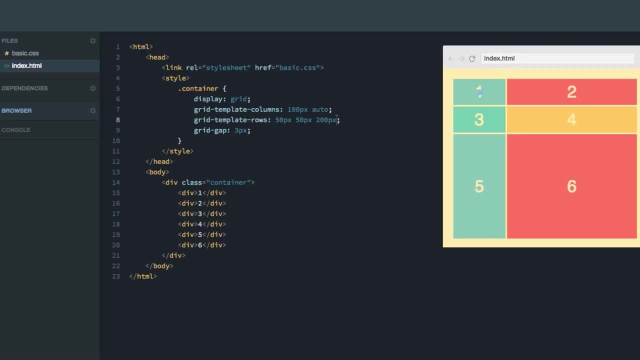 and three rows 123.. The two first rows are 50 pixels tall, or the third one is 200 pixels, And the grid is still responsive as the second column is set to auto. So in the next screencast I'm going to show you a few more ways of setting these values inside the template columns and grid. 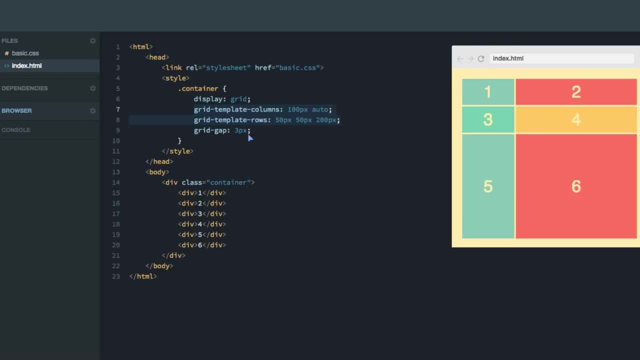 template roles. But before we jump on to do that, I would recommend you to jump into the code here and play around with the values So that you're 100% sure that you understand the relation between what's going on here in the CSS and how that plays out in the 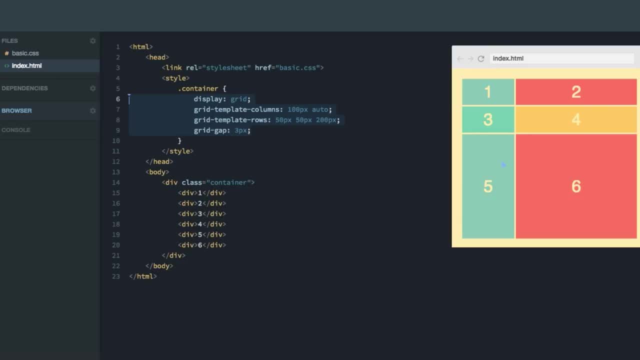 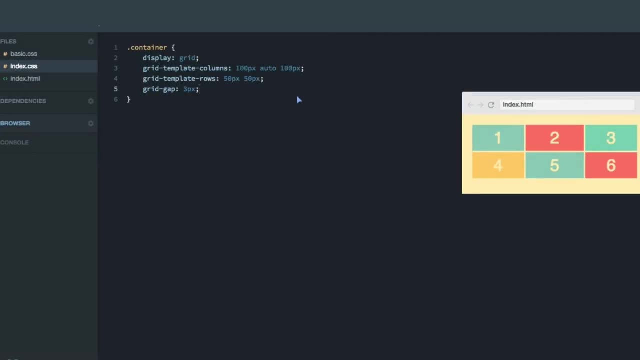 simulator over here, So go ahead and do that, And I'll see you in the next screencast. Hey there, in this screencast I'm going to teach you a better and more powerful way of defining columns and rows. As you can see, we're now working in the index dot CSS file and not directly in the. 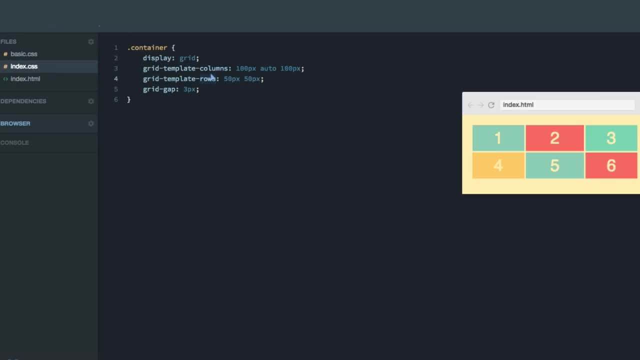 HTML file, As doing it in the index dot CSS gives us the benefits of automatic updates in the browser window. So we have this very simple grid here, which you probably recognize from the previous cost to got three columns, the first one being 100 pixels wide, the second being auto and the third 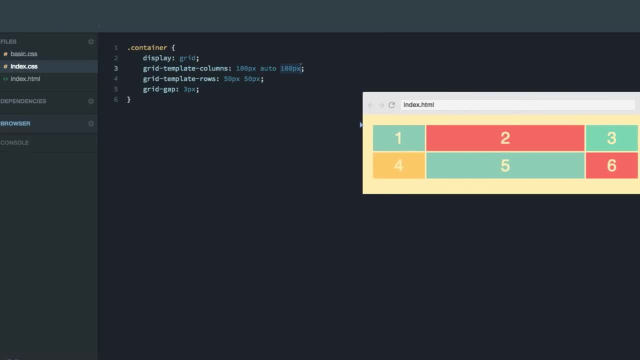 is set to 100 pixels as well, So this grid is responsive as the second column grows and shrinks with the width of the container. We also have two rows which are 50 pixels each. Now the first one is going to change the responsiveness of the grid, Because let's say that we want all three. 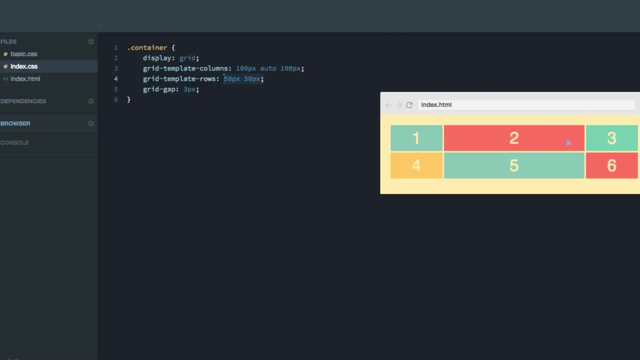 columns to grow in size. as the container grows in size, we want them to be equal, regardless of the width. In order to achieve that, I'm going to teach you a new value which CSS grid brings with it. It's called fraction unit And it's written like this one: fr. Let's set all three columns to be: 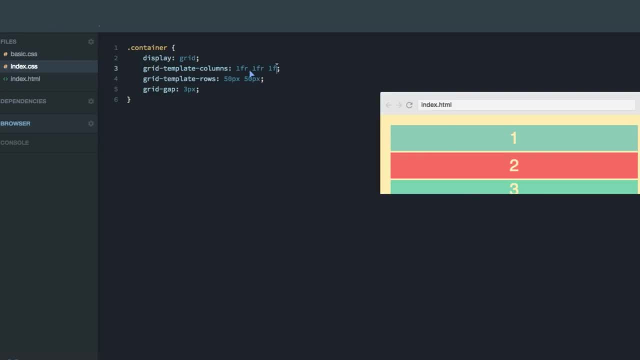 one fraction unit each loop, one fr for the second one and for the third one, And now, as you can see, they all grow and shrink equally. So what happens here is that the grid splits the entire width into three fractions. each of the columns take up one fraction unit. So if we change the second one, 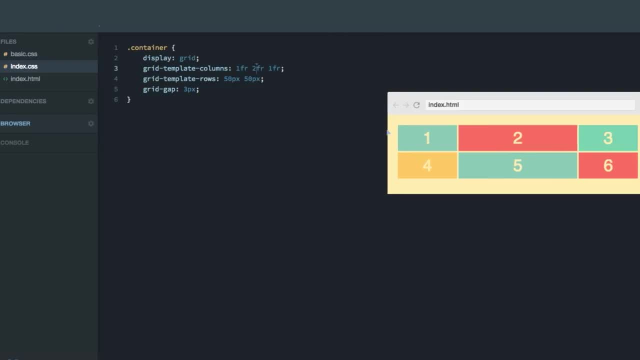 here to two fraction units, you can see that it'll always be twice as wide as the first and third column, Because now the grid has split the entire width into four fraction units And the second, one and third column take up one each. Okay, so let's go back to having each of the columns equally. 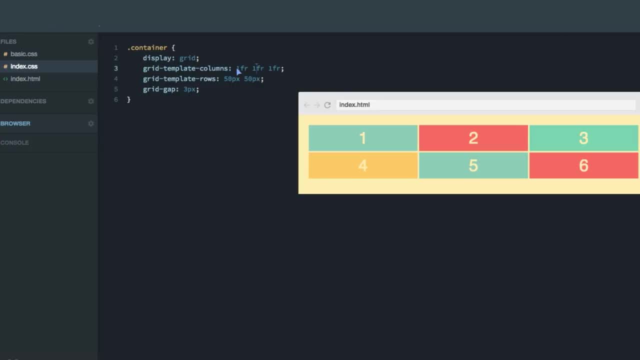 wide. In this case we can actually write this in a simpler way. We can do repeat times, one fraction units And, as you can see, gives the exact same result. So the first parameter of the repeat function is the amount of rows or columns, And the second one is the value, just the height or the 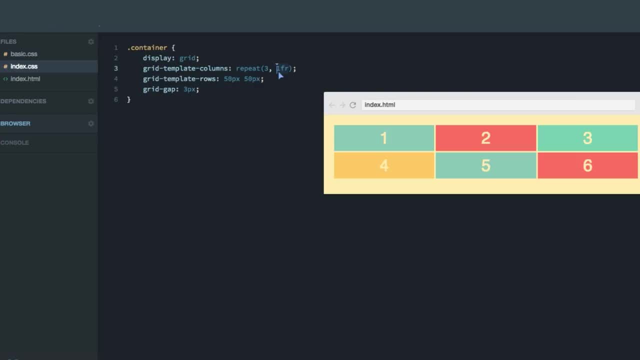 width of the rows or columns. So let's say we want six columns instead. then we can simply change this number here to six instead And, as you can see now our six items fill up only one row, as we have six columns and six items in this grid. So let's go back to three. 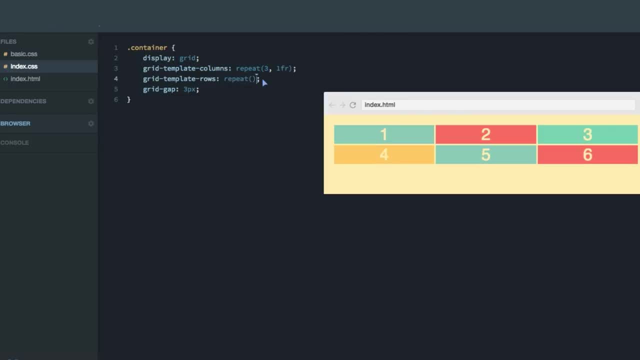 we can also do the same with the rows. of course, it two times 50 pixels. Finally, I also want to show you a simpler way of defining the rows and columns, because we can use the shorthand method for this. So I'm going to copy the rows value here and remove that line. 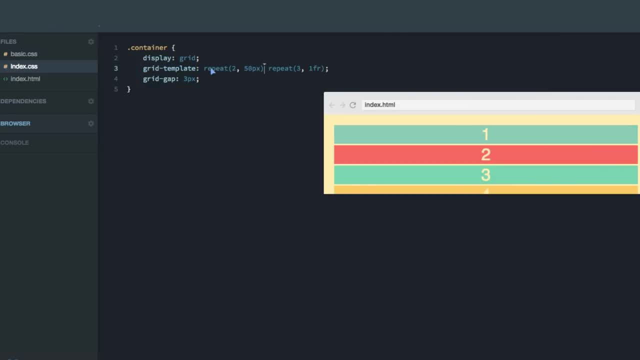 and also remove the dash columns. I'm going to paste in the rows value or slash, and then let the column value come after that And that'll give the exact same result. So grid template is the shorthand method for grid template columns and grid template rows, And it can be a bit hard to. 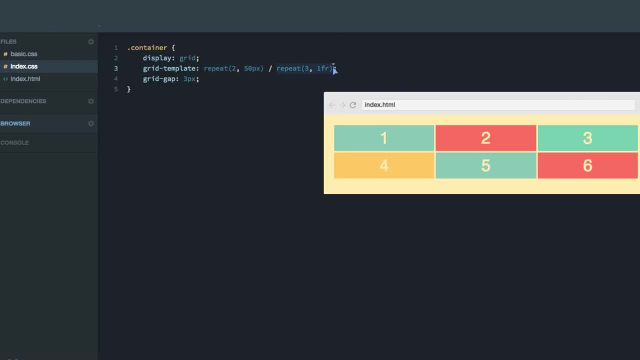 remember which one of rows or columns goes first And which one goes last, And the rule I use to remember this is to think of it as drawing an L: you start at the top and go downwards across the rows And then you go to the right across the 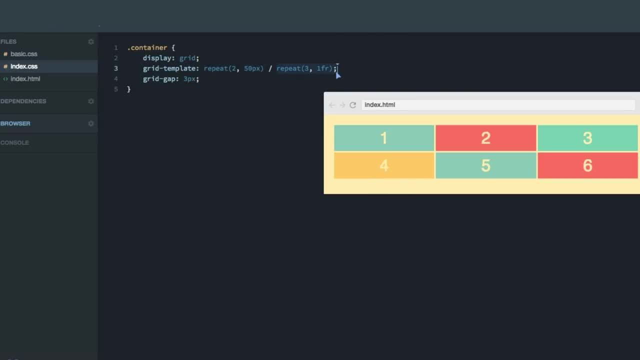 columns. Start with the rows and then the columns. So in the next screencast you're going to learn how to adjust the size and position of the items in the grid. So stay tuned and I'll see you there, Hey. 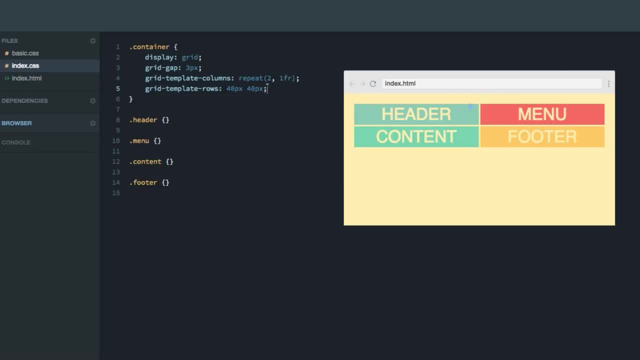 you're going to learn how to adjust the position and size of the items on the grid, which is critical to know in order to create real world websites. with CSS grid, we're going to create a mockup for a website And here in the indexhtml, you can see the 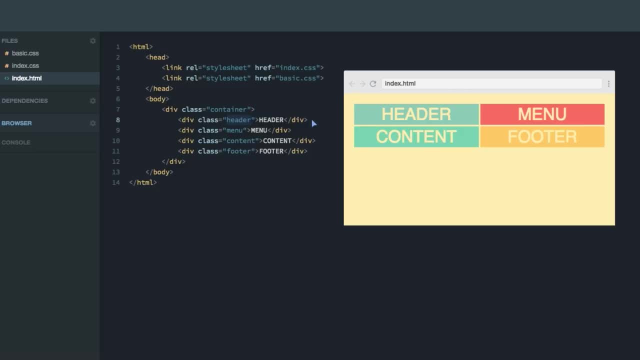 markup for that. As you can see, we're targeting each of the items using a class, name, header, menu content and footer. To start with, we have this two by two grid. Each of the columns are one interaction unit, So they're responsive, as you can see, and each of the rows are 40 pixels tall. 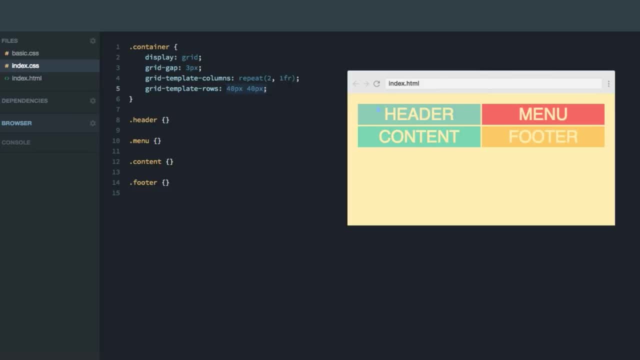 For our website, though, we're going to need three rows, as we want the header to take up the top row, the menu and the content to be on the second row and the footer to be on the third row, all the way at the bottom, So let's create a third row here. let's place it in between the 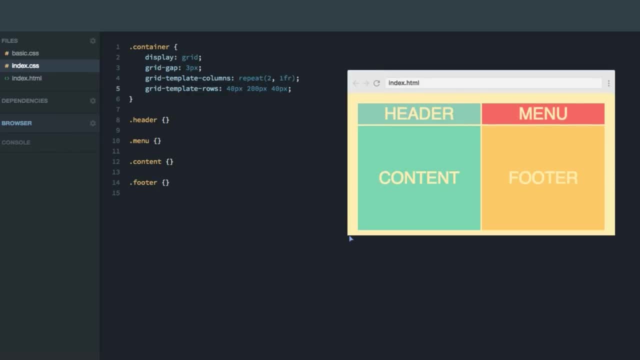 two existing rows and give it a height of 200 pixels. As you can see now, the header and the menu is on the top row and the content and the footer in the second row. And our third row is blank as we haven't filled it with content yet, since our items only take up the first four grid. 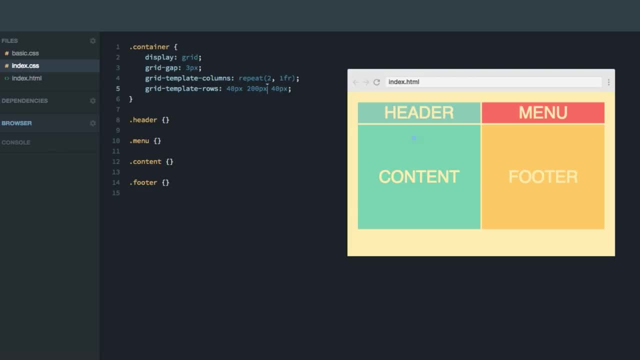 cells. So let's change that. We'll start by targeting the header and making it span from the left hand side all the way over to the far right hand side. To achieve that, we need to head into the dot header and give it a grid column. Arc, set that to one and also give it a grid column. 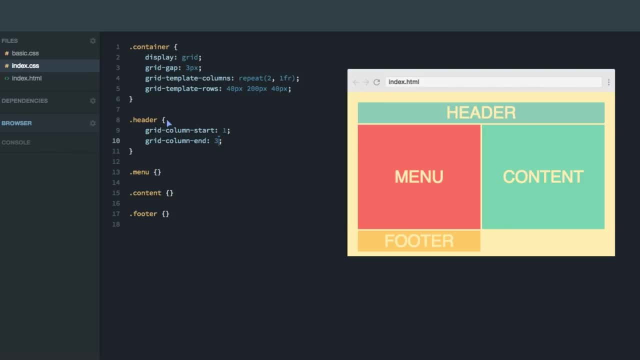 And, as you can see now, the header spans across the entire first row, And what we're saying here is that we want the header to start at the first column line and end at the third column line. And you might wonder why we have three column lines when we only have defined two columns. Well, 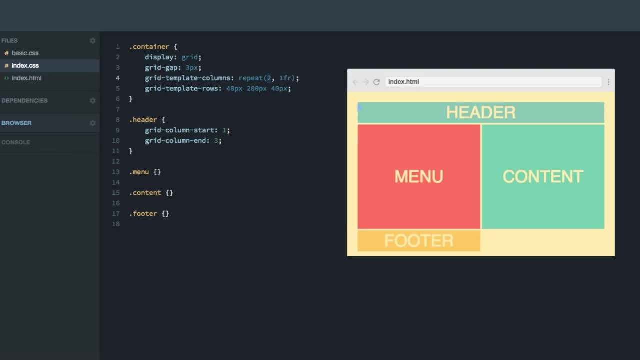 that's because the first column line goes from top to bottom on the left side of the grid. The second column line is the one that separates the two columns. and the second column line is the one that separates the two columns columns. And the third is the one that goes from top to bottom on the far right hand side of the. 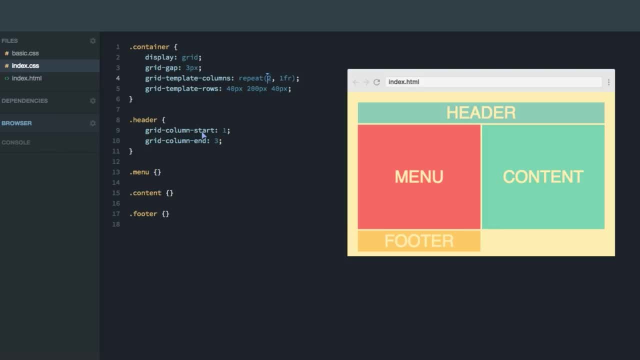 grid, So when you have two columns, you have three column lines, And you can write that like this. Alternatively, though, we can also use the shorthand method, which I prefer. Let's remove this line here And also remove dash start, rather, do one forward, slash three. 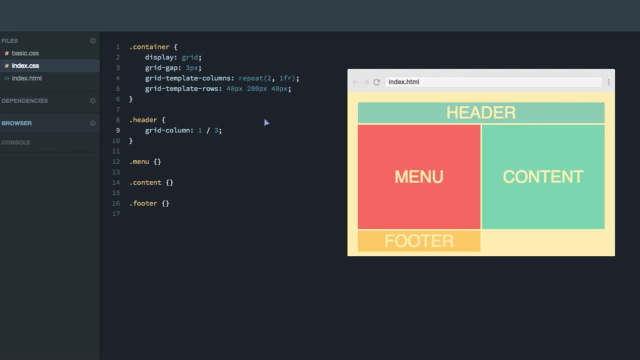 as you can see, that gives the exact same result. Let's also do the exact same thing with the footer. Now, the footer also spans across the entire width. Alternatively, we could have written this in a different way. we could have done. we could have done one forward slash span. 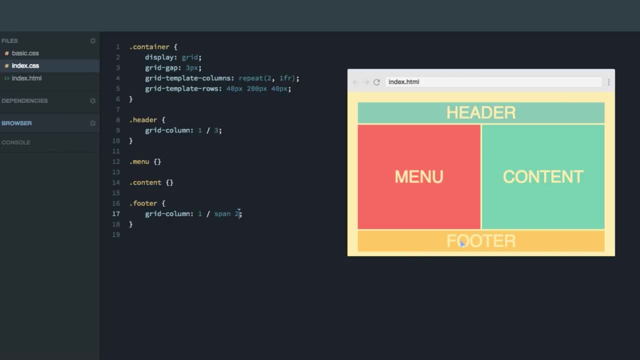 two that'll give the exact same result. What we're here saying is that we want the footer to start at the first column line and span across two columns. And finally, there's also a third way, which is to write minus one. 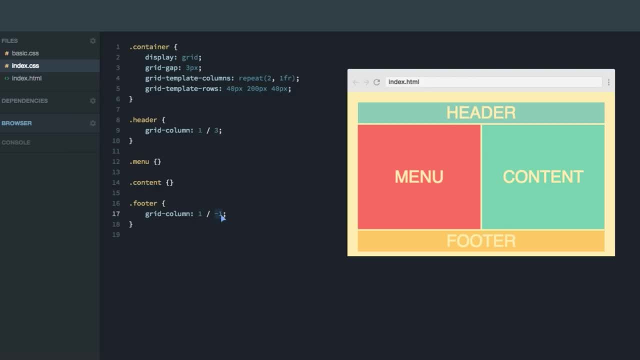 That'll target the very last column line. Now that we know that we want our footer and header to span all the way to the last column line, we can do that with both of them And take the advantage of the fact that in the future you might not know how many columns we're going to. 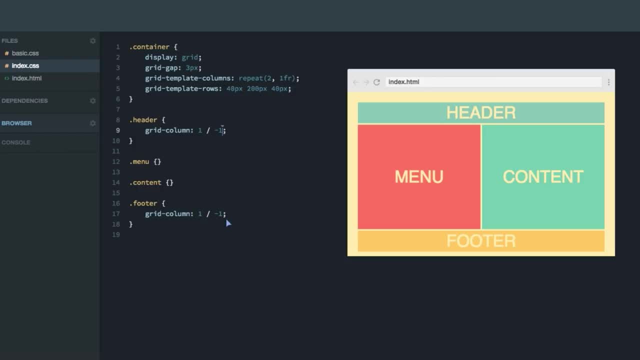 have in this grid, as we can change that however we want. So this is a nice little trick when you don't know exactly how many columns the item will span across in the grid. And to prove that point for you, I'm actually going to change the amount of columns we have in the grid. 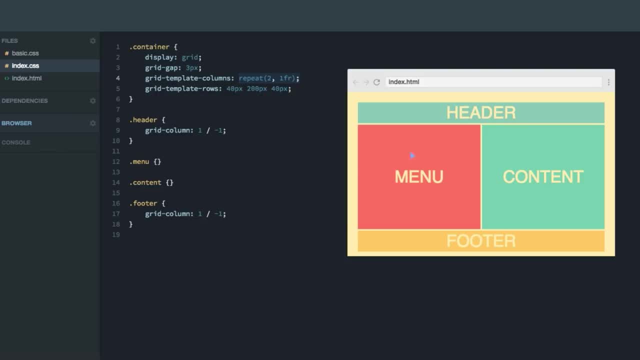 right now, Because we don't want the menu here and the content to take up an equal amount of space in the width. That doesn't make sense. We want the menu to be a narrow sidebar on the left hand side here And we want the content to take up much more space, And we could do this without. 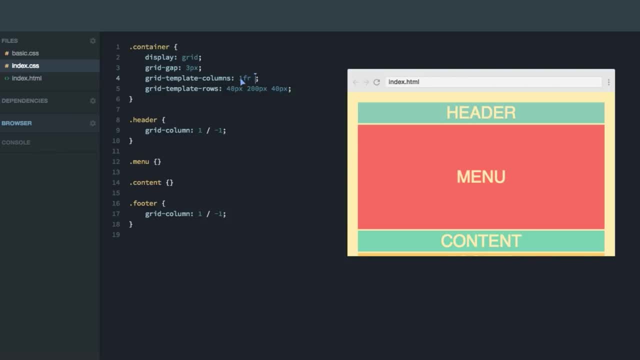 adding more columns by simply doing one fr, four fr, for example. Now you can see that the content takes up much more space, since the second column is four fraction units and the first column is only one fraction unit. However, this is not a very flexible way of doing. 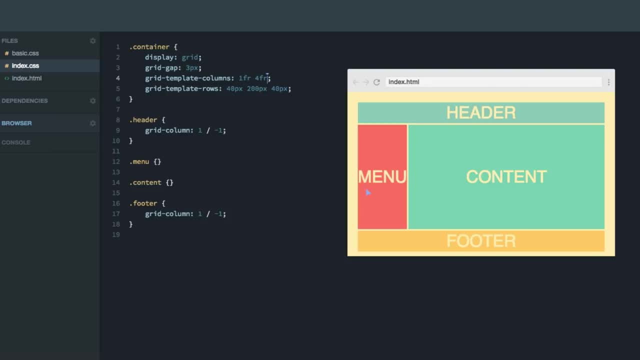 it, Because now we're still stuck with two columns on a website layout And you normally want a lot more columns than that in order to have the flexibility to shuffle around and change the content. So what I'm going to do instead is use repeat. give it 12 columns each of one fraction. 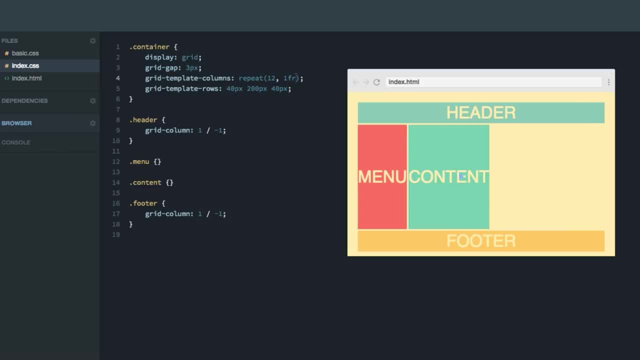 units. Now the menu and the content take up one fraction unit each, in other words, one column each, And they're actually four. So you can see that by moving the columns, we're increasing the columns to be as wide as they need in order to display their content, which is the two descriptions we've added. 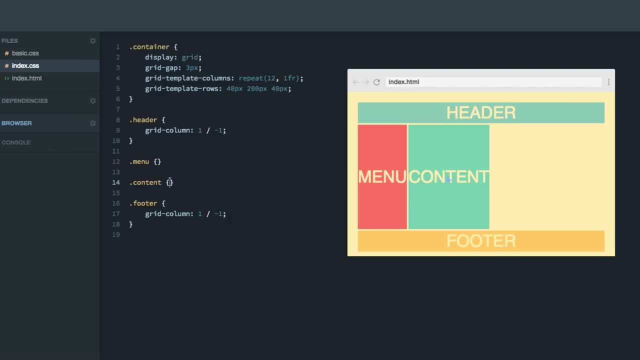 inside items. In order to make this look nice again, I'm going to head into the content class and give it a grid column. We know that it starts on the second column line And we want to go all the way to the final column line like that, So we're going to do minus. 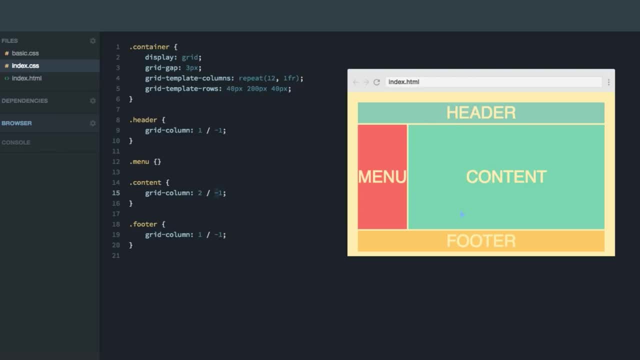 one And now we have a 12 column layouts Instead two column layout, meaning that we have much more flexibility. if you want to shuffle around on stuff And notice that the footer and the header still spans across the entire width, which is 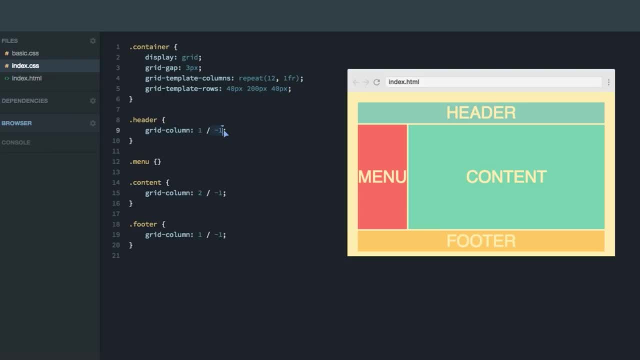 solely because we're using the minus one here. if we had stuck with the three here and here, that wouldn't have worked at all, So let's change it back to minus one. Now. let's also look at the grid row property, as we're going to need that if we, for example, want the menu here to span all the 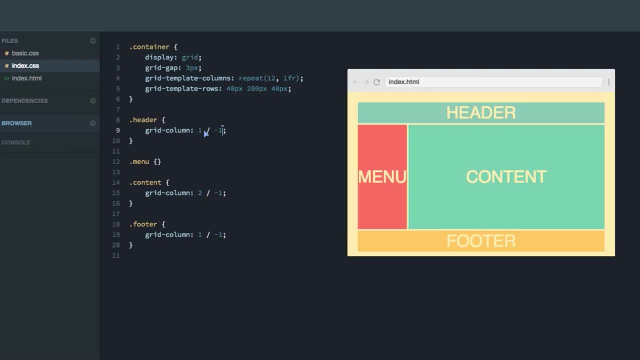 way to the top. In order to do that, we first have to change the header, though, as we need to make the space here available, this little grid cell here needs to be available for the menu, So we'll change it to two. Now we have a blank cell here, meaning that we can head into the menu class and 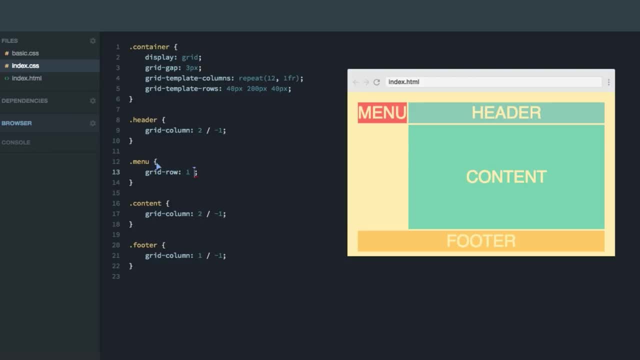 give it a grid row and set that one slash three, Meaning that it spans from the first row line to the third row line. as you can see, took up the spot here in the top left corner because this is the first row line, This is the second And here 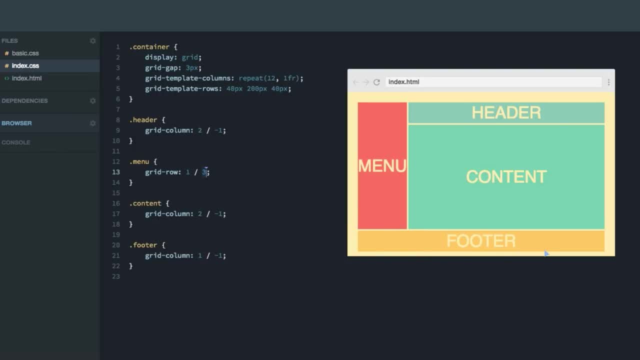 is the third. The fourth then is, of course, the the bottom line. Okay, so before we jump on to the next screen cast, I would recommend you to, for example, try to make the menu span all the way to the bottom, or, alternatively, make it appear on the right hand side instead of on the left hand. 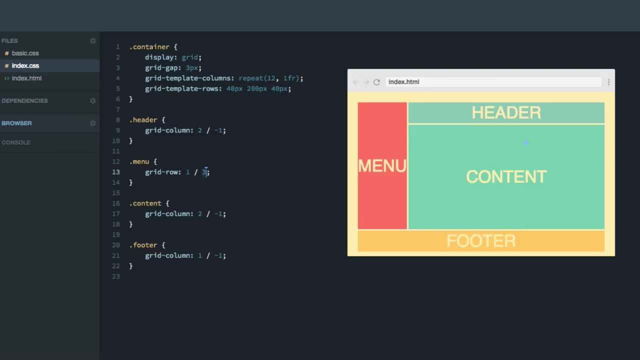 side. And then in the next screen cast, we're going to have the menu span all the way to the bottom. And then, in the next screen cast, we're going to have the menu span all the way to the bottom. And then, in the next screen cast, I'm going to show you a really cool way of defining. 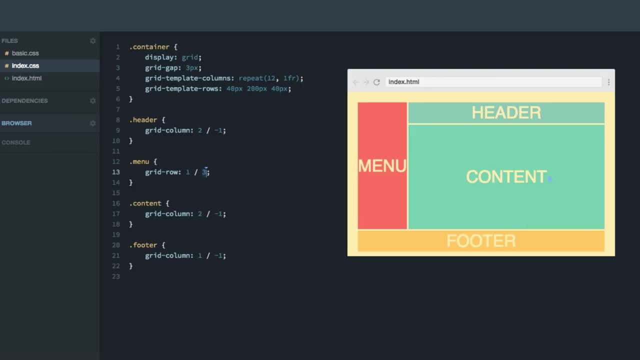 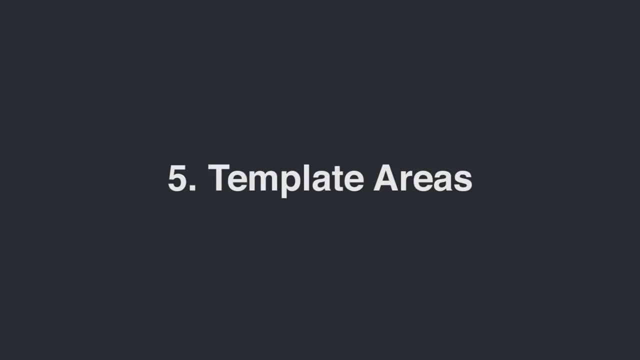 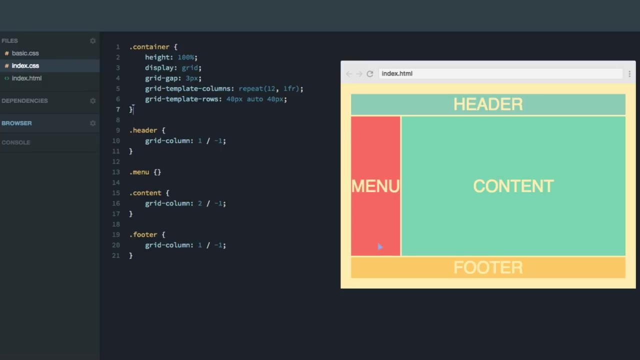 layouts, which gives you a lot of flexibility in terms of shuffling around on the content and experimenting. So stay tuned and I'll see you there. Hey, in this screen cast you're going to learn really cool feature of CSS grid called template areas, which allows you to change an experiment with layouts much more. 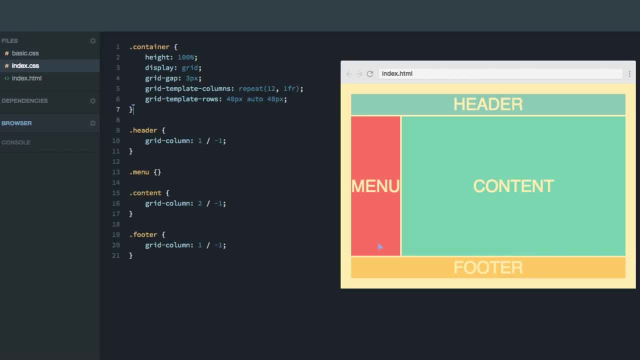 easily than with the techniques you learned in the previous cost. This feature is ideally ideal for creating prototypes of layouts quickly. We're using more or less the same example from the previous screencast. Our grid has 12 columns and three rows. The columns are just as they were in 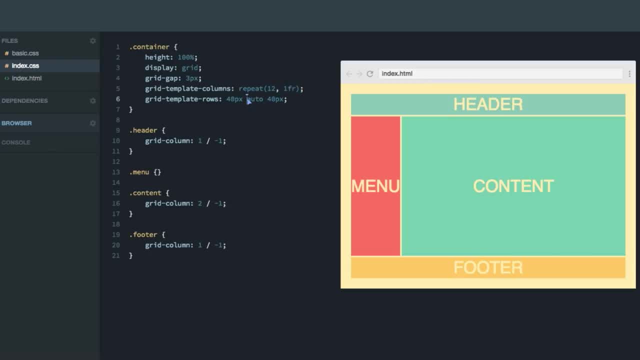 the previous screencast. However, for the rows, I've changed the second one from 200 pixels to auto. That means it'll take up whatever available space there is left in the height and combining that with setting the height of the grid container itself to 100%. 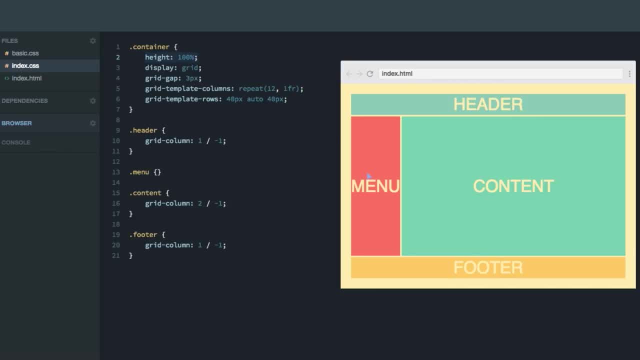 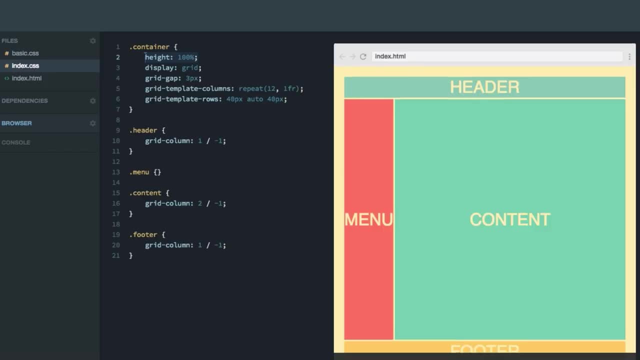 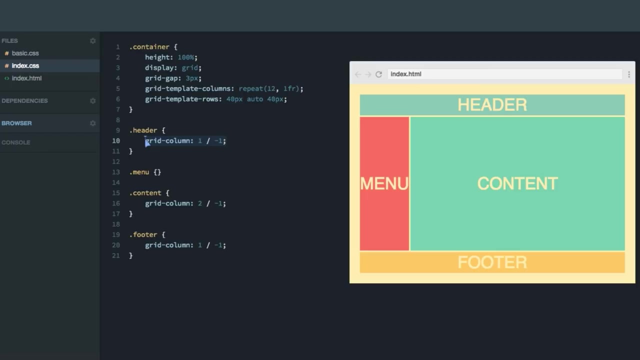 This will result in the grid being responsive in the height as well. As you can see, if we make it taller, the second row grows with the grid. Now we're still using the grid column property to adjust the position and size of the items. 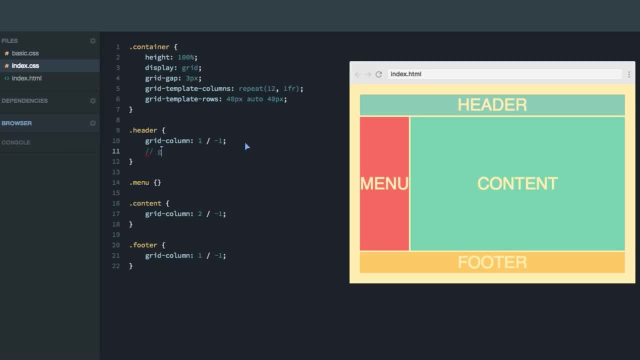 What we rather want to do in this screencast is use something called grid area, And to be able to do that, we're going to have to give the container a grid template areas property, And the syntax you're about to see now might seem a bit weird. It'll be a visual representation of 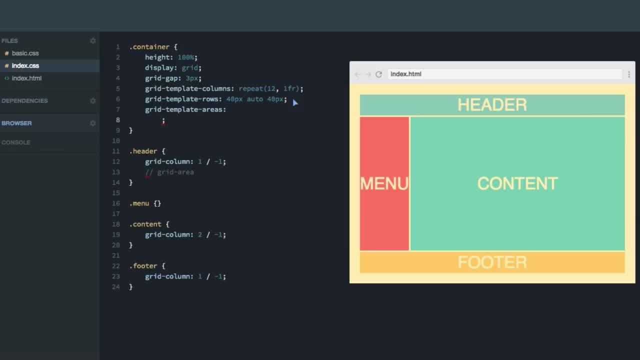 the grid And the way it works is that will create a string for each of the rows And in those strings we'll create a cell for each of the columns. So let's add the letter age 12 times in the first string. We have to give it exactly 12 characters. that has to match the amount of columns. 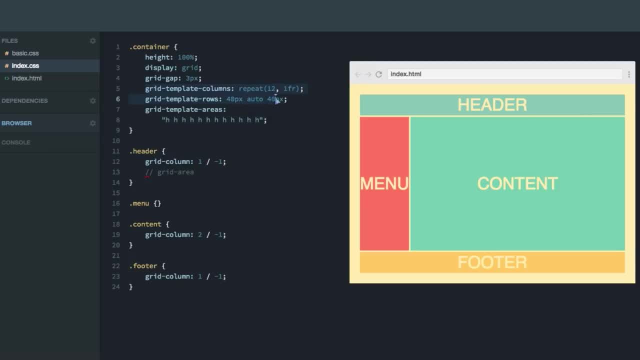 So we're not actually defining the columns or roles here. We've already done that up here. We're just naming them so that we can refer them using these names later on. In the second row we'll add one M and 11 seats and in the third row, Lynn, 12 Fs. What you have here is a visual representation of 200 statues. 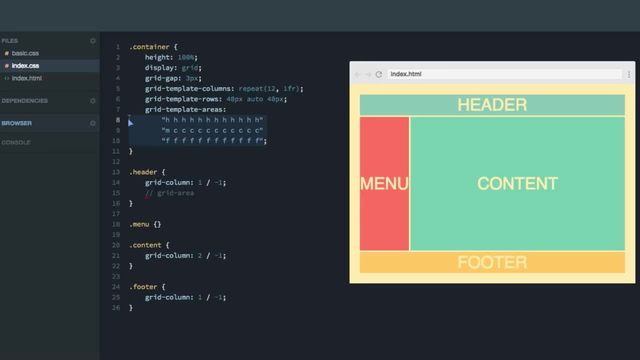 Here, now we can focus on our. So if we did, our Was words and addition representation of how we want our grid to look like And, as you might have understood, the age M, C and F refer to header, menu content and footer. So now let's remove the old way of. 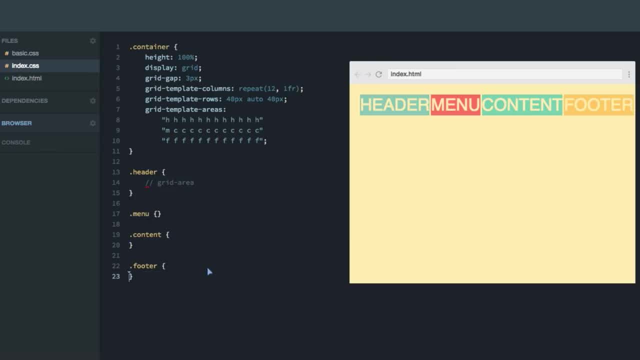 positioning the items like that and build up the grid over again. We'll give the header a grid area of age, As you can see. as a result, the header takes up the entire top row, just as we've defined here. We'll give the menu a grid area of M content: grid area. 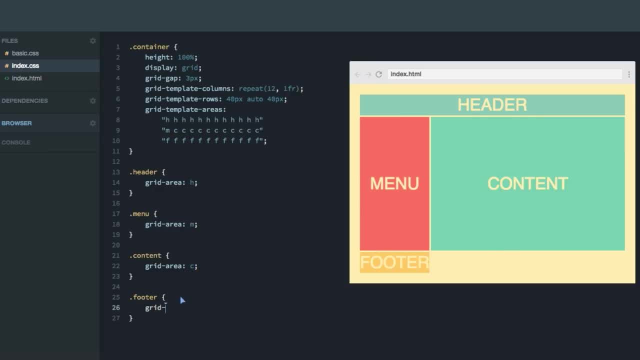 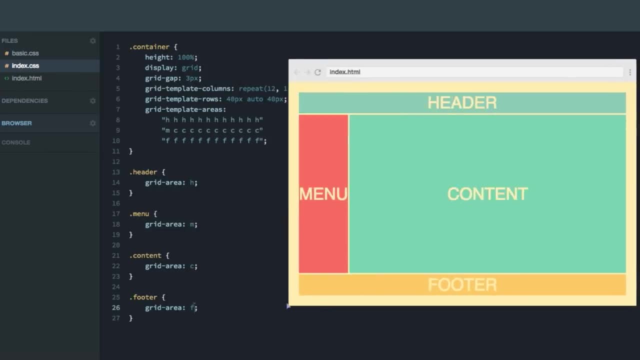 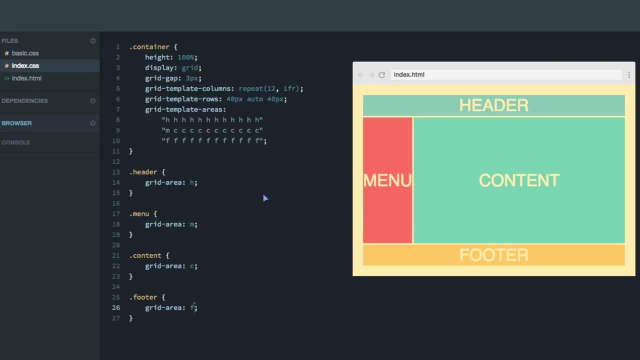 C, footer, grid. area of F. As you can see, our layout is just the way we want it to be, And it's responsive. Now, the reason this technique is brilliant for creating mockups is because now we want to make the menu span all the way to the top. 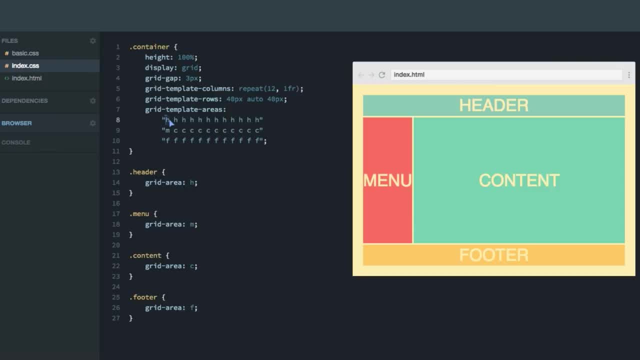 like we did in the previous screencast, We can just replace this age here with an M And, as you can see, automatically the menu popped up to the top. If you want to make it span all the way to the bottom, let's do the same thing here as well, And just as easy as that. 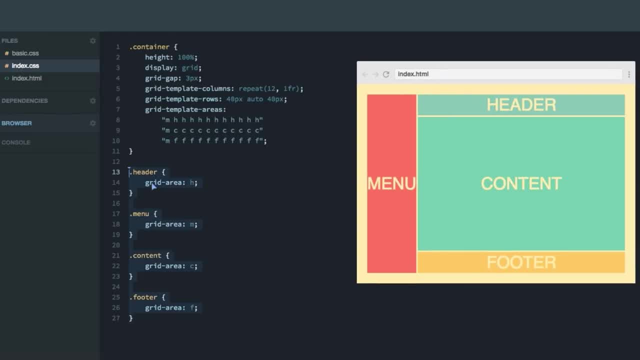 we have changed layout without having to fiddle around with the values in the item classes. You can also use dots, which will result in blank cells like that. There, there and there, And now we have this weird experimental layout where all the corners 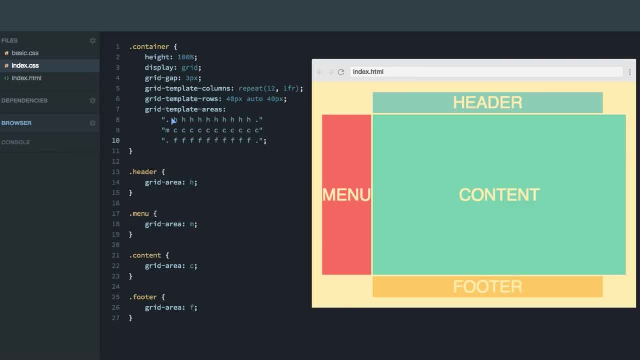 are blank. Now, one thing you need to be aware of is that the areas will only be valid if they are rectangle. Try and change this to an F so that the F footer goes like that. then, up you can see, it breaks the entire layout. So you have to use rectangles, As you understand. 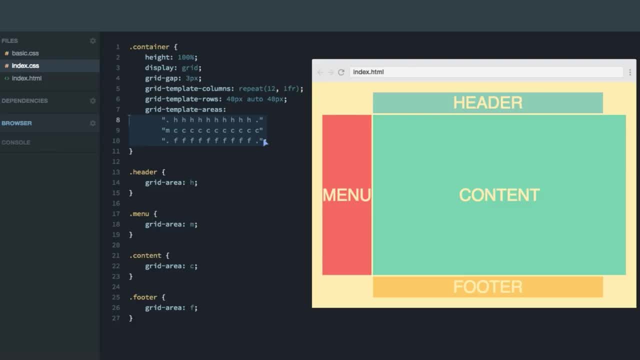 this is a super simple way of experimenting with the layout, So I'd recommend you to play around with these values here so that you make sure that you properly understand it, And once you've done that, you have finished the first section of this course. So congratulations, you now know quite a. 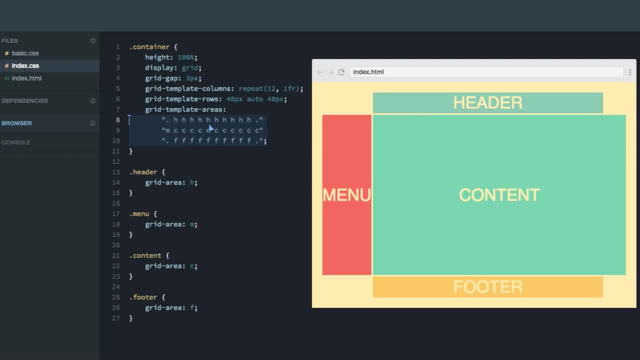 lot about CSS grid. However, there's still a lot of stuff to learn. So in the next section, I'm going to teach you how to create a CSS grid And I'm going to show you how to create a CSS grid- some more advanced stuff- And we're going to create even more responsive grids. That'll be. 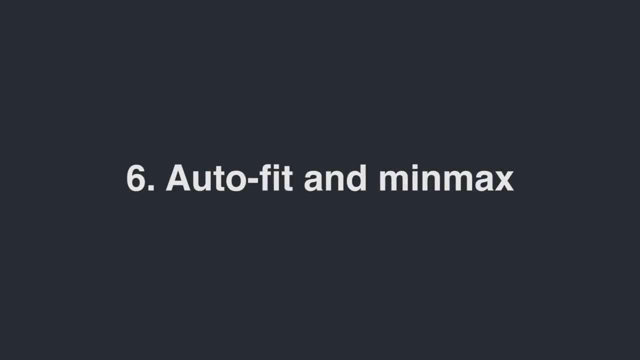 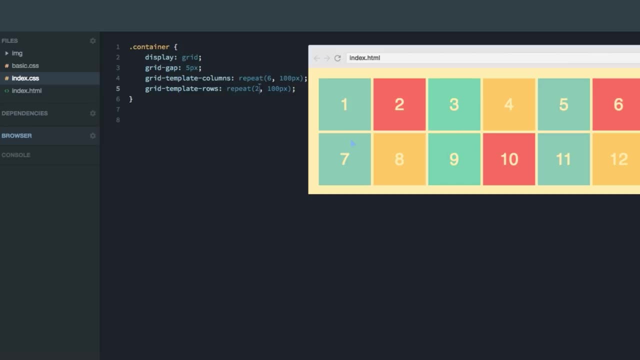 super cool, So I'll see you there. Hey, and welcome to the second section in this CSS grid course. In it, you're going to learn more advanced concepts. You've already learned about responsiveness, But now we're going to take that to a new level. So here we have the setup for a grid, which you can see in the browser window. 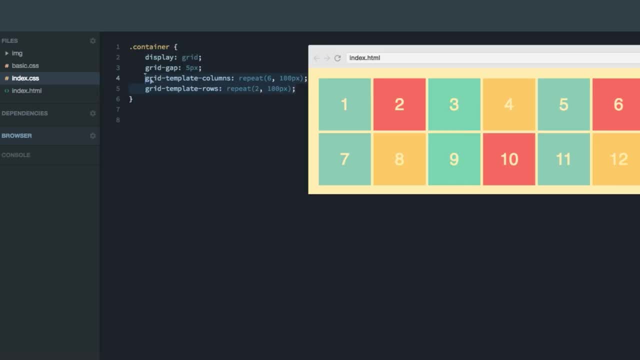 it's got six columns and two rows And that's defined here and should be pretty basic to you by now. both the columns and rows have a value of 100 pixels in width and height. So this grid is not responsive now, as you can see, but we know from previous costs that we can turn it into. 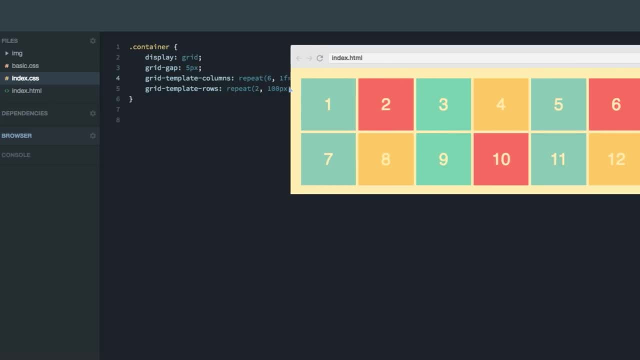 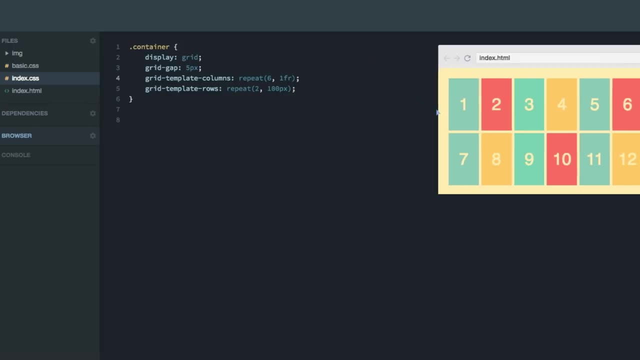 responsive grid by doing one fr instead. Now the columns will grow and shrink with the width of the container. However, you wouldn't necessarily always want your columns to be six like now. they're very squeezed together And at this point they're suddenly very wide. What you 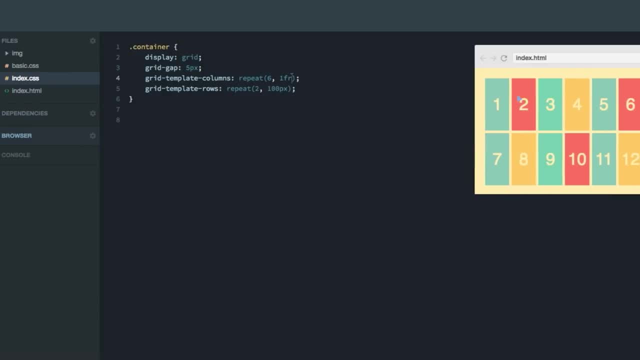 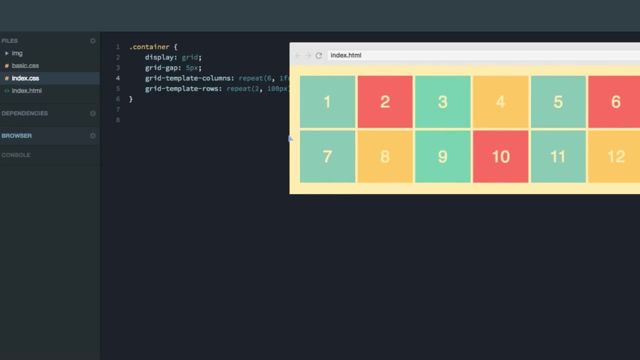 perhaps rather want to do is, for example, only have two in width when the example is being viewed on a mobile and six in width when it's viewed on a normal screen. So let's make the amount of columns vary with the width of the container. We'll first go back to having 100 pixels here instead, And 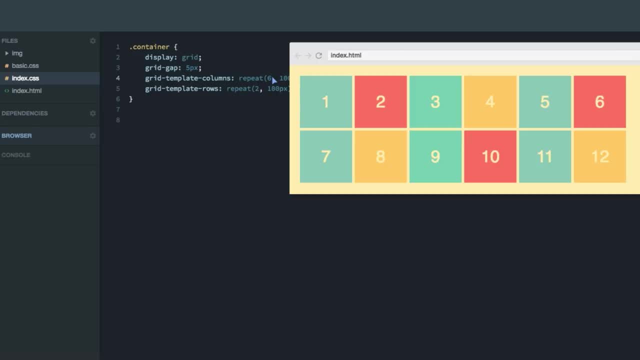 then, rather than hard coding in six columns, we're going to use something called auto fit. Now what will happen is that it'll vary the amount of columns with the width of the grid. As you can see, it simply tries to fit as many columns as possible into the container, And when it gets 100, 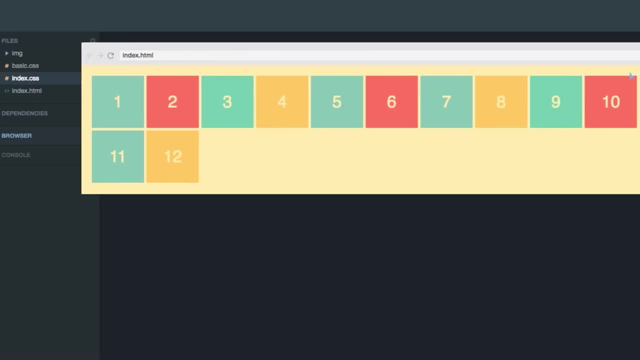 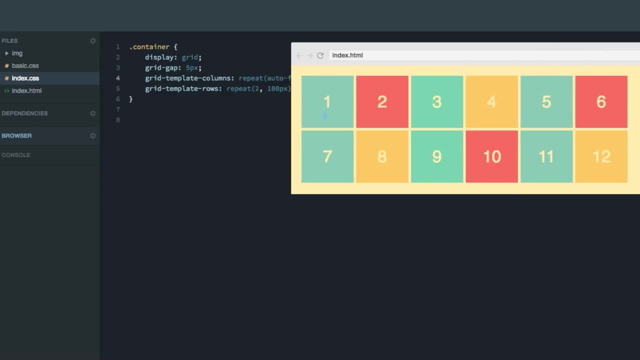 pixels extra space on the right hand side, it'll boom, add a new one. So on a very narrow screen it'll only show a couple of columns. However, this doesn't give us the responsiveness we want, as the amount of 100 pixel columns rarely add up exactly to the width of the container. Then we get 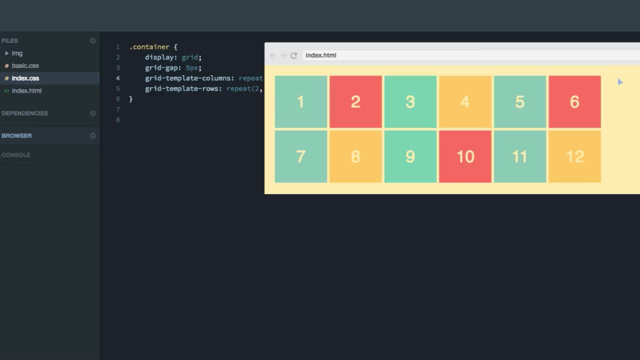 here, where we have quite a lot of space left on the right hand side, though, not enough to add a new column. that doesn't look nice. Now. you might think that we could rather do auto fit one fr. However, that'll only give us one column, because auto fit tries to fill up the grid with as many. 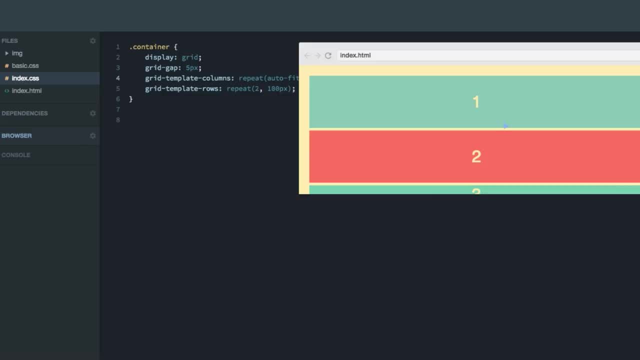 columns as possible until there's not enough space to add a new column. So when you use fraction unit, it starts by adding one column. However, then all the width is used up immediately, because at that point both the width of the entire container and the first 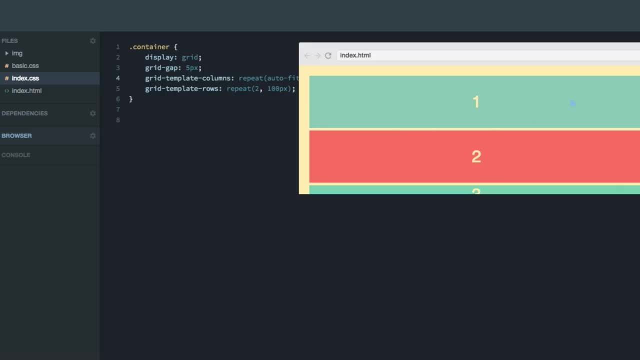 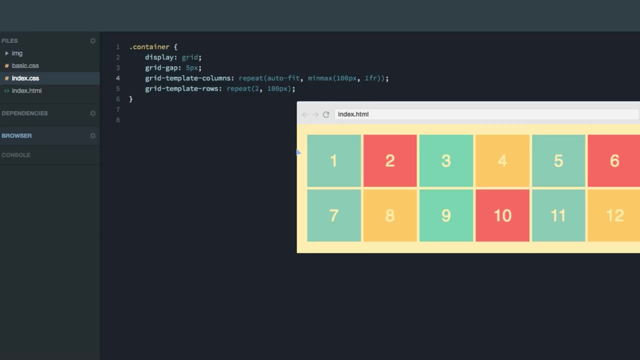 column are set to one fraction unit. So to get the behavior we want, we're going to use something called min max And we'll set our columns to be: minimum: 100 pixels, Maximum one fraction unit. Now you'll see that the columns will always fit the entire grid, regardless of whether or not the 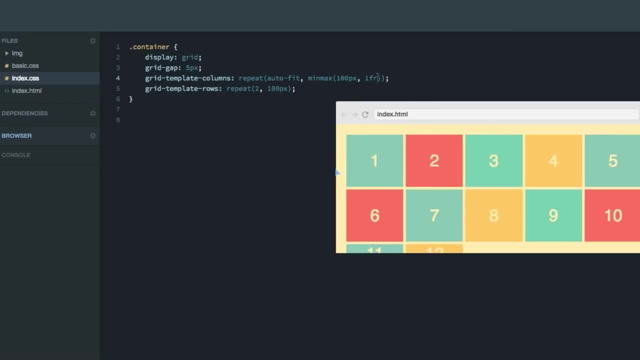 container exactly adds up to 100 pixels. Now you'll see that the columns will always fit the entire grid, regardless of whether or not the container exactly adds up to 100 pixels. Now you'll see that the columns will always fit the entire grid, regardless of whether or not the container exactly adds up to 100 pixels. 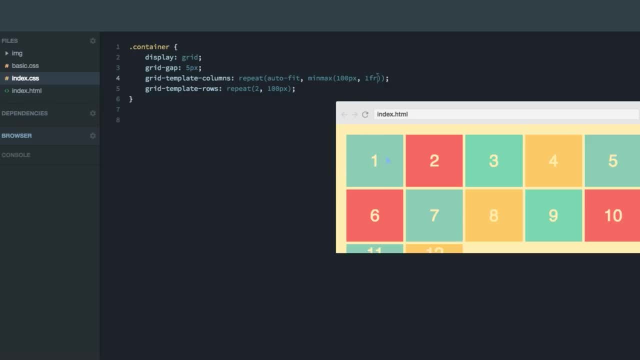 So what happens here is that the columns will always be at least 100 pixels, But if there's more available space, it'll simply distribute that equally across all the columns. So now they are more or less 100 pixels. If we make the page a little bit wider, you can see that. 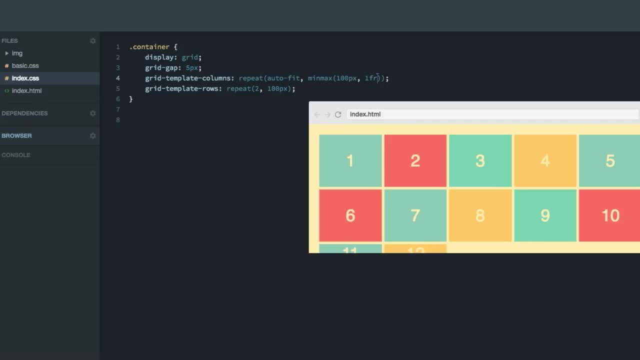 it stretches all of the columns. So now the width of the container is something like 550 pixels or something. However, when it reaches 600 pixels there, it uses the minimum size for the columns so that it can fit in six columns. So it prefers to use the minimum. However, when it doesn't add up, 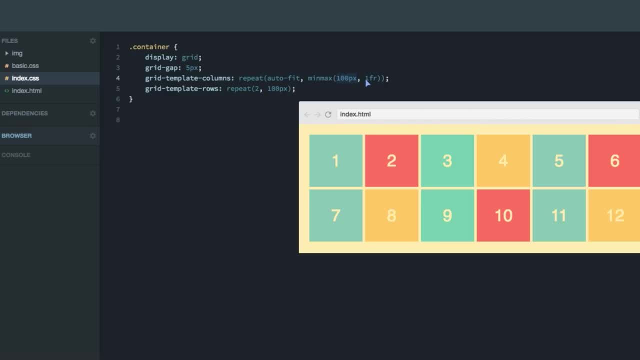 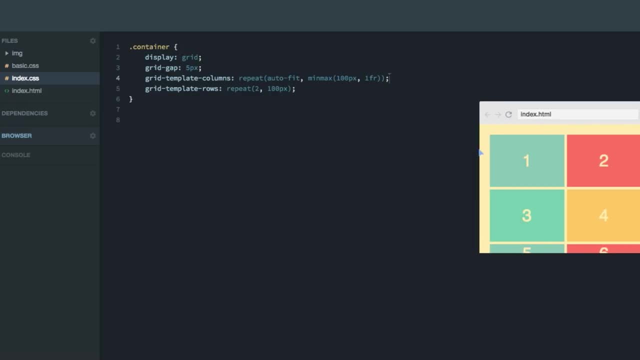 to exactly 500 or 600 pixels. it uses one fraction unit instead. So now we also get a nice view on mobile like that, and a nice view on a very wide screen. Okay, so in the next screencast I'm going to tell you about implicit rows, So stay tuned and I'll see you there. 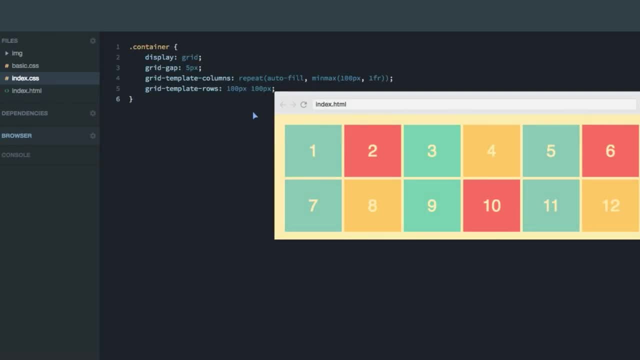 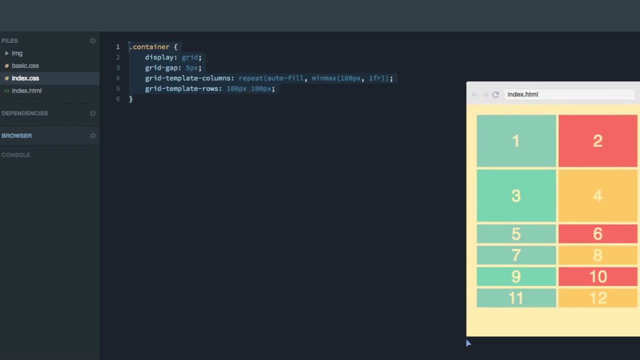 Hey, in this screencast we're going to continue with the grid from the previous one, as it still has an issue we need to fix, Because if we make this grid narrow like this and have a look at the rows that are created beneath the two rows we defined, we'll see that 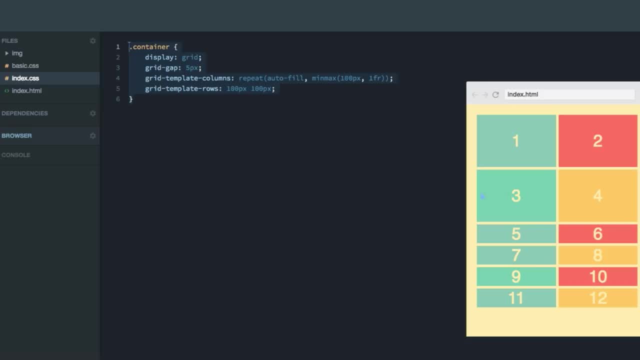 they're not acting the way we want them to. They're not 100 pixels in height, which we defined here. they're only as tall as the content inside of them force them to be, And that's because the rows are implicitly created, Because, as you can see here, we only explicitly created two rows. 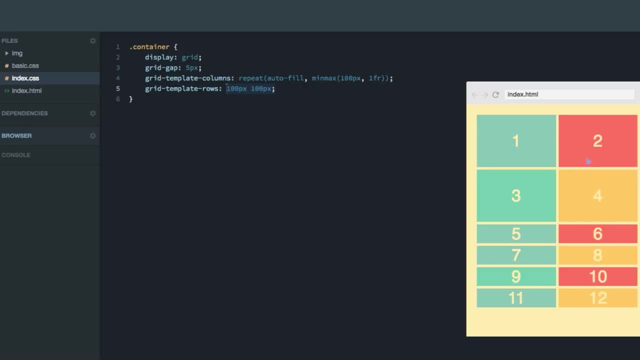 However, with our current defined behavior for the columns, we are going to need somewhere to place these items, which can't fit in our explicit grid up here. So, from five onwards, we need to create new rows automatically in order to display our items And, as we haven't told our 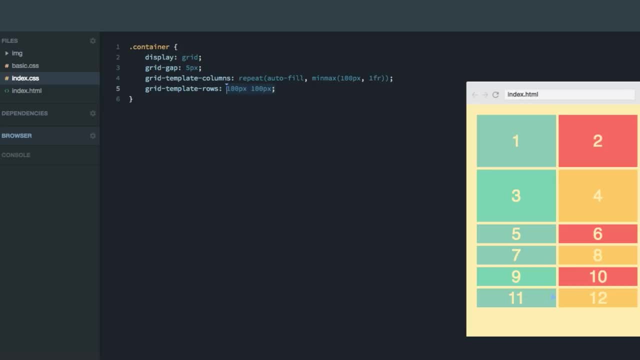 grid how we want to style those that it has to add to the grid itself. it just has to decide for itself how these rows are going to look. So let's fix this, Because we can target these rows by simply doing grid auto rows and set the value to 100 pixels. Now, as you can see, 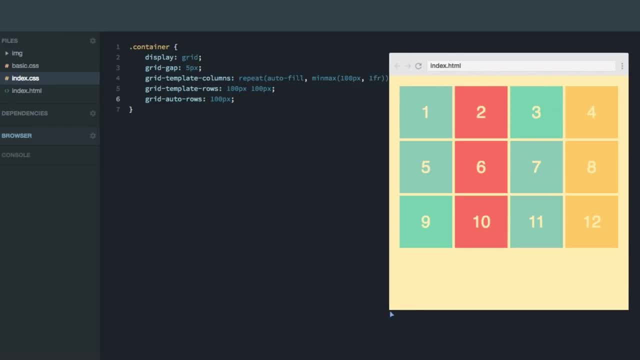 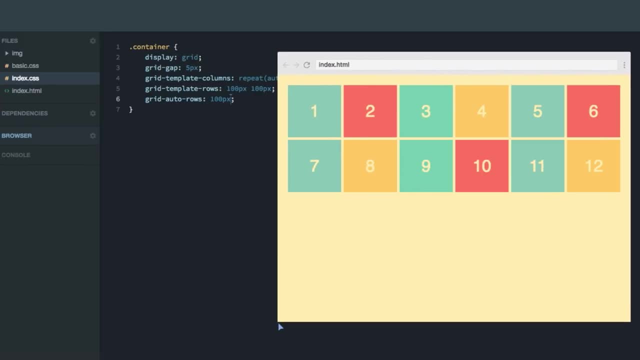 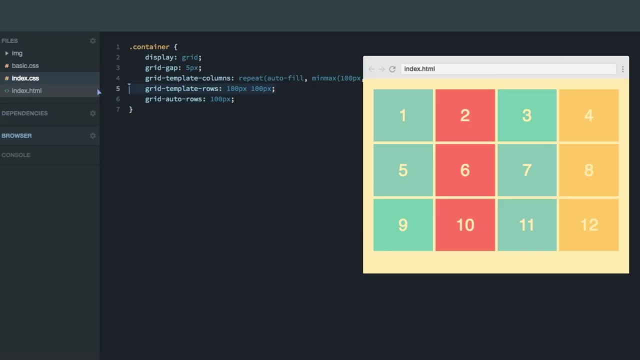 they're just how we want them to be. You can see that as well grows and shrinks nicely, with all rows always being 100 pixels tall, And now that we've defined this one, we can actually get rid of this one like that Now. 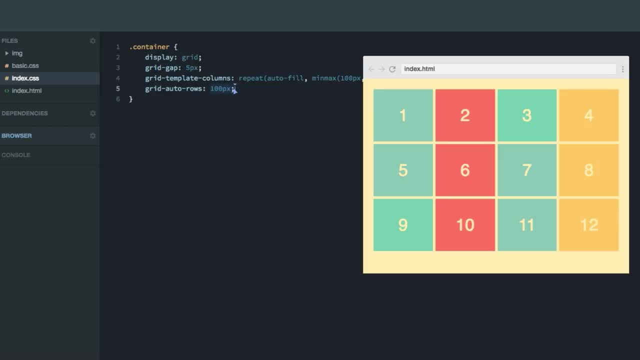 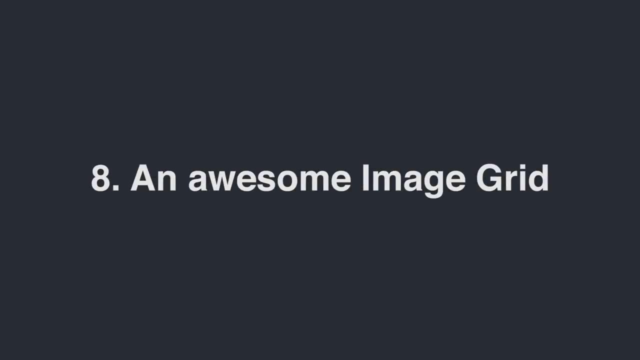 all rows will be created implicitly and they'll always be 100 pixels tall. So in the next screen cost, we're going to tie all the concepts you've learned up until now together and create a super cool image grid. So I'm looking forward to see you there. Hey, and welcome to the. 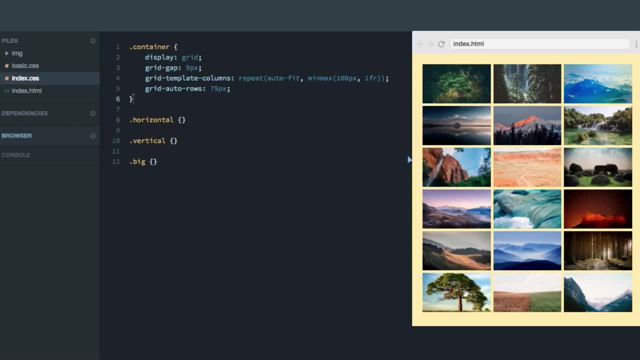 final screencast of the second section. Here we're going to take what you've learned up until now and use it to create really cool image grid. I've already created the setup. we're using the technique for responsiveness, which we talked about previously, using auto fit in combination. 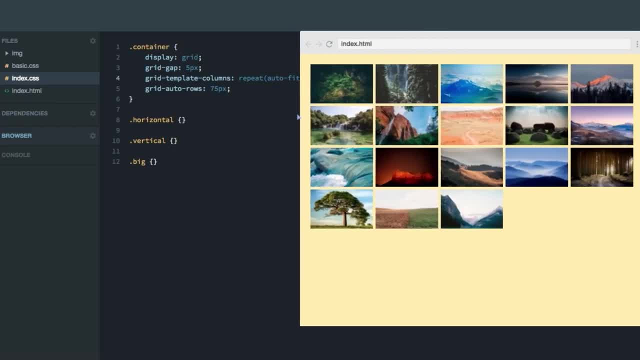 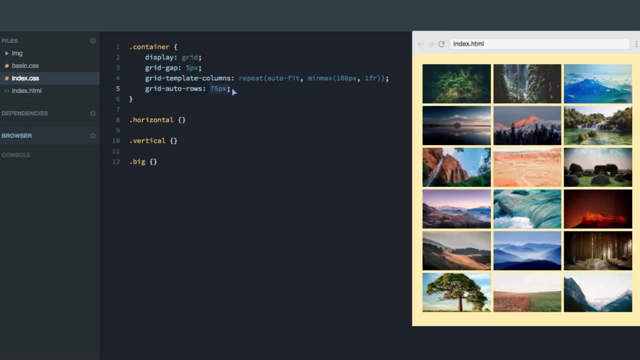 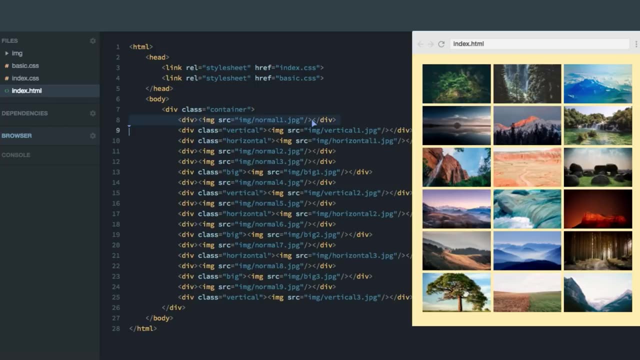 with min max, which gives us a nice responsive grid that varies. the amount of columns And the rows are implicitly created and are 75 pixels tall. In the index dot HTML you can see added an image to each of the items in the grid. That's, of course, the images you can see here. 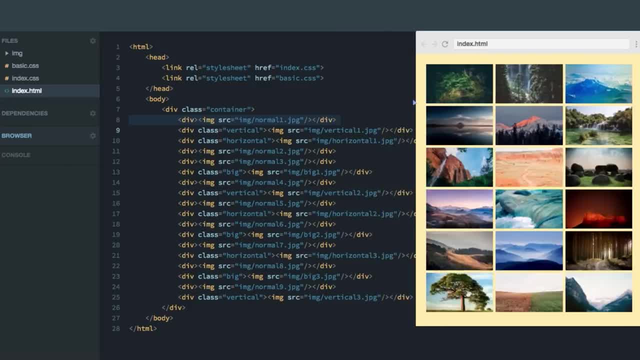 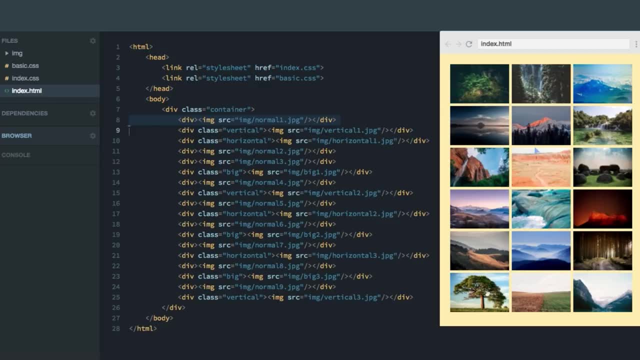 And this is already, I'd say, a pretty cool grid. However, not all of these images fit the frame they're given equally well. some of them might be more horizontal, while other images might be more vertical. I also have a few favorites which I think deserve a little bit of extra attention. 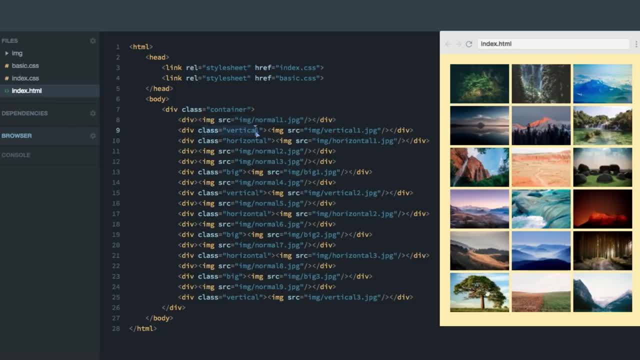 And you can see that I've actually given some of these item classes like vertical, horizontal and big. These are the images which I don't think fit well into only one grid cell. So let's go ahead and make the horizontal images twice as wide. We'll head over to the CSS, to the horizontal. 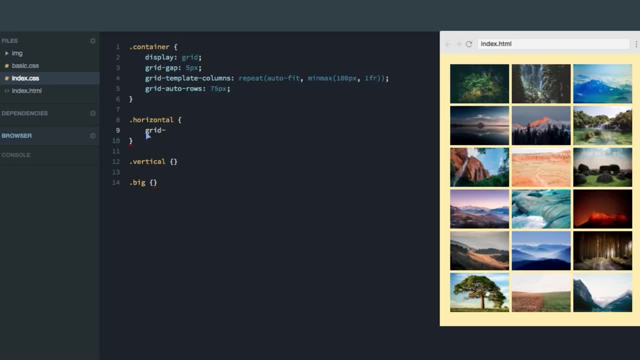 class And we'll set the grid column property. Now, previously we do something like one, that's the starting value, And then, for example, to span two so that they'd span across two, And then, for example, to span two so that they'd span across two, And then, for example, 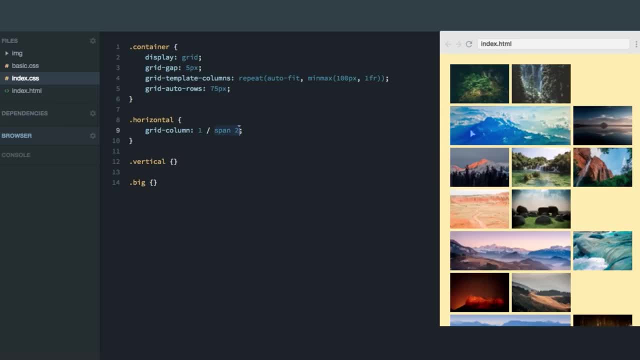 to span two so that they'd span across two columns. However, as you can see, that'll force all the horizontal images, which is this one, this one, for example, to start on the first column line. If we enlarge in the grid, you'll see that they'll that they'll still stick to the first grid. 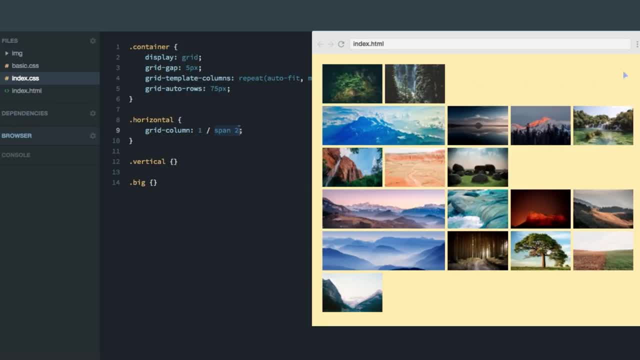 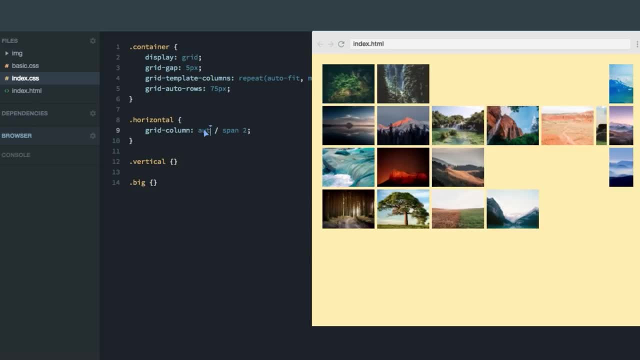 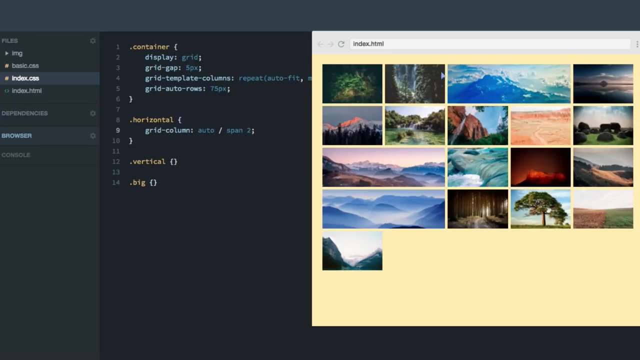 column line which, amongst other things, leaves open spaces in the grid, which is something we're going to talk about later on. So what we rather want to do is swap out this one here with auto. Now you can see, they start on whatever column line they were given initially. this one starts here And these two now happen to. 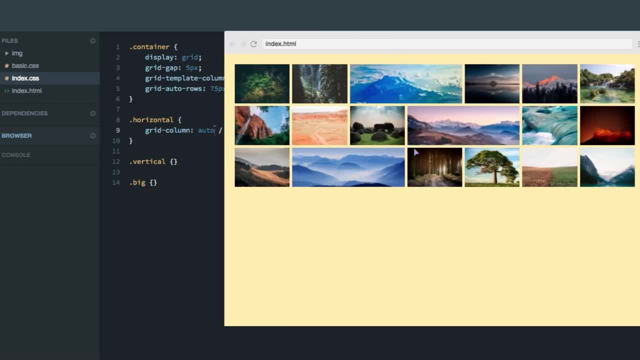 start on the first column line. But if we change the way that you can see that the horizontal images start on various grid lines and not just one, what we actually also can do here is remove this entirely. just do grid column span two, So the grid column and grid row properties can take. 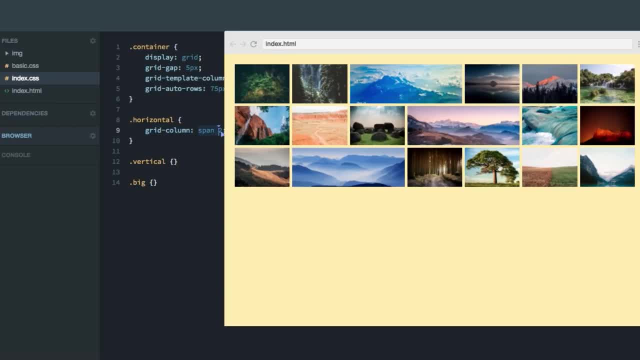 a lot of different values and combinations, And at this point, this is the simplest we can do. However, I wanted to show you the very various alternatives. Okay, now let's do the same thing with the vertical images, the ones we want to make taller than the rest of the images. So here we'll use grid row. 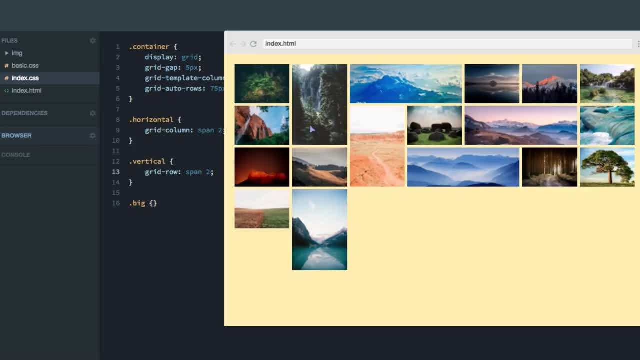 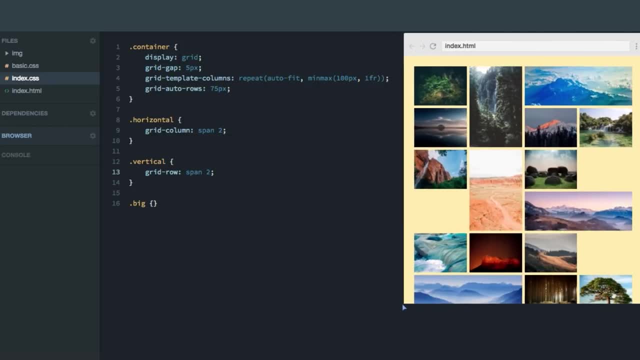 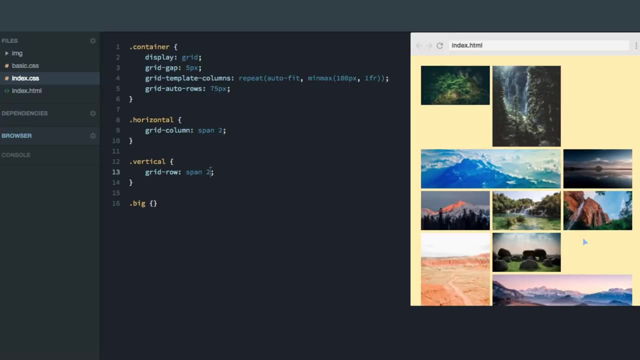 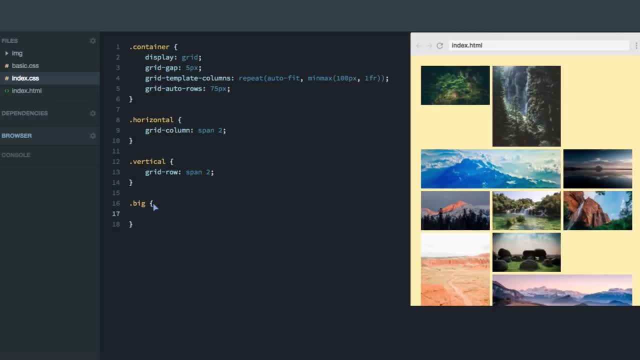 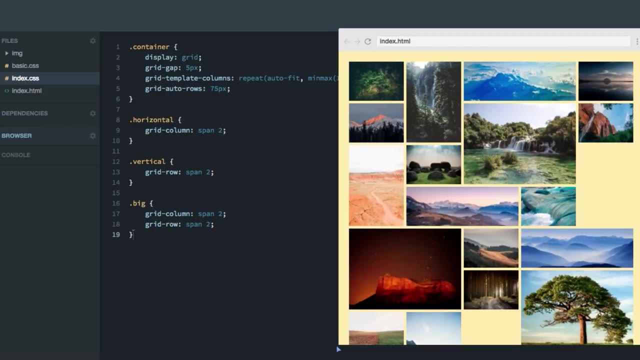 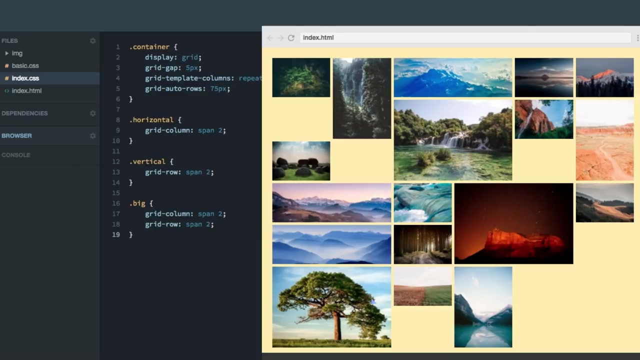 make the big images once we want to highlight: twice as tall and twice as wide as the normal images. grid column and two and grid row span two. Now you can see this image here, this one here and this one here are really getting the attention they deserve. 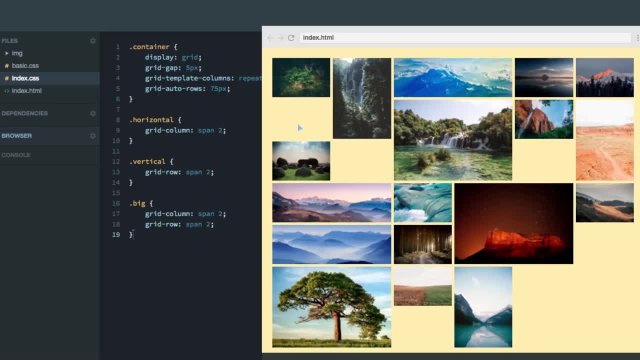 But we need to fix these blank spots here because that doesn't look nice. So why do these blank spots appear? To understand that, let's look at how the grid lays out. each of the items starts up here in the top left corner lays out the first item, the second, third. 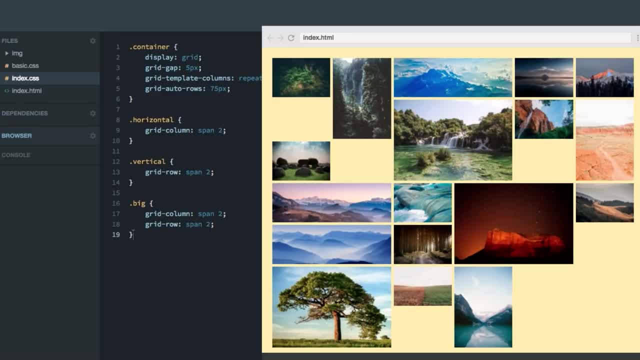 fourth, fifth and then it needs to continue on the next row, which is here, And it tries to fit in the sixth image. However, when it's about to lay out that one, it can't fit it, as it only has one grid cell available here. However, 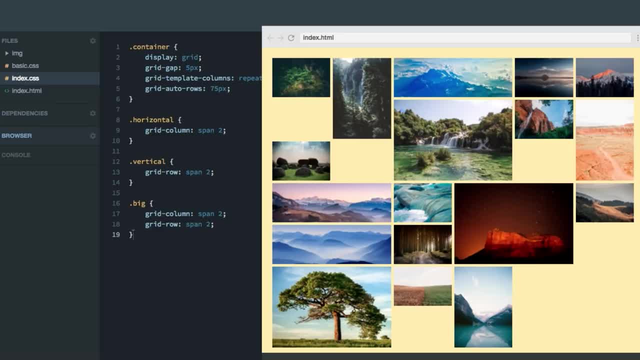 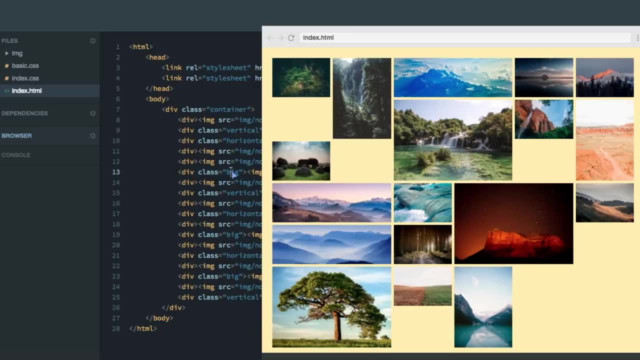 the sixth item is a big one. It's this one here. Let's double check that in the HTML, laying out the next item here here and then one here, leaving that spot here blank. Wouldn't it be great if we somehow could fill these spots? 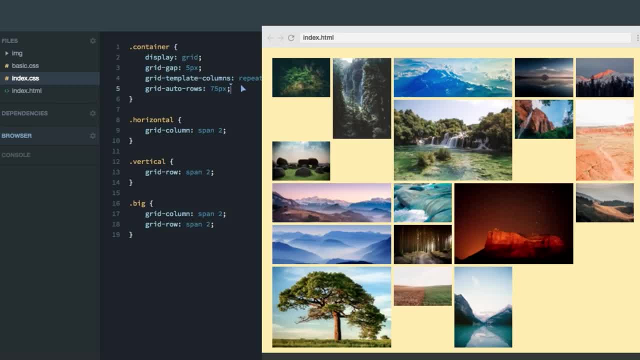 Well, we can, And to do that we're going to use a property called gridAutoFlow. It's, by default, set to row, meaning that it'll lay out the items one row at a time, just as we talked about starting here and going across the first row. 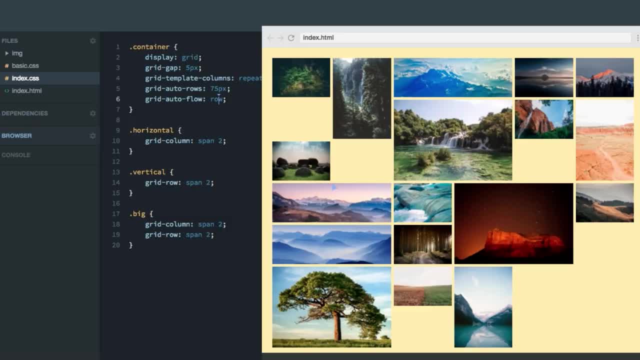 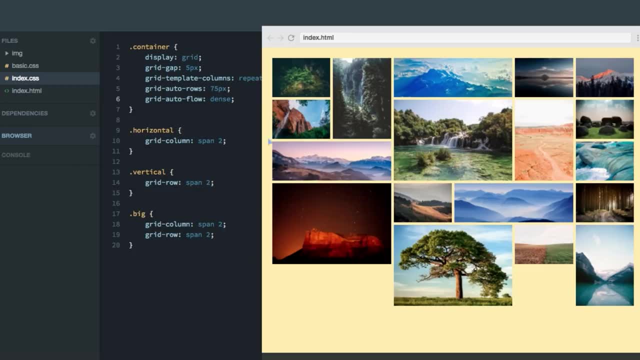 and then jumping next to the second row and continuing on like that. However, if we set it to dense, we'll use so-called dense packing algorithm, which attempts to fill the holes in the grid. If there are holes in the grid and smaller items come up later. 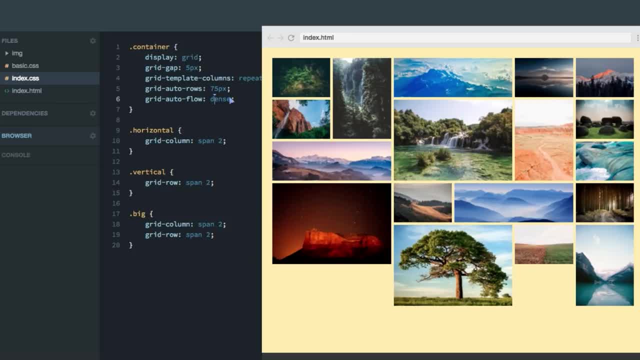 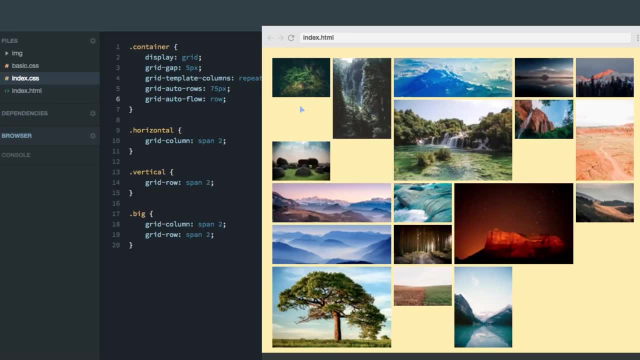 then it'll move those up to fill the blank spaces. So if we go back to row, we see that this space this blank, and the next item in the grid which could potentially fit in here would be not this one, the sixth item, but the seventh item of the waterfall here. 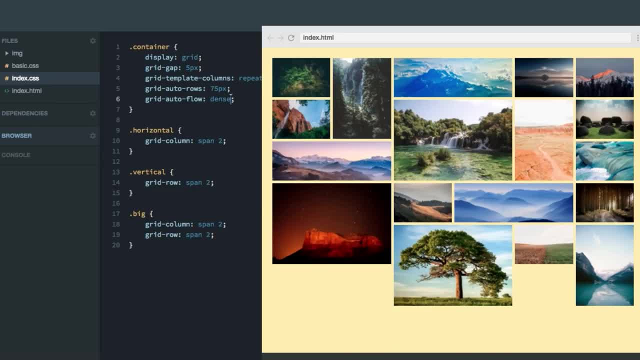 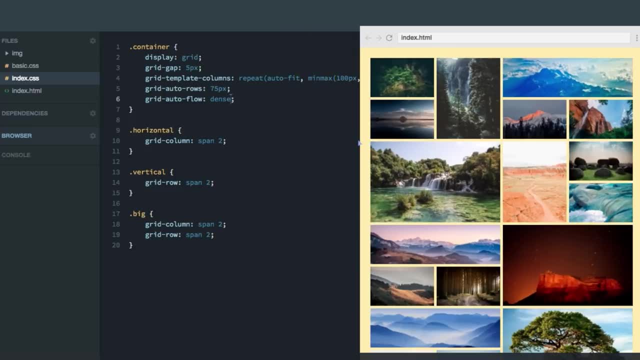 So let's look at what happens when you change it to dense, And indeed the waterfall image has now jumped back to this position and filled that hole, And this works regardless of how wide the screen is. As you can see, we have a super cool image grid now. 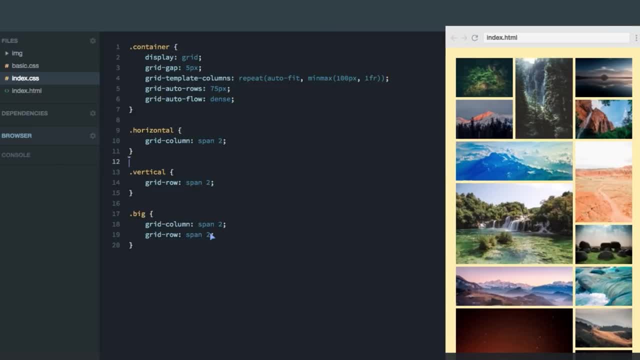 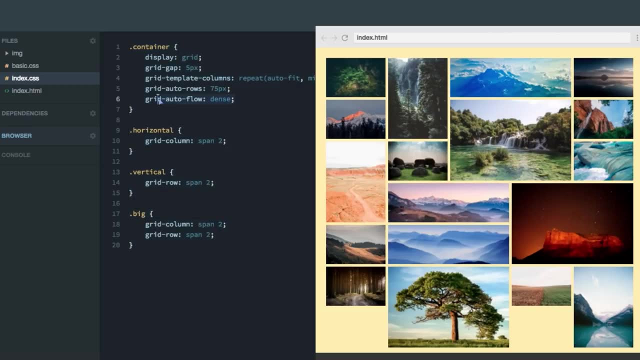 which looks really hard to create actually. However, we've done it Simply using these 20 lines of CSS. And finally, I want to mention that this dense feature here is an example of source order independence, which is a huge win for CSS. 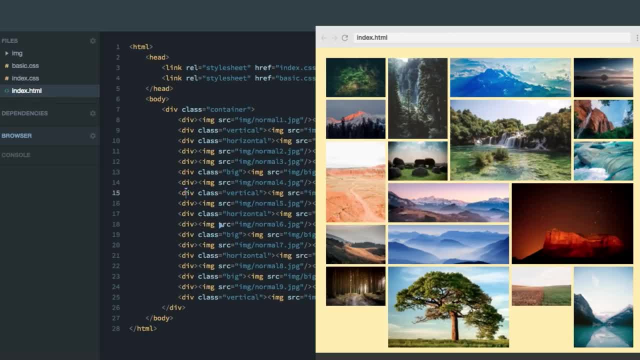 It means that the grid can arrange the items regardless of how they're laid out in the markup. Here, we simply use the markup for what it's supposed to be used for- markup for content- and we're using the CSS for what it's supposed to be used for: styling. 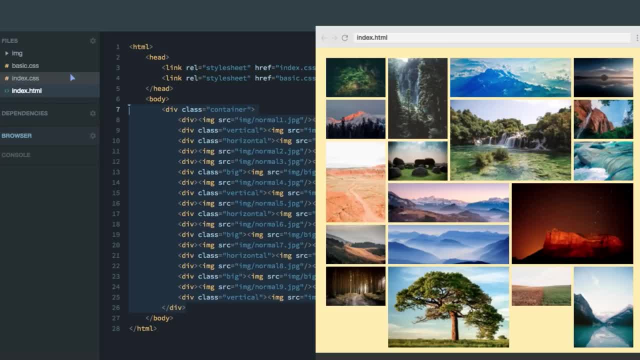 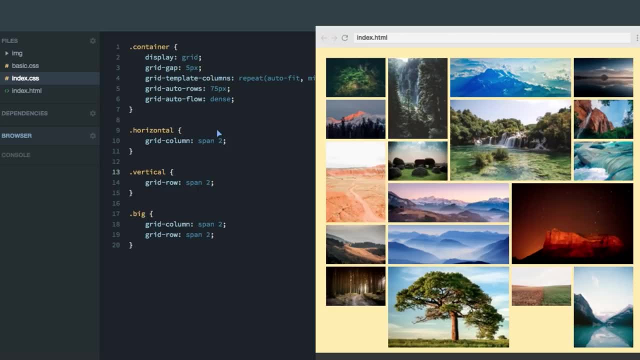 And we're not losing the markup. We're just limiting it to whatever order we laid out the images initially. So source order independence gives you a lot of flexibility. So this marks the end of this section. You now know quite a lot about building advanced CSS grid layouts. 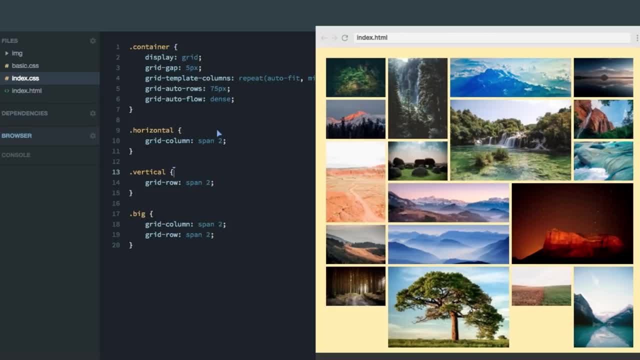 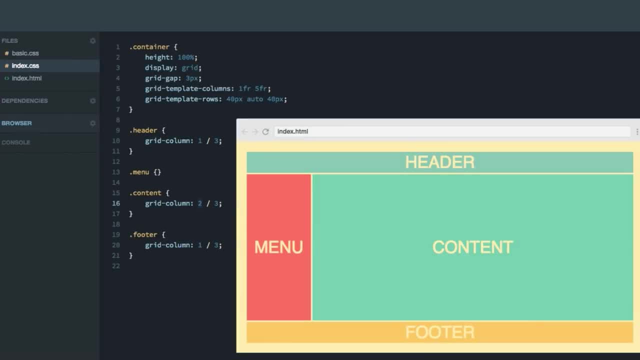 However, be sure to check out the bonus material if you're hungry to learn even more. Thank you, Hey. in this screencast, you're going to learn a new way of positioning and sizing the items on the grid using some of the Bill's tools. 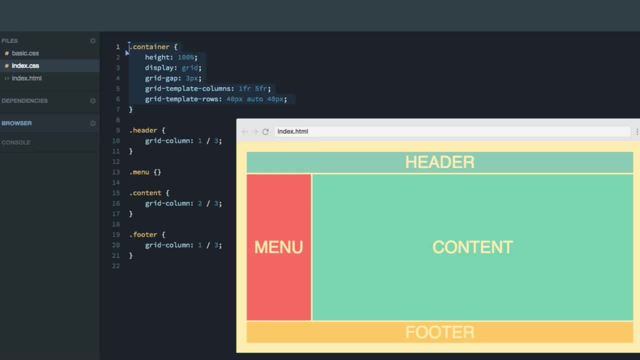 something called named lines. So we've defined our normal grid here, which is the website layout you should be familiar with by now, Though in this case we're defining it in the very simple way of only having two columns, one being one fraction unit and one being five fraction units. So we're 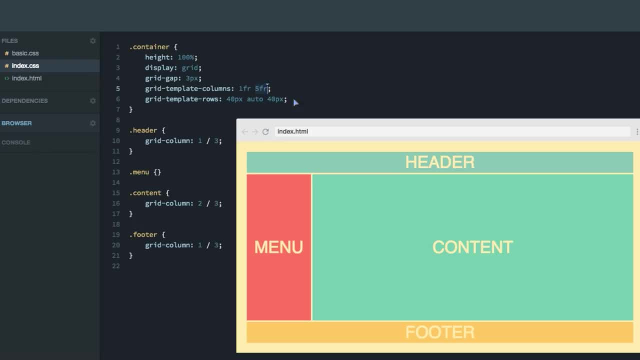 not using the flexible 12 column layout here, as this setup makes it easier when using named lines. So to brush up a little bit, the grid has column lines and row lines. The first column line is the one on the left hand side, The second one is one separating the two columns And the third one is 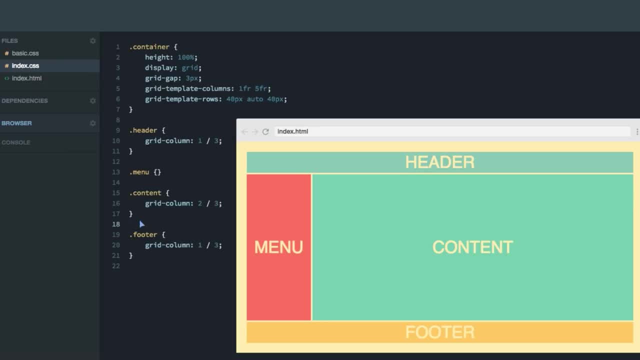 the one on the far right hand side, And our content item, for example, is defined to span from the second row line to the third row line, from here to here. In our code, that will be from the line that goes in between here and until the line that goes here. So what we now can do is we can add a. 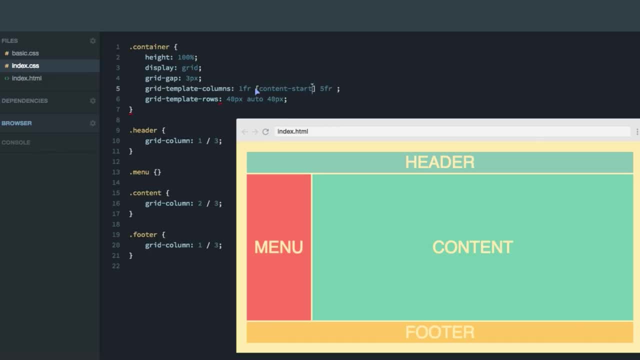 square bracket in between and write content. Start, for example, on the third line and write content And like that. Now what we can do is we can swap out the number two here with content start And the number three with content end. 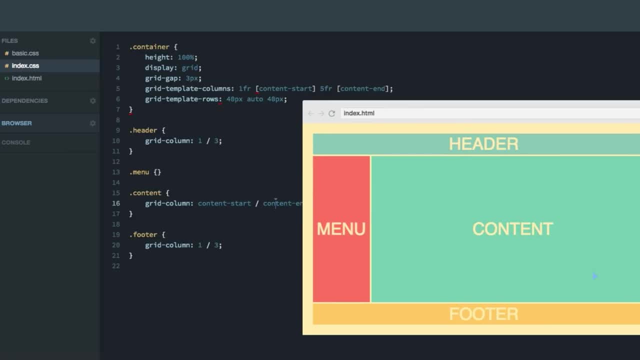 like that. As you can see, that works fine. If we wanted to do the same thing for the header, we'd have to give a name to the first line. Well, up here, let's call that main start. So now the header spans from main start to content end. 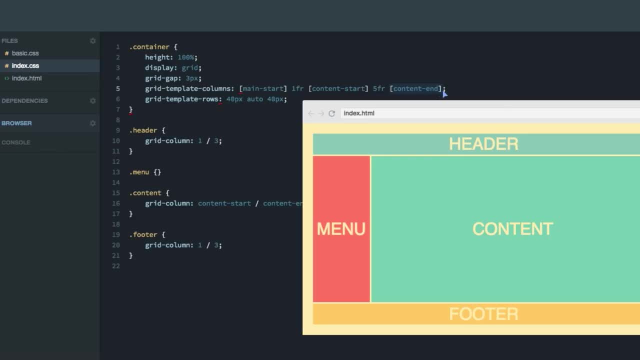 However, I actually want to call this line main end as well, because there might be a case in the future where we want to reference the main end explicitly, not use content end as a proxy for it. So So let's just add a new name here. 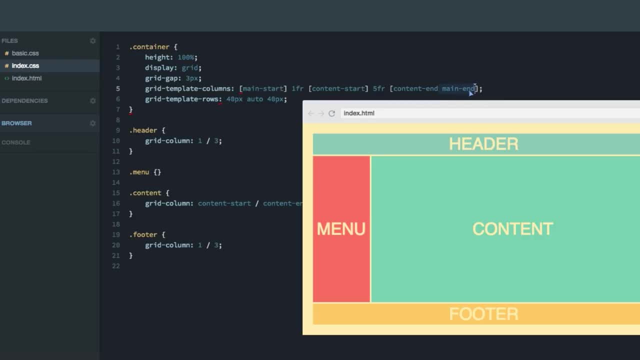 And like that, just give the space and then the new Name. Now we can do main art, main end. As you can see, works perfectly fine. The footer can get the exact same layout like that. Now let's also name the rows using the. 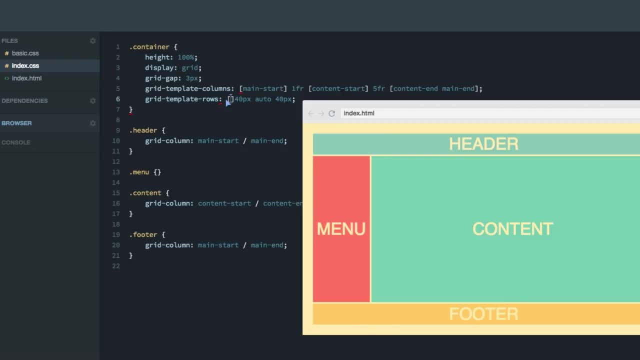 exact same convention. We'll do main start. I'm just going to copy them and then start And And main end like that. Now you might wonder why we've been using this dash syntax here, And that's because they give you a little bit of magic. 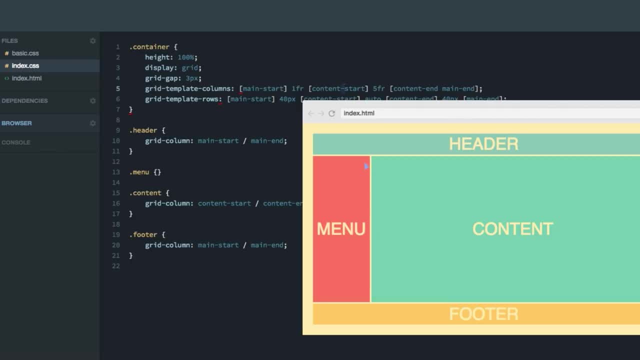 Now, given that we've called this line here for content start and this line here for content end, the grid knows that this is the content column or columns, if that was the case, so you can actually set the grid column to just content like that and, as you can see, it works. now the header and the 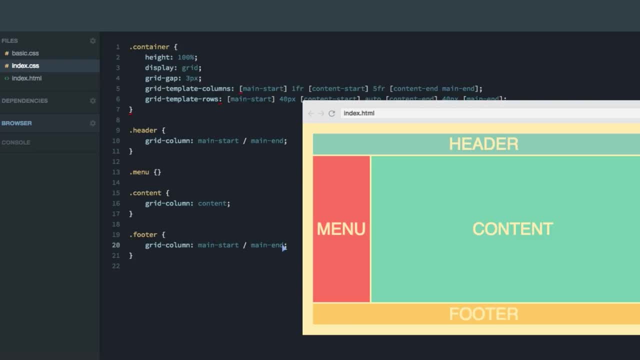 footer spans from main start to main end. so we can do the exact same thing there as well: just use grid column main. and to take this even a step further, actually we can also use grid area in one of these cases. that'll be in the content case, because let's have a look at the content lines. 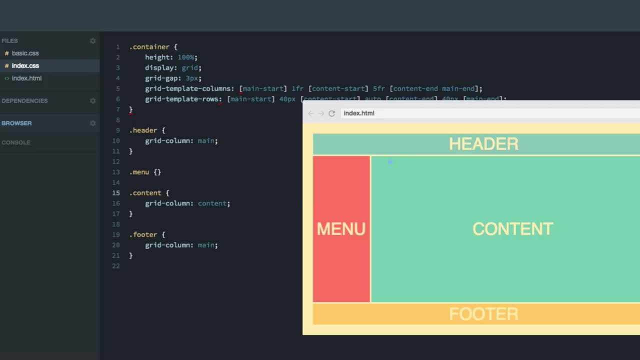 both the row lines and the column lines. so we know we have the content start here and the content end here, though we also have a content start here- the second row line, first, second. so this one here and this one and the second one, and we have the content start here and the content end here. 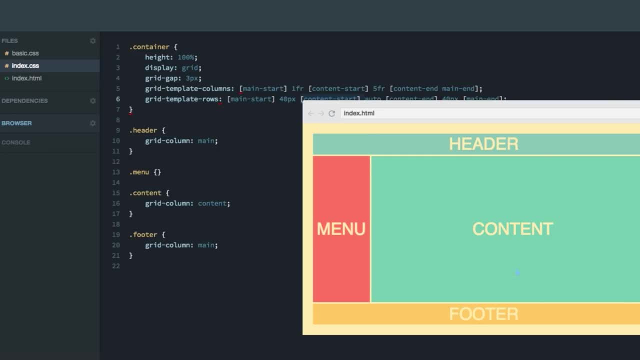 so let's check how the跟ya content lines are it? although we almost necessarily don't have to here, and we have a content end on the third row line, the third one here, meaning we have boxed in an area with content lines here, here, here, here and here. 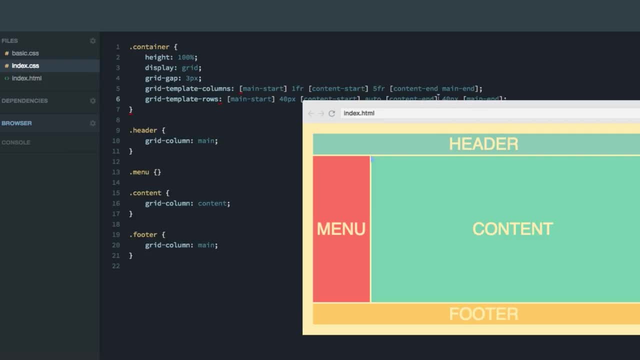 and now we can actually use grid area, which you might remember from section 1 of this course, by simply doing grid area and set it to content like that, and it still works. however, you might be tempted to try and do the same thing down on the footer. 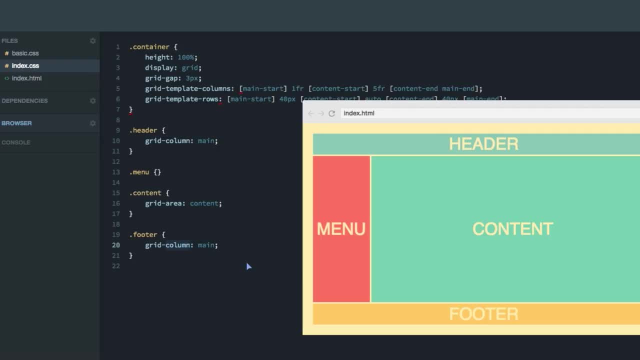 though that wouldn't work because it has to be boxed in by four main lines, though the main start row line is the one that starts up here, not down here above the footer. so here we have only kind of boxed it partially in. we have the main start column line here, which is 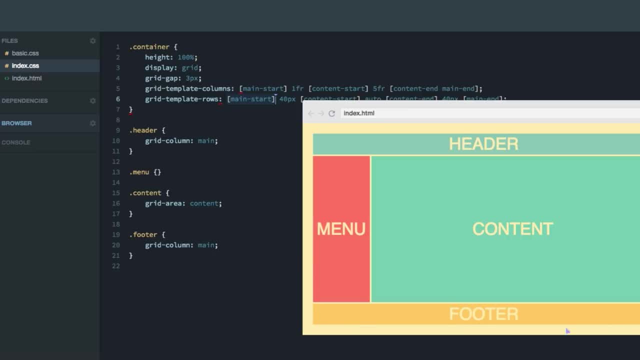 the start of the footer and the main end row line, which is the bottom of the footer, and the main end column line, which is the right hand side of the footer, though the top of the footer is the content end line, so we can't use grid area main here. as you can see, it breaks the entire. 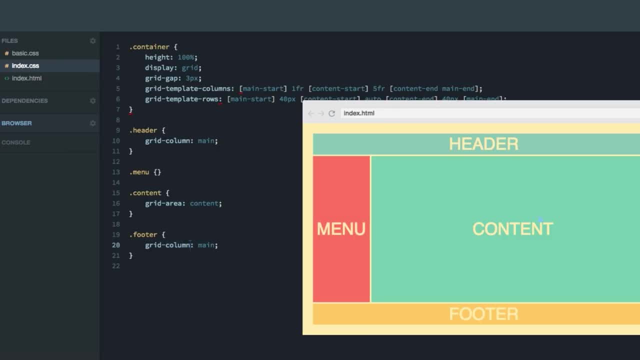 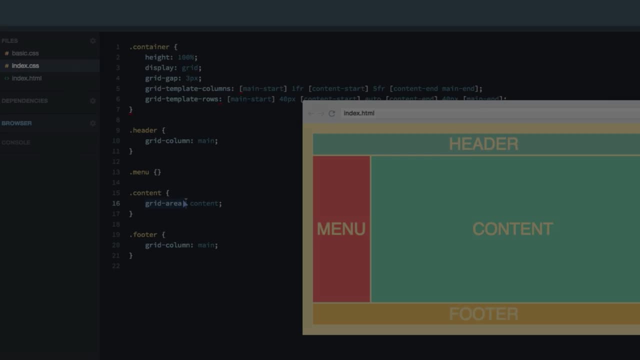 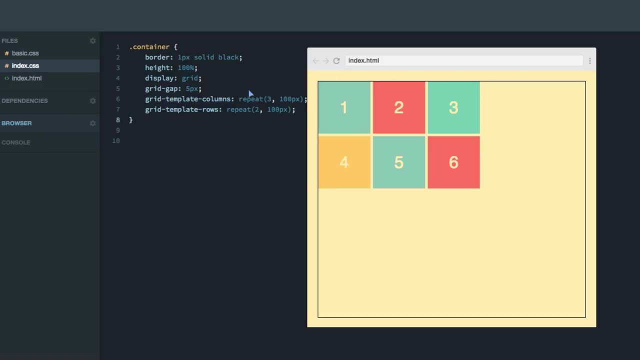 layout. so be careful and make sure that you have properly boxed in an area before you start using grid area. ok, that was it for this bonus screencast. thank you, hey. in this screencast I'm going to show you how to justify and align. 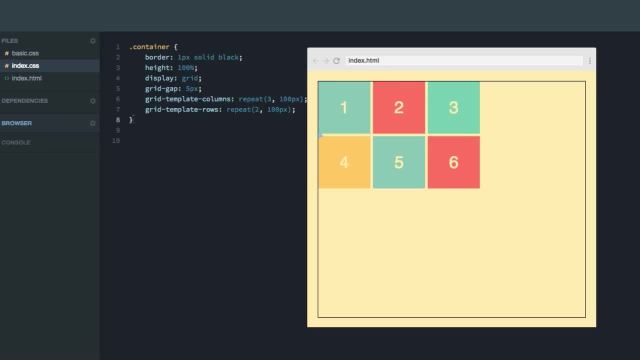 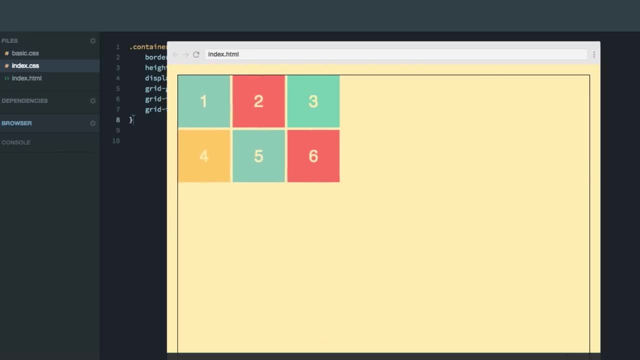 the entire content of a grid. I've added here a black border around the grid container so that we can see its edges. I've also made sure that the grid is fully responsive and that there's a little bit of space around it. so right now our grid items only occupy 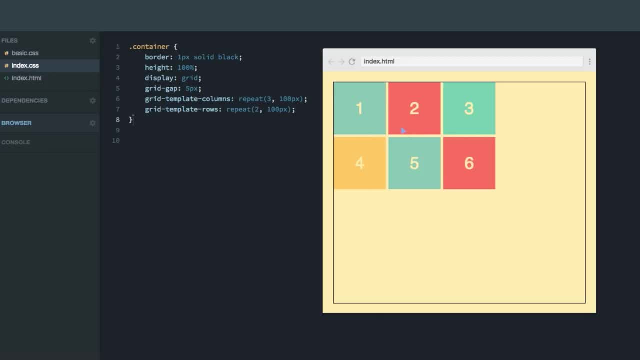 a tiny part of the entire grid container and that's important in order to learn about justifying and aligning the content. so let's start with the justification, which defines and distributes space between and around the items along the row axis from left to right. 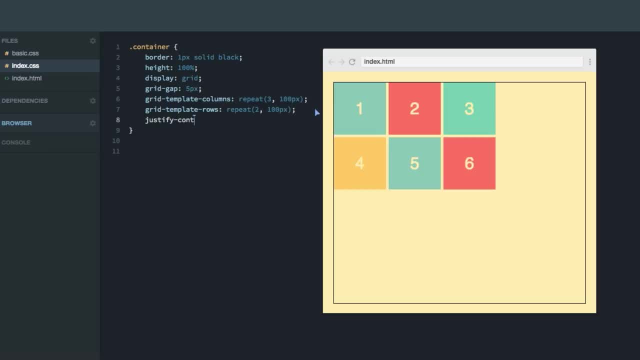 so if we set justify content and set that to end, as you can see, that'll shuffle all the content over to the right hand side, to the end of that axis, the row axis. the default value here was start. you can also do center like that. 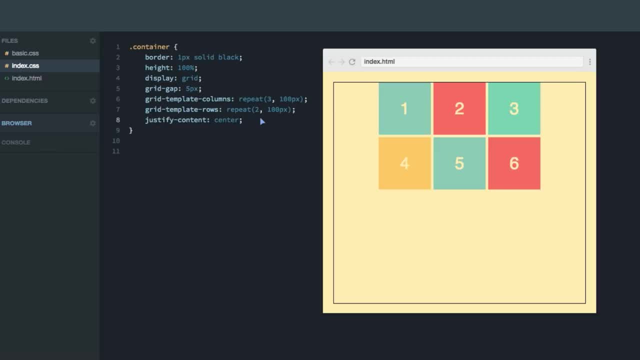 that'll center it along the row axis. so let's combine this with align content as well, and do end. for example, I'll push all the content down to the lower end of the grid, because aligning controls the content along the column axis, the vertical one, which goes from top to bottom. 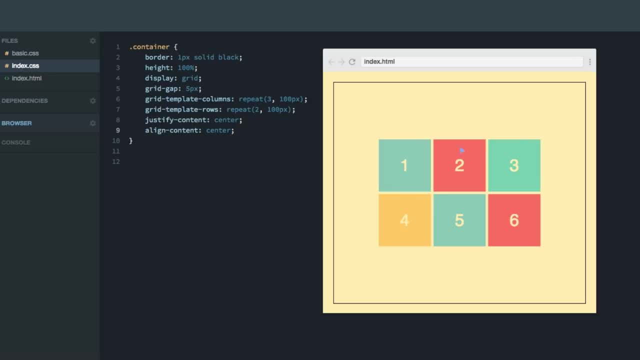 if we do center here as well, we'll fully center the items in the grid. now let's comment out this one and have a look at the other values you can use here, because there's a couple of cool ones if we, for example, want a lot. 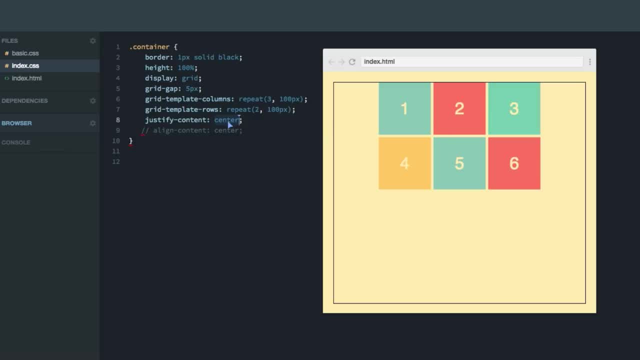 of space in between the items. we can do space between. now we have as much space as possible in between the items along the row axis. we can also do space evenly, like that which distributes the items evenly throughout the row axis, so the items have an equal amount of space around them. finally, there's also the space around this. 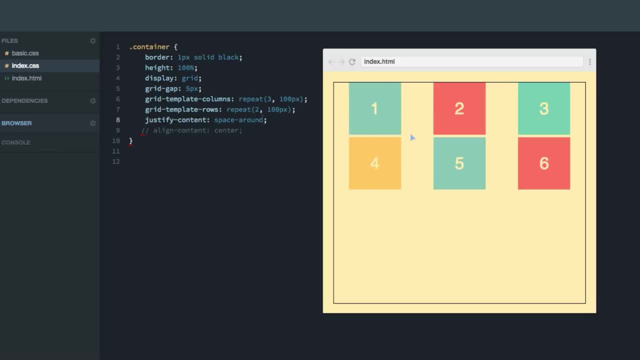 one is pretty similar to space. evenly, though, each of the items have a half size space on either end, meaning that if you have two items besides each other, that'll give a full size space between them, though here, in between the first column line and the first item, we only have a half space. 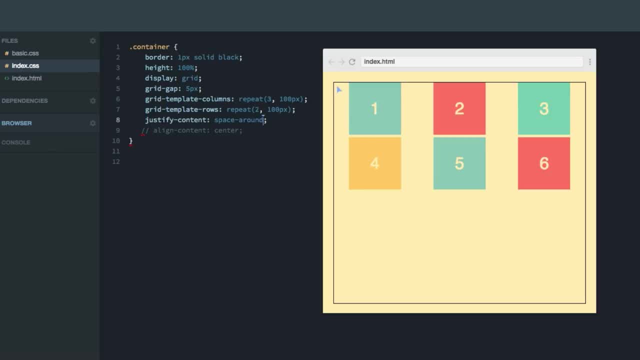 so we can do space evenly like that, so the items have an equal amount of space around them. as this item forces a half space on this side, though the grid line itself doesn't force the grid to create any space for it, though, in between these two, both of the items force the grid to add. 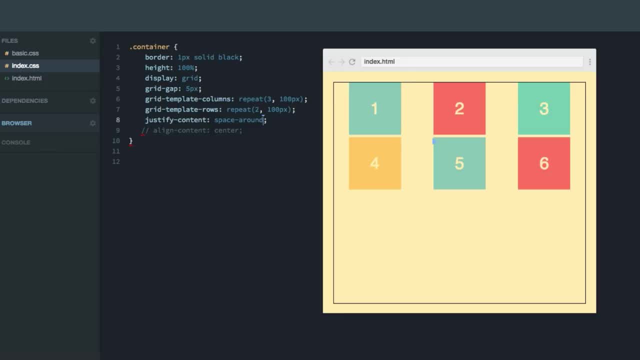 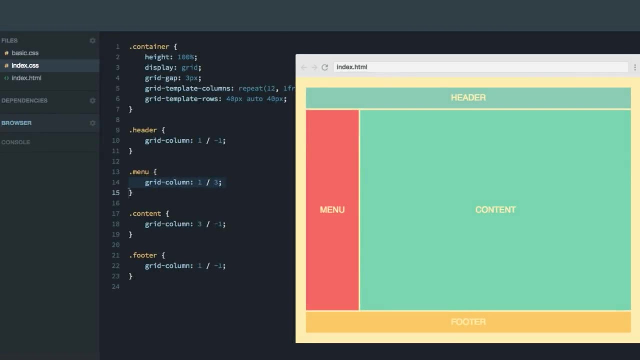 a half space in between them, resulting resulting in full size space. so that was the basics of justifying and aligning the content. thank you, hey. in this screencast, i'm going to show you how to create a grid line. i'll teach you how to justify and align the items on the grid. so here we have our classic website. 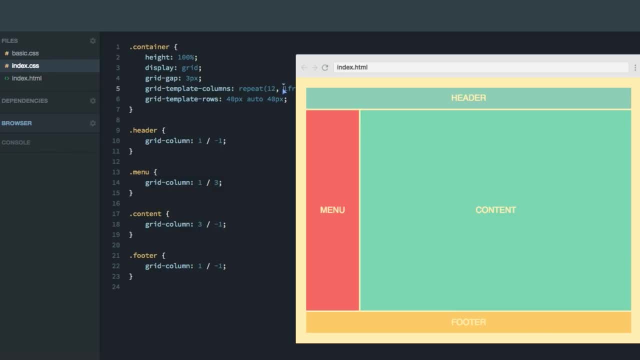 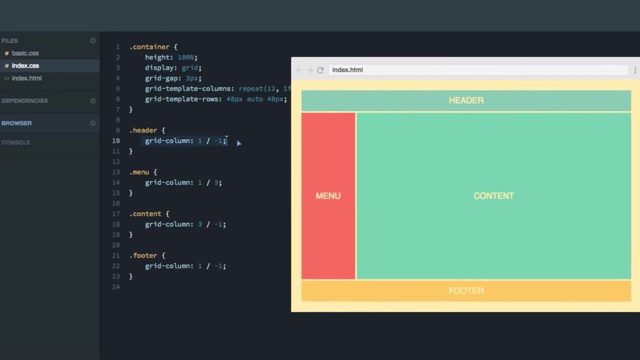 layout. it contains 12 columns in the width. each are one fraction unit and three rows, where the second one is auto. so this grid is responsive in both width and height. as you can see, we have defined the width of each of the items using the grid column value. so for the header, for example, 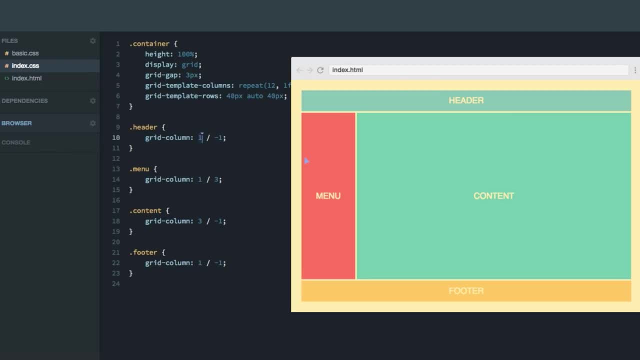 we're saying: start at the first column line, which is the first column line, and then we're going to this one and end at the last one, which is this one over on the right hand side. so it's kind of stretching from the start point to the end point and this axis, here, the row axis, is the one you. 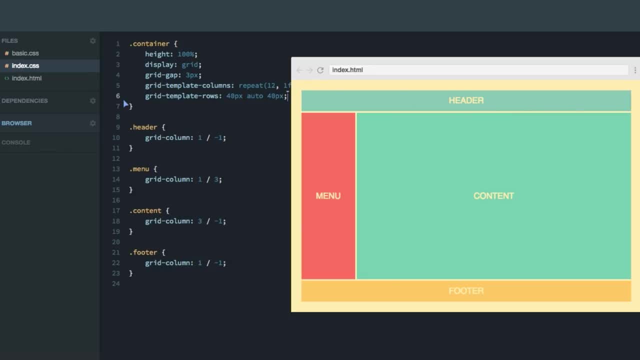 control with justification. so if we do, or if we do justify items, that'll be by default set to stretch. however, if we, for example, want each of the items to rather center itself as much as possible and not stretch the items, then we can do that by doing a little bit of a stretch here and then we can. 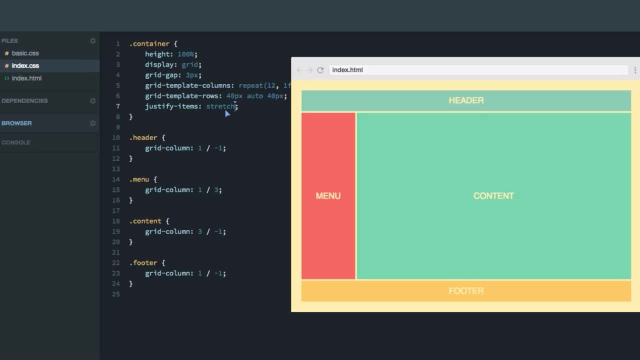 it all the way from the left-hand side to the right-hand side. we can use center And, as you can see now, each of the items are centered at as much as possible. You can also use start- That'll squeeze all of them towards the left-hand side, And end is the opposite of this, That'll squeeze. 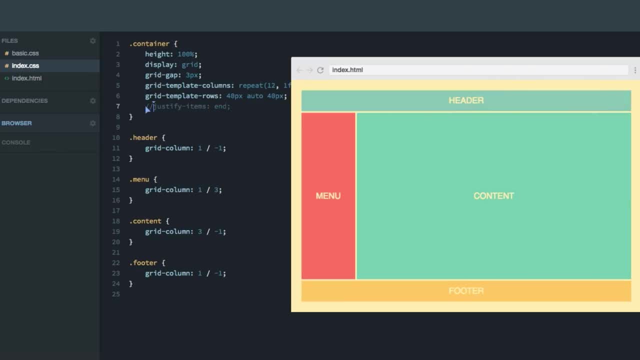 all the items to the right-hand side. Now let's comment out this a little bit and use the align items property. That'll do the same thing, though along the column axis, So the vertical axis, from top to bottom. So if we do center here, you can see that each of the items are now squeezed together. 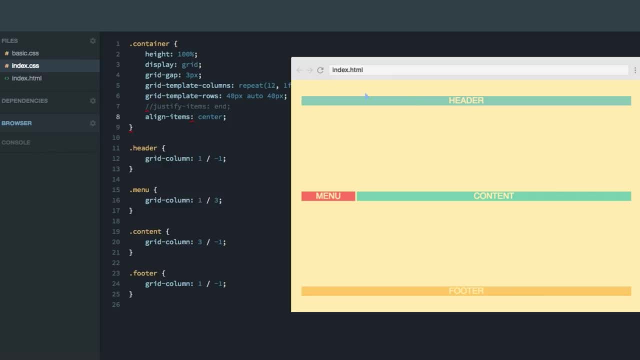 towards the center, though not on the left to right row axis, but on the top to bottom column axis. We can do end That'll squeeze all of them to the bottom, Or start That'll squeeze them towards the top. Now, 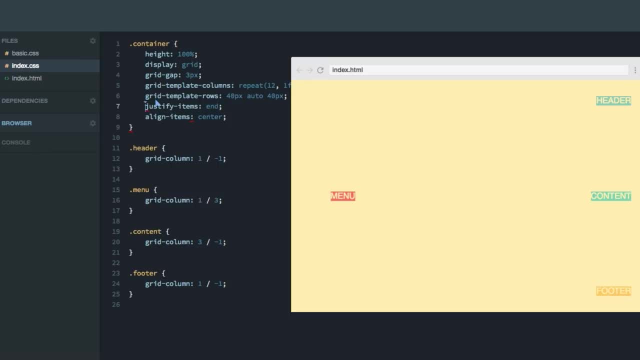 let's do center again and combine this with center here. Now all the items are just a tiny rectangle in the center of the grid cells, which are originally occupied fully. Now I have no idea why you'd want to create a website layout like this. It's really weird, but that's besides the. 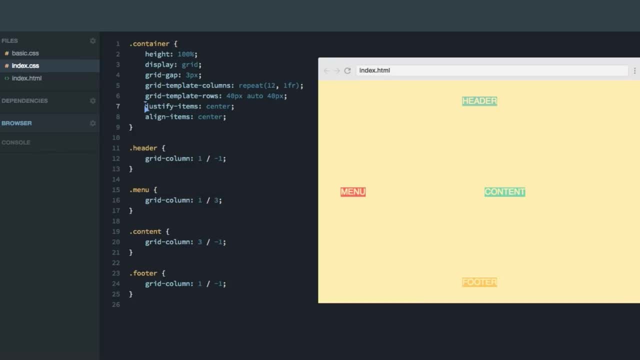 point of this screencast. Finally, let's comment out these two. Get back to the original layout And look at how you can do the same thing, though only targeting one of the items. Let's head into the content, for example. Then you can use justify self and do center. 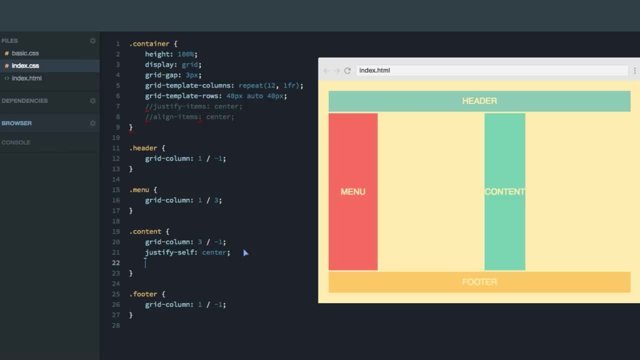 Now only the content is centered. Do align self as well, Do end. And now the content is squeezed down to this tiny little box in the bottom center of the huge space it originally occupied. A little bit sad actually to see the content being turned into a shadow of itself like that. 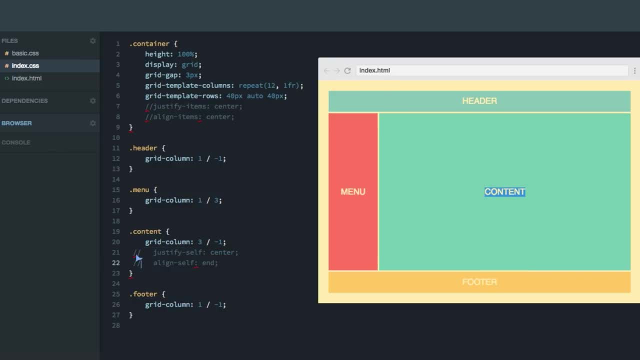 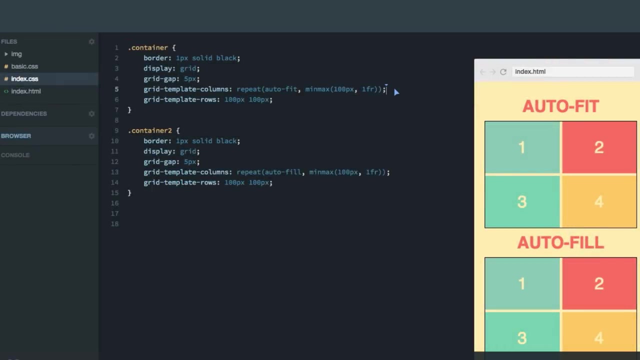 So let's give it back its original space, like that. Okay, so that was it. I hope you learned something and feel free to play around with this yourself. Thank you, Hey. in this screencast I'm going to explain the difference between auto fit and auto fill. So here, 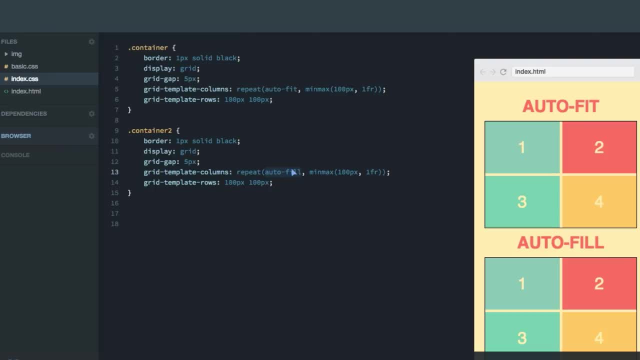 we have two different grids, using one or the other. you can see them on the page here And I'm assuming that you understand the basics of this complicated expression here- where we're basically repeating with auto fit as many columns as we can fit into the grid Given these constraints. 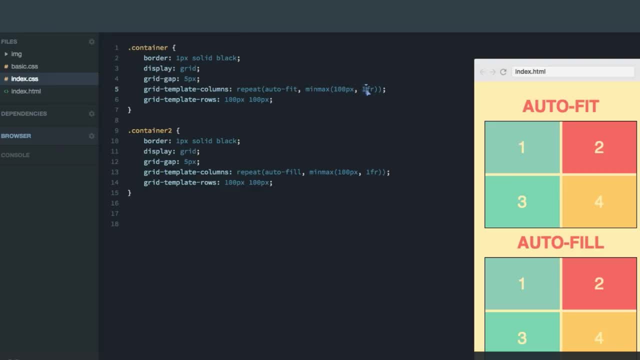 here they should be minimum 100 pixels and maximum one fraction unit And that, as you probably remember from the screencast in the second section, will give a nice responsive behavior where the amount of columns grows with the second section. So here we have two different grids using. 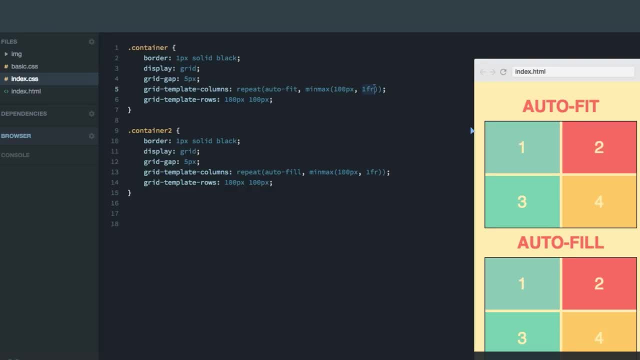 one or the other. You can see them on the page here and I'm assuming that you understand the basics of this. amount of columns grows with the size of the grid, like this: if we enlarge in this page, boom there, the grid crossed the 300 pixel threshold, meaning it could fit three columns in instead of two. 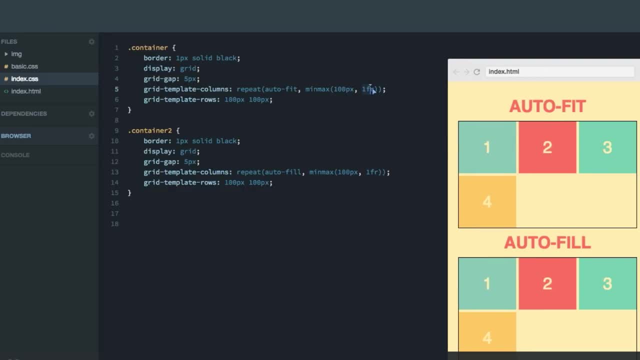 And as we make it more wide, the columns become one fraction unit until it reaches the next threshold, which is 400 pixels, and boom, then auto fit and auto fill adds another column to the grid, since we now can fit 400 pixel columns into the grid. However, there's a slight difference. 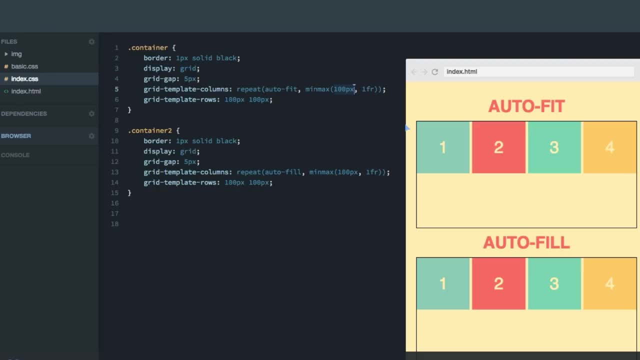 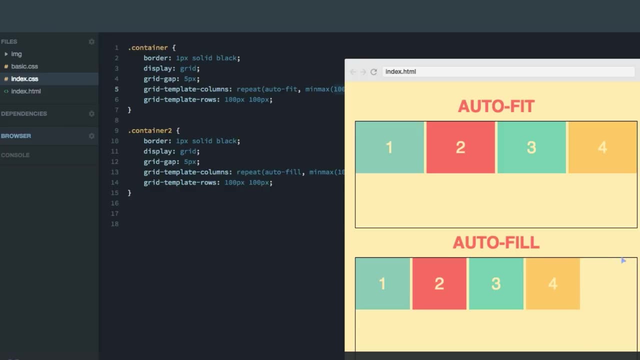 between the two, and that'll be apparent if we try to enlarge the grid even more, like this. Now, what you can see in that auto fill actually added a fifth column, even though we don't have a fifth element to add there, whereas auto fit made sure that the four items we have actually 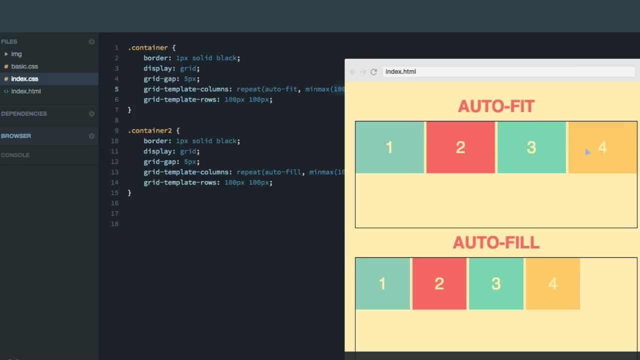 fit the grid. Now, under the hood, what's happening here is actually that both of them actually fit the grid. So we can see that the four items we have actually fit the grid Add new column tracks- though auto fit actually collapses those new columns to zero pixels in. 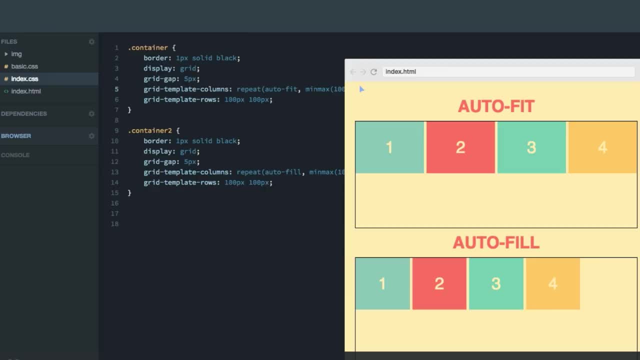 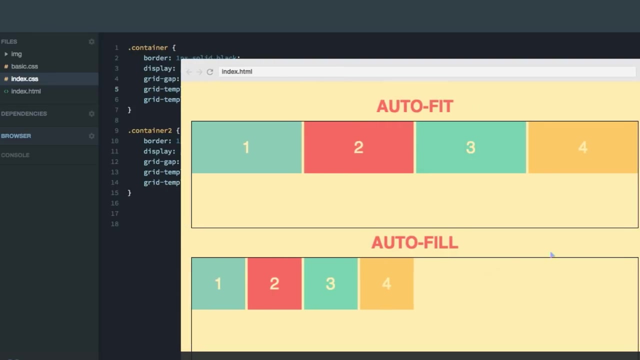 width, so that the current items you have in the grid, when defined like this with a maximum size of one fraction unit, actually will fit to the grid regardless, Whereas auto fill at every 100 threshold, like there and there, and there it'll add new column tracks which, basically, are empty. 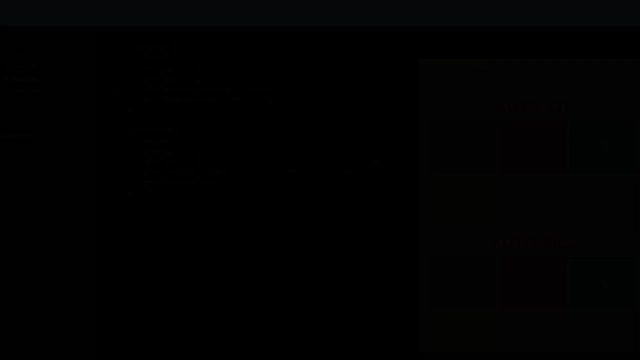 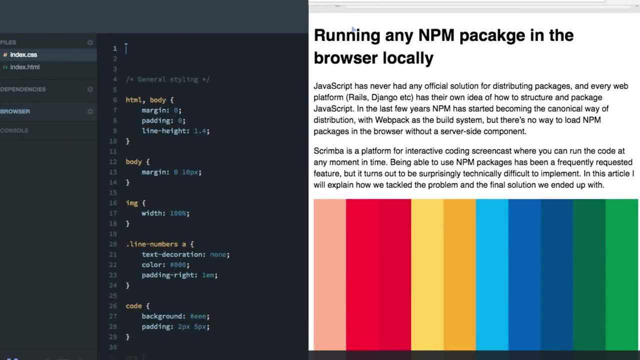 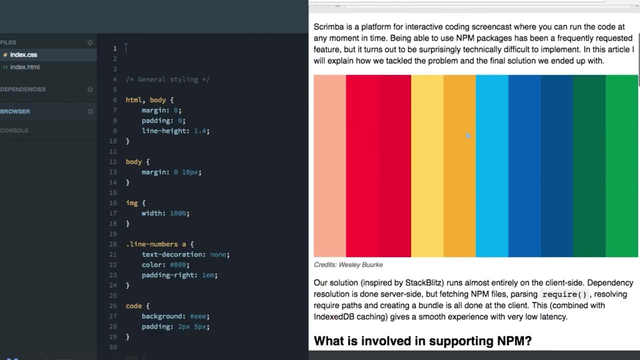 So that was the difference between auto fit and auto fill. In this example I will show you how you can use CSS grids to create an article layout. So in this example I have a plain article that I've written. I wrote it originally in Markdown. 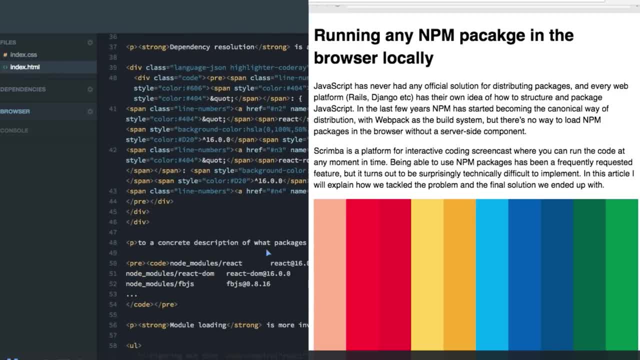 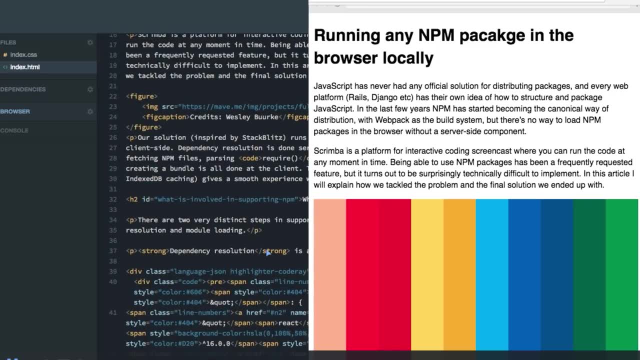 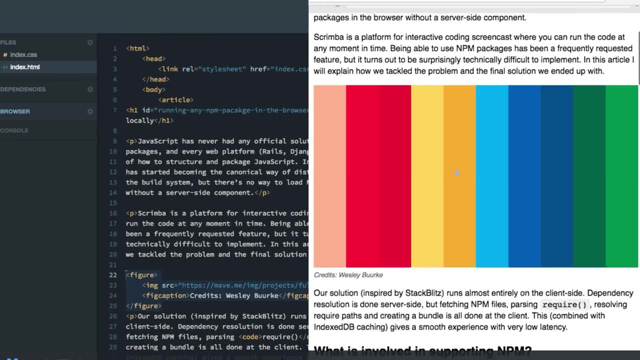 and then I generated this HTML using a Markdown compiler. So it's pretty nice. It has ULs, it has some P's And there's a div here for the code highlighting and a figure tag for the image and just basic HTML. 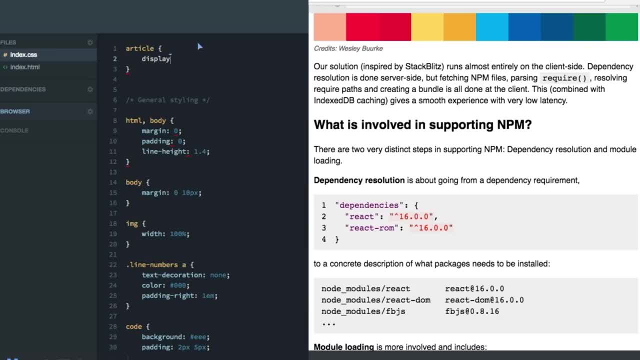 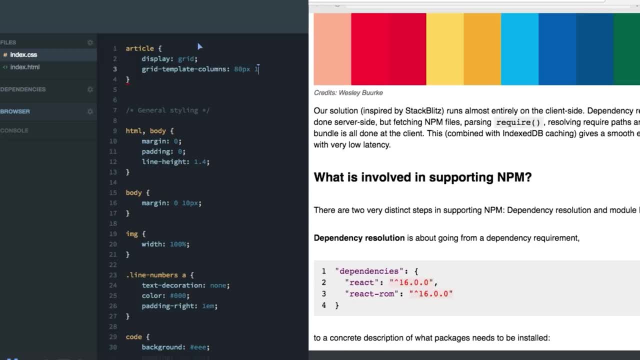 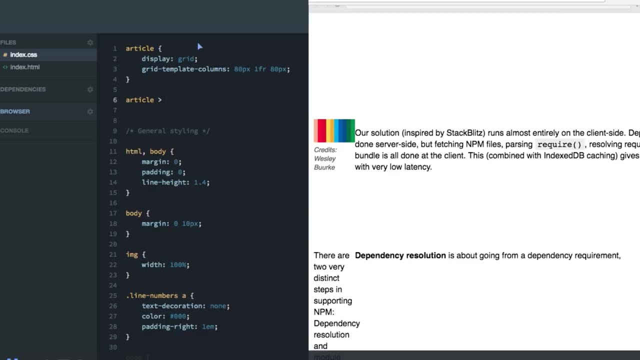 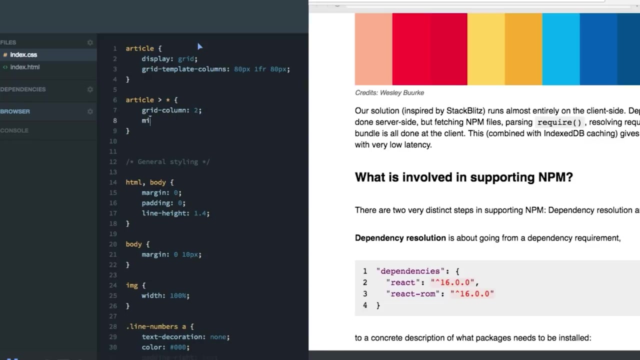 And I'm just going to go straight ahead and turn this into grid and then I will explain what I'm trying to accomplish with that. So now it looks. now we have a grid which is very funky. I just move everything where I want it, I want them to be, and there we go. 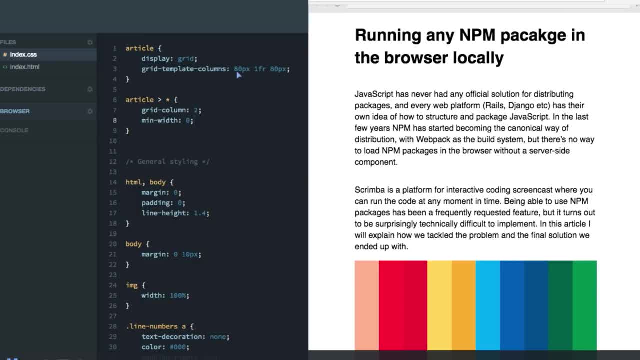 So now I've defined the grid, which has three columns. There is the first column, that's 80 pixels, Then there's a main column that takes one fraction of the space, And then there's the right column that takes 80 pixels. 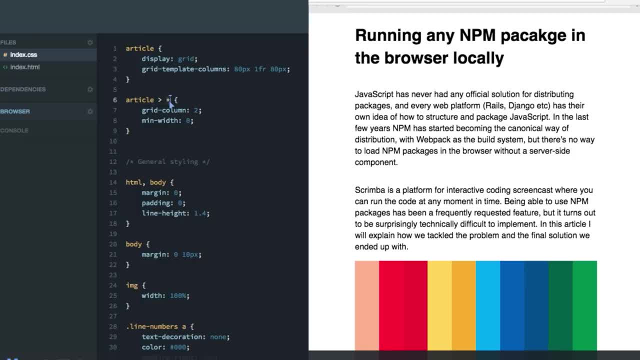 And I have this rule here which says that every element inside the element it takes 80 pixels. article should start at the grid, column line number 2.. So remember that the grid 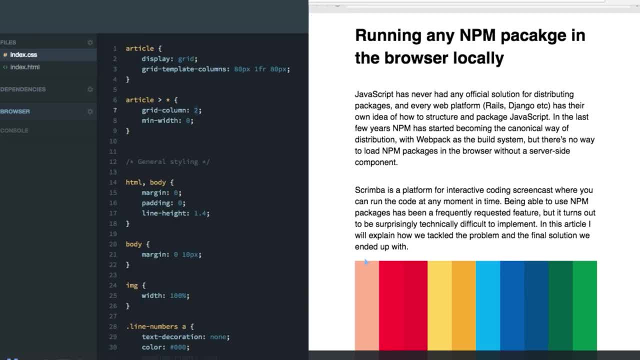 column line 1 goes down here, 2 goes down here, then we have 3 over here and 4 over there, And by setting grid- column 2, we say that every element should start in this column and we need to set the min-width to 0 to actually allow it to. 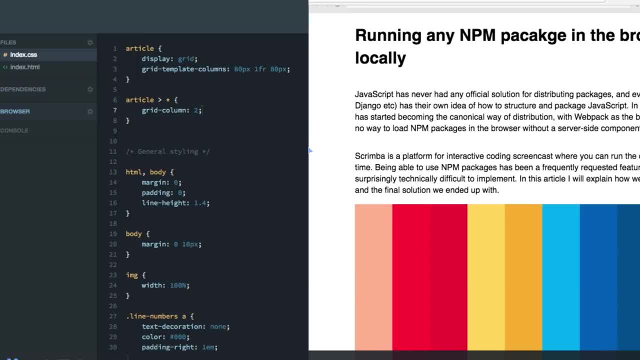 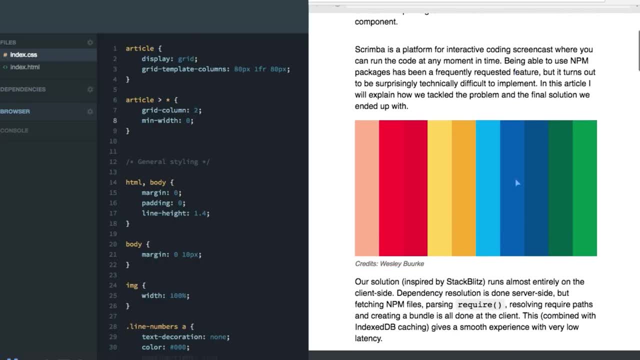 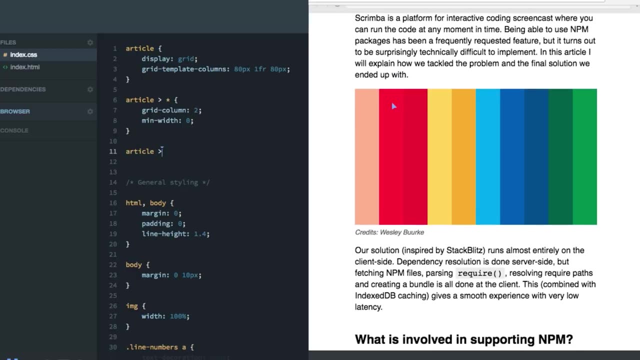 shrink. If we don't set this, you will see that it goes all the way over there. Now, right now, this is just a way of adding some spaces on the side, but since this is a grid, we can now do some things very easily, Since I now want this figure. 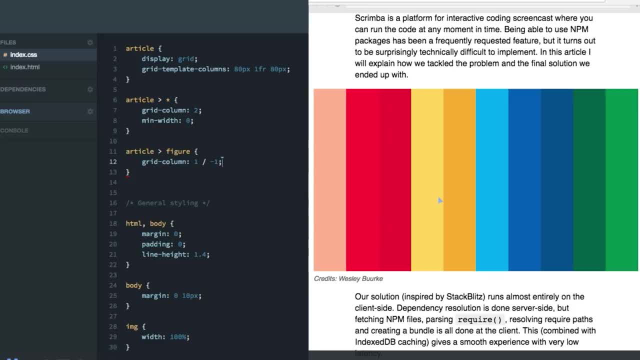 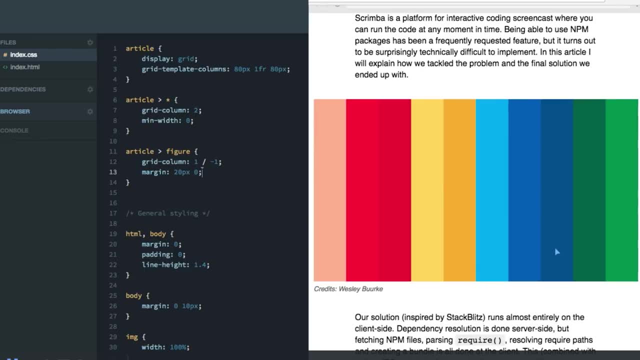 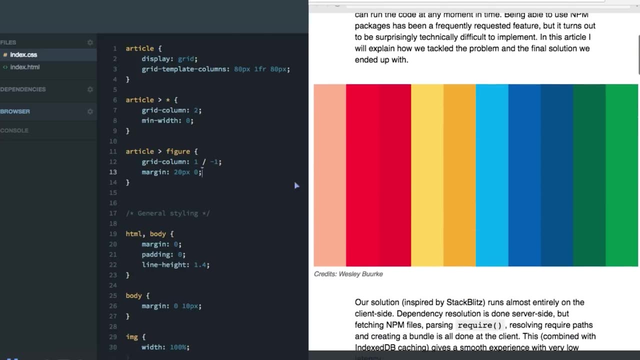 take the whole width, and that was all. And let's add some space on top of it. Wait, a second Right. So what did we do here? I set the grid column to start at line 1, and end at line minus 1, which is the last one. So this is the way of saying: make the element. 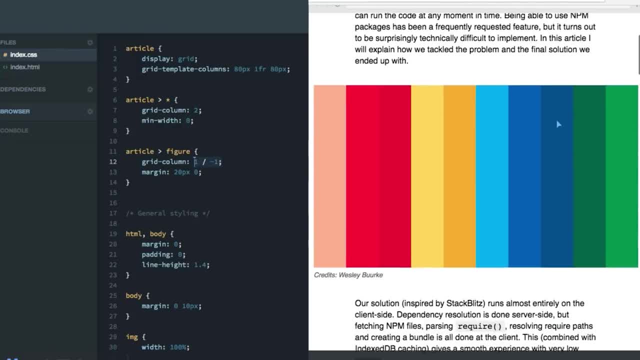 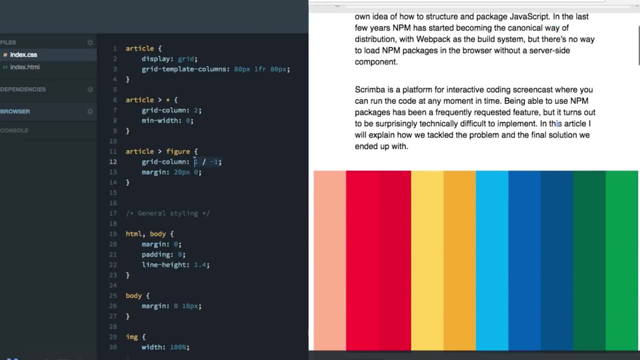 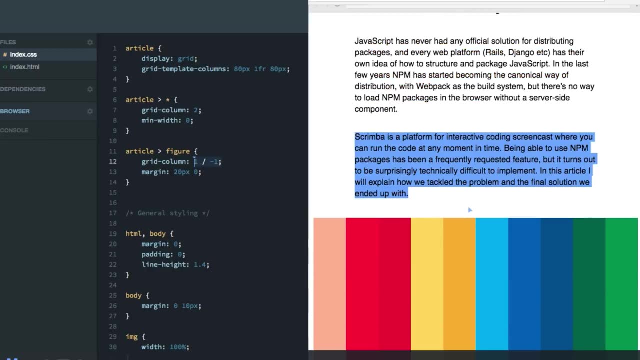 take the whole width, And this is just radically simpler than any other way to accomplish the same thing. If you don't have a CSS grid, you end up having to say that these elements here should have a margin, a standard margin and a 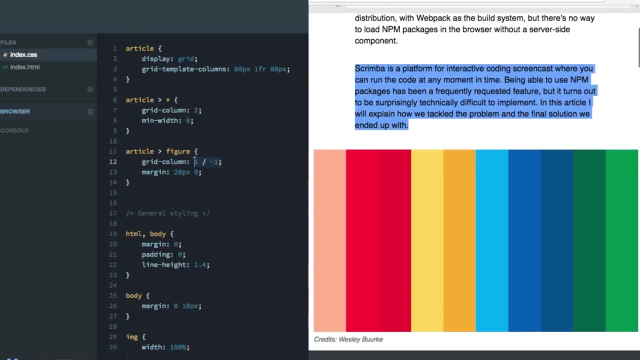 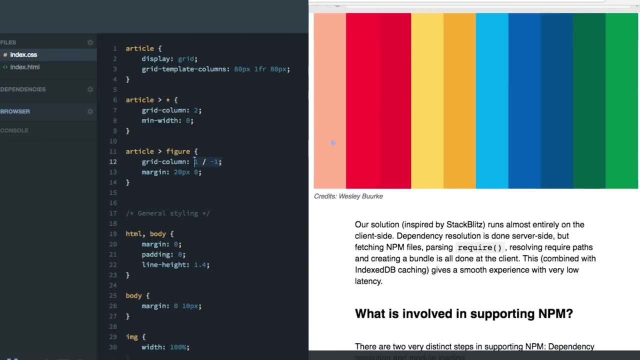 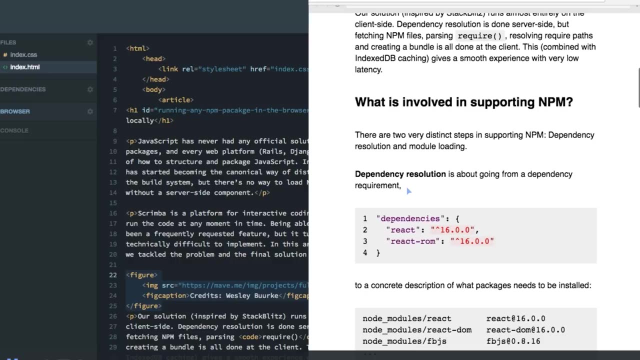 margin And this should not cancel out the margin you set by default. And often this is very tricky because you often end up having to have custom HTML just to handle where things should, when they should be narrow and when they should be wide, And it can be really tricky. 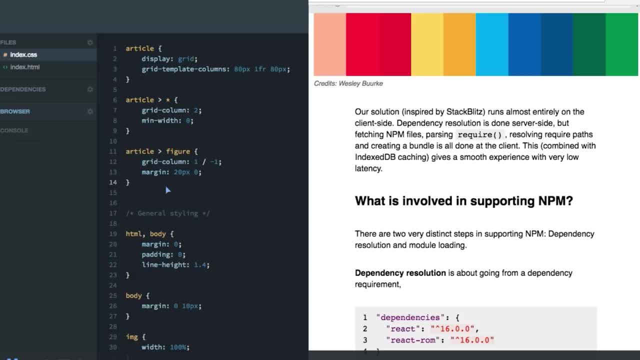 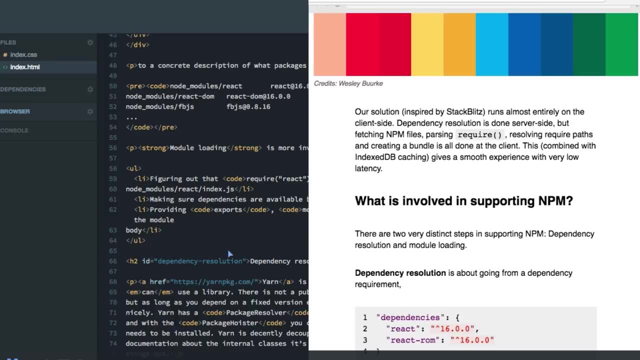 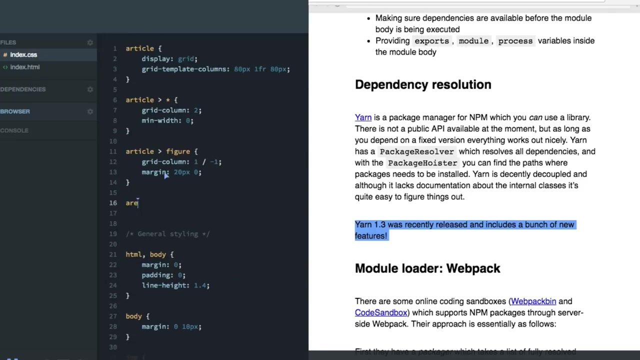 deciding where to put things. So another thing that we can do is to add another element. I'm going to call it a side, And here I'm going to just write subtext, And it includes a bunch of new elements. Now we have this new paragraph over here, And now I can style it. 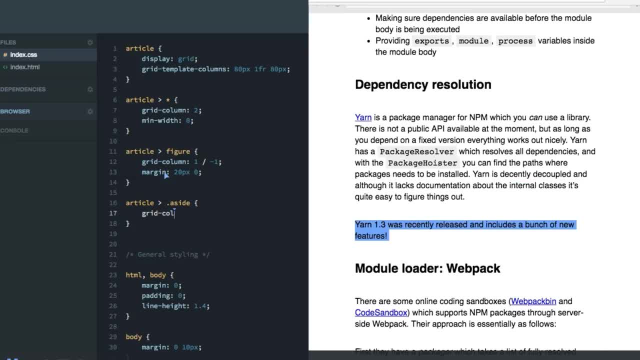 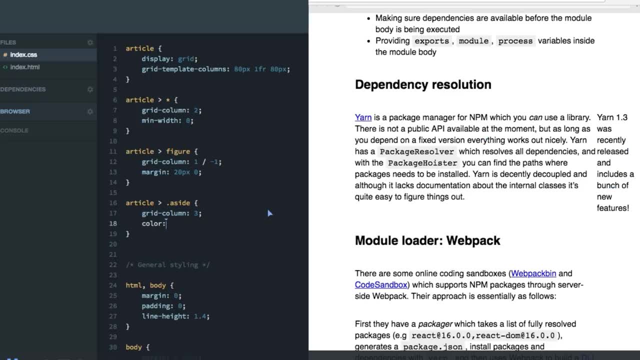 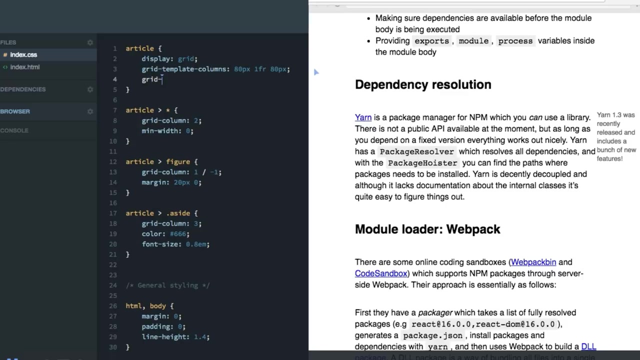 And now I want to style it like this, I want to say it in the third column, I want it to have like a gray color And a note like that And a smaller font size, And this seems like a good time to add a gap spacing between 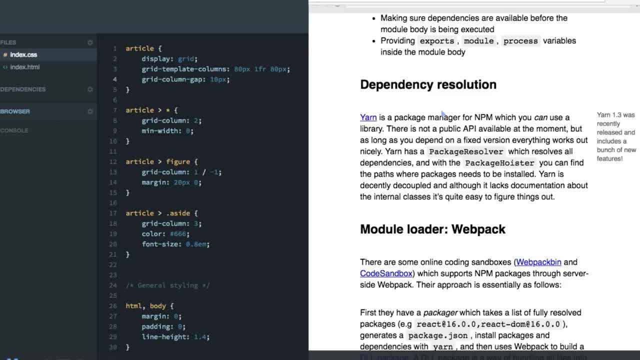 So yeah, And if I want it to be on the left side, I can just set it to grid and press me. If you're trying to do this without a grid, it's so hacky I can't even begin to think, Because you have this element here, which 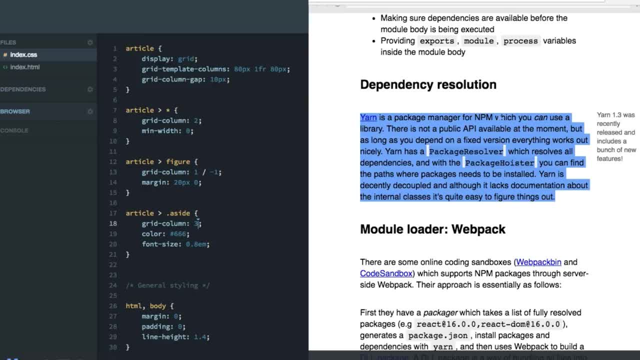 originally has a margin. And then maybe if you put both of these elements inside the same div, maybe you can do like position absolute and set left 100 or something. yeah, i don't know, i don't really know. this is just something i don't know: a clean way of doing in plain css. 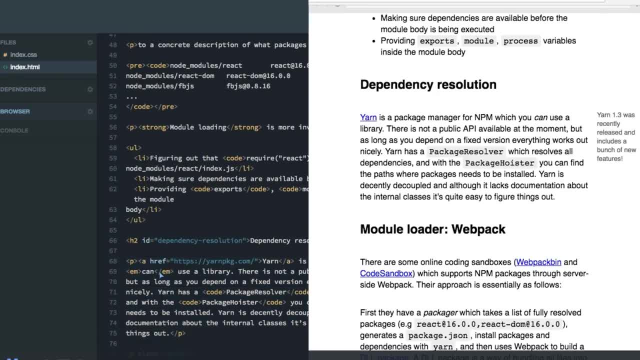 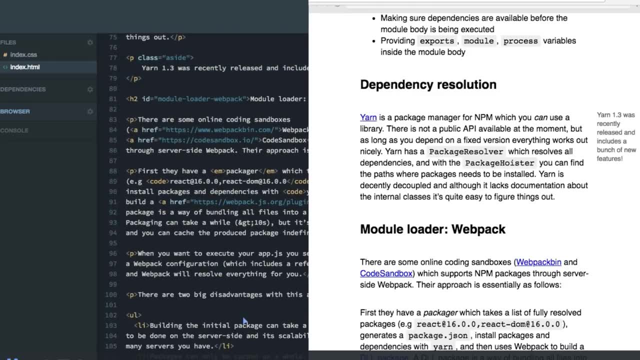 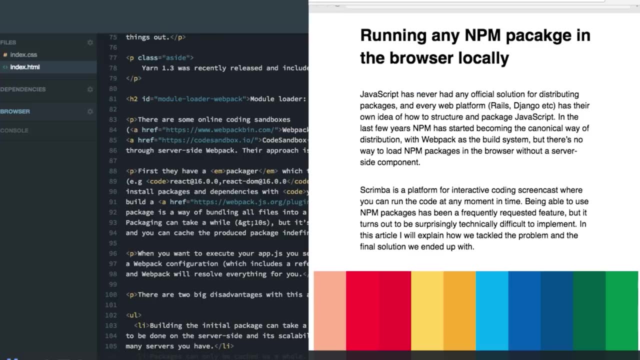 and especially not in a way where you can have no changes in the html. basically, now there's one thing you need to know, and that is: this is actually a separate grid, so this is becoming a grid row that goes here and this is a separate grid row, and this has the consequence. 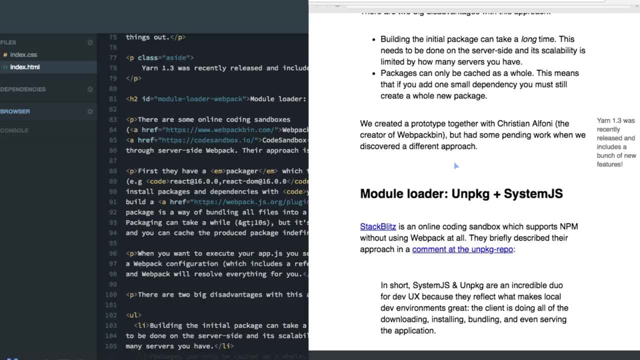 that you often end up with this spaces. you might, in this case, want this space to be gone and then this text to go down further to the right side of the header, but that's currently not possible with css grid. that's just a limitation that you can't really avoid. 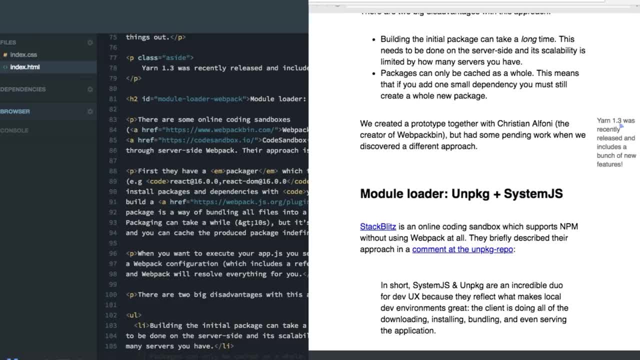 and whether it's good or bad, i don't really know. in this case i don't think it's that bad because this paragraph belongs with this paragraph and here we have a header which starts a completely new section, so it's not that big a problem. but if we had, like, another paragraph over here, it can be a bit confusing. 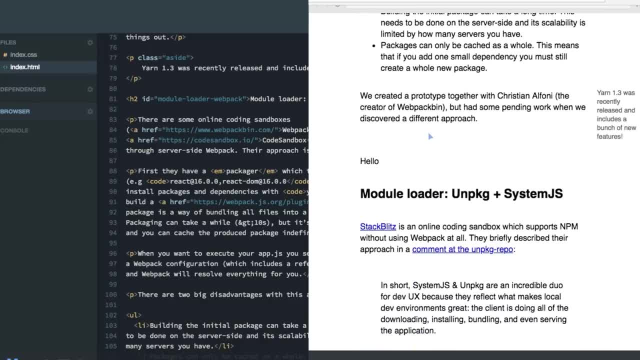 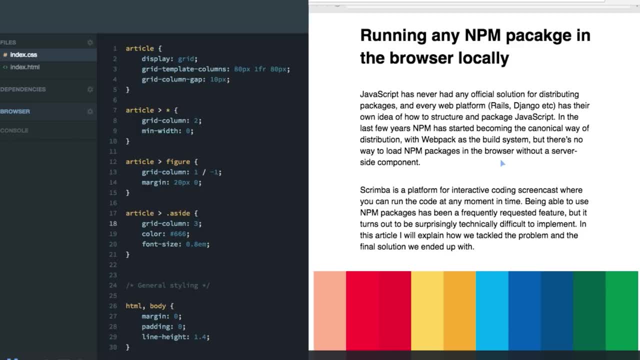 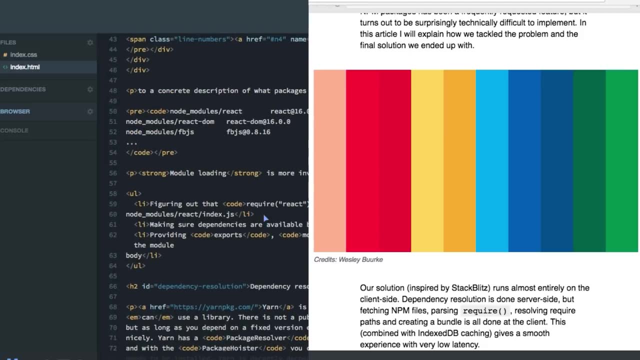 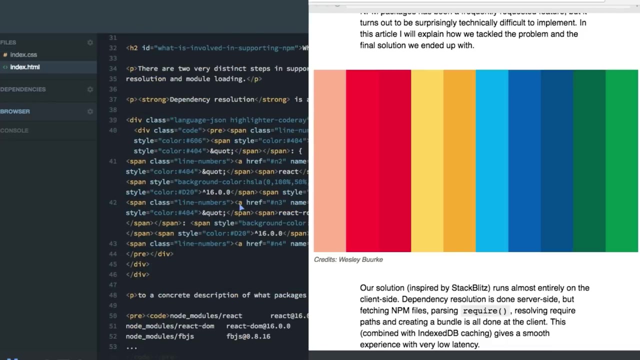 that you have these big spaces, which isn't quite optimal. but other than that, i find that using css grid for this type of article layout makes the the html much cleaner. you can basically just take the output from a markdown parser and dump it straight in. you don't need to do anything special to support. 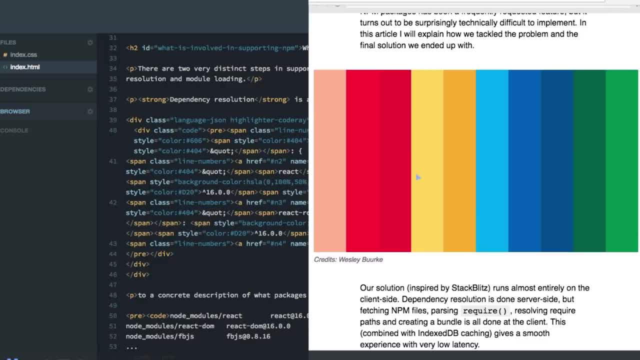 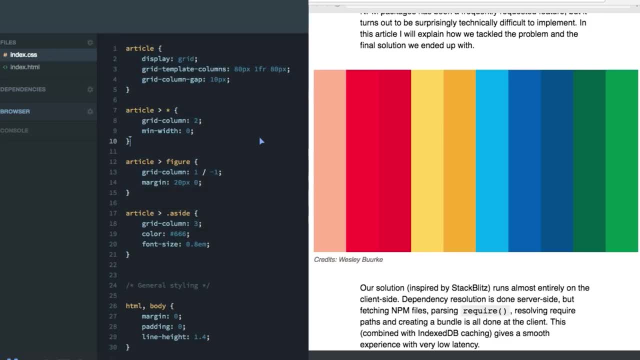 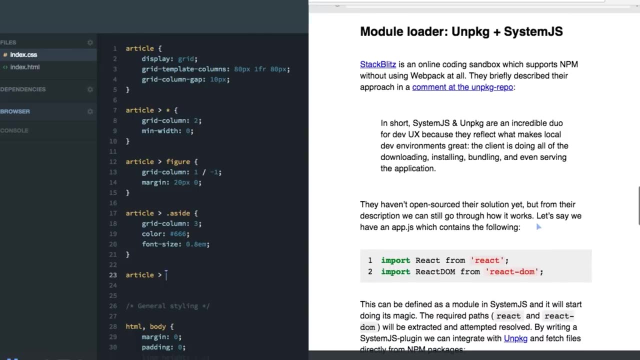 either having things in the left column or the right column or in in full width, and the styling itself. it's 20 lines, um, and even here i haven't touched anything like block quotes, but here's the quote. maybe you also want that to be in the full width. 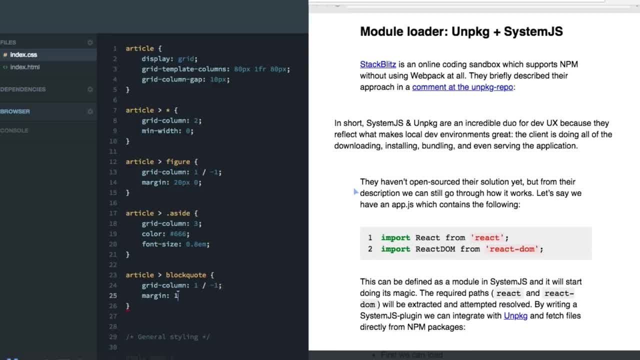 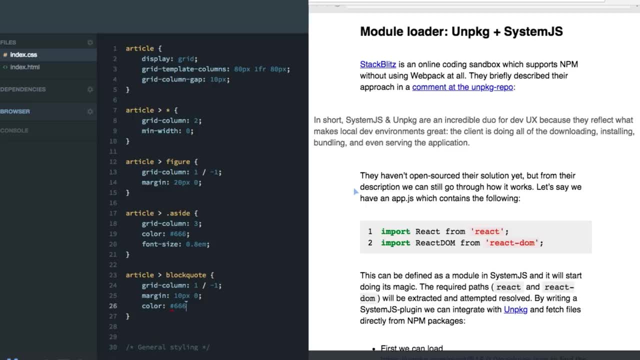 oh, we should remove the margin at the side and maybe we want to set a color once again and maybe like: border to the left is cool, solid things like that as well- and notice that i can just add padding, add borders. i just set the column to be from one to minus one and everything works. 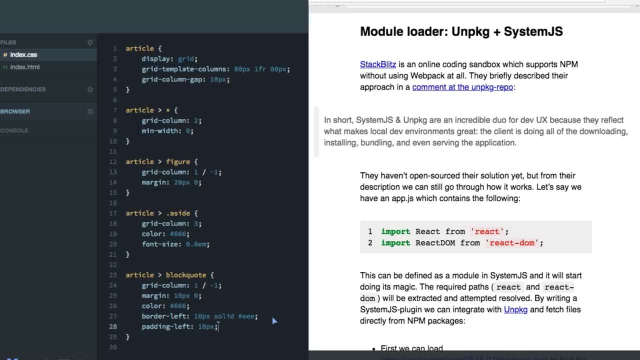 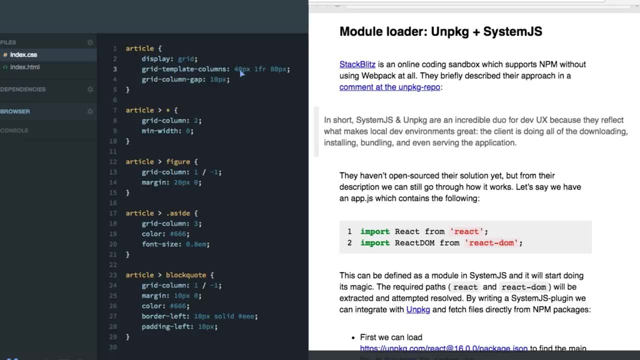 i don't need to worry about negative margins or or or, knowing what the width of this column is. so now, if i want to set the left column to be 17 instead, or maybe 40, and the right one to be 40, that works perfectly fine. 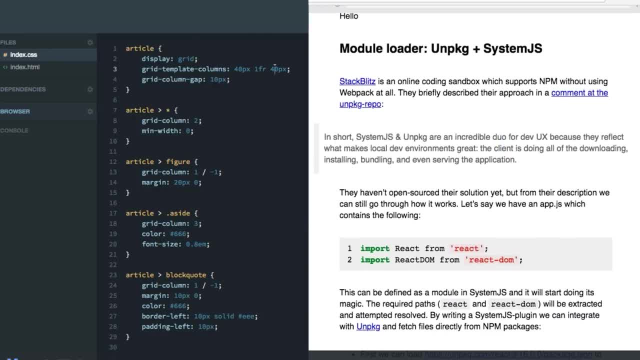 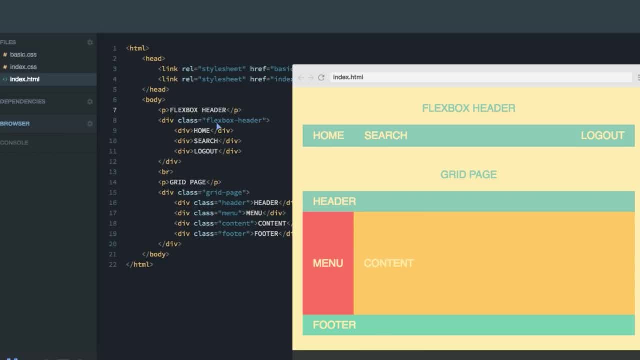 and all is just very, very good. thanks screencast. i'm going to talk about the difference between flexbox and grid, and i'm also going to show you how you can use the two together. so we have a header here which is built using flexbox, and a page layout which is built 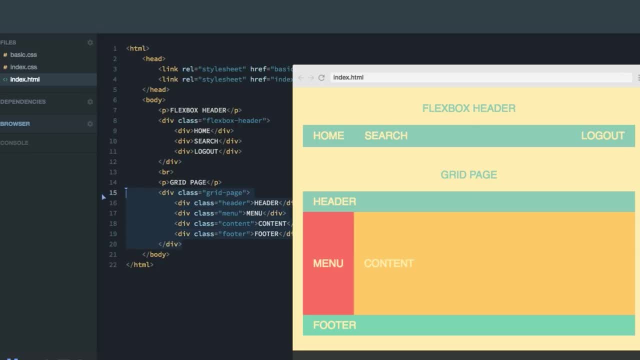 using css grid. here is the html for the grid example and the html for the flexbox example, and the css is located in the indexcss file here, and we're going to look at this code in a minute. however, let's first look at the examples themselves, because you might actually be able to. 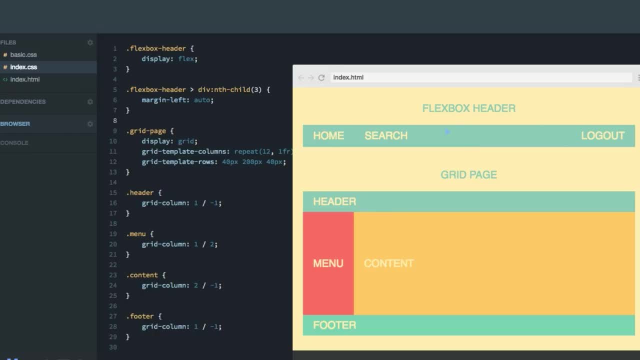 guess the main difference between flexbox and grid just by looking at these two examples. because flexbox is built for one dimensional layout like this one goes in one direction, from left to right being just a single row, whereas css grid is built for two-dimensional layouts like this page here. 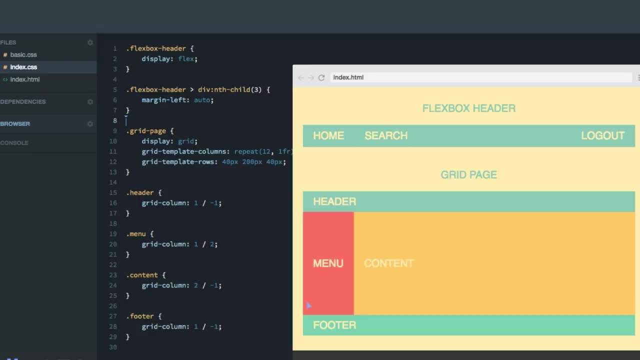 it has three rows: the top one, the middle one and the bottom one. that actually has 12 columns, though we can only see two of them visually here due to how we've laid out the items. so if you're going to create layout which has a direction, either row or column- then use flexbox. it's great. 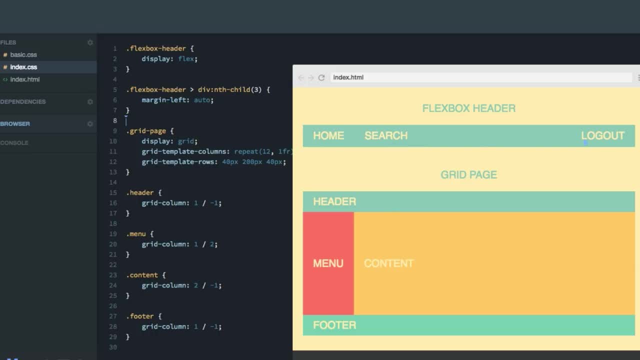 for aligning content within that container and gives you a lot of flexibility. however, if you're going to create a more overall layout with both rows and columns, then you should definitely use css grid, as it'll give you much more flexibility and simpler markup than if you were to, for example, 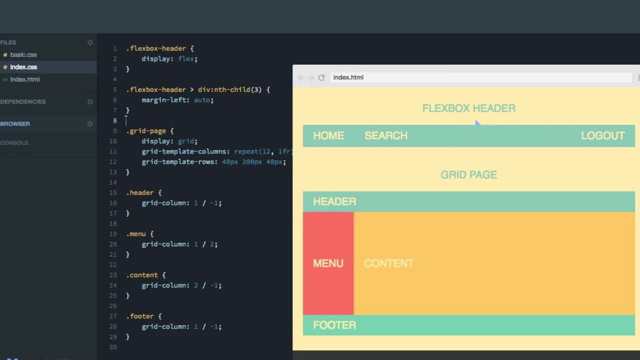 try to use flexbox to create two-dimensional layouts. okay, there's also another overall difference, which is that flexbox takes basis in the content- it's so-called content- first, whereas grid is layout first. it takes spaces in the layout. now this might seem a little bit abstract, so let's. 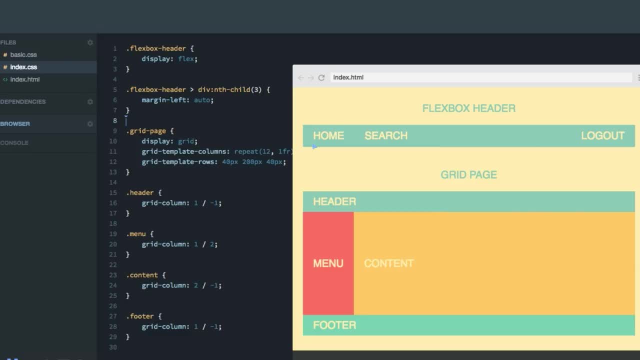 look into the code, because that'll make it a bit more clear. so the flexbox header here is turned into a simple box by simply giving it a display flex. you don't have to do anything else. we then let the content make most of the decisions of where they're going to be placed throughout the 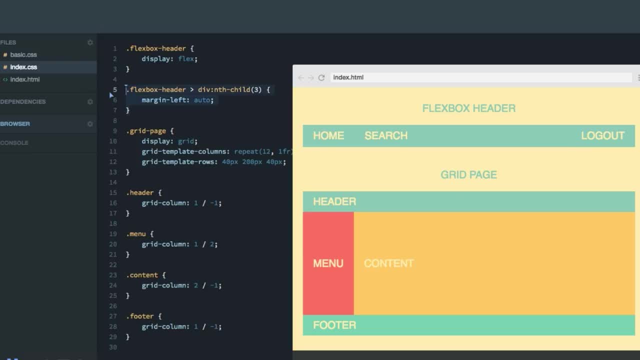 container. for example, you can see the third child here. the logout element simply adds a margin to its left hand side and thereby shoving itself all the way to the end of the container. now let's look at how we create our grid layout. first of all, we can't just simply give it a display grid and then 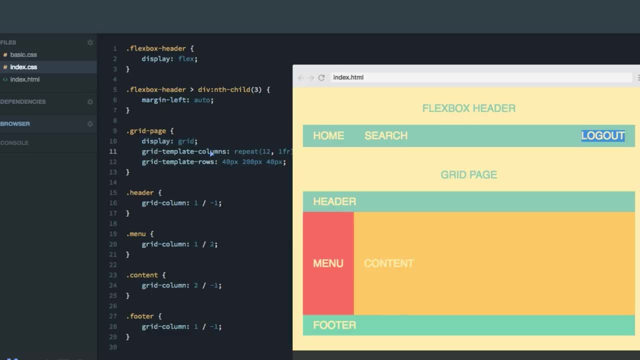 content into the container. no, we also have to define either columns or rows or both, as we're doing here. we're giving it 12 columns, each being a fraction unit wide, and three rows, and just by doing this you can understand that grid to a larger degree takes basis in the layout. first, you're. 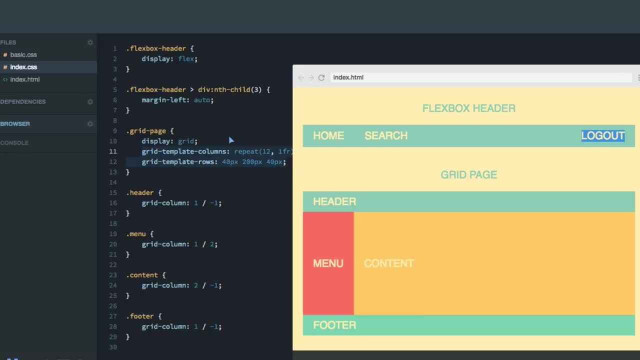 constrained by the layout you define here. whereas we could have added as many items in the width on this single row in our header here, we're now constrained with 12 columns in our grid example here, and also we need to place the elements according to the layout. 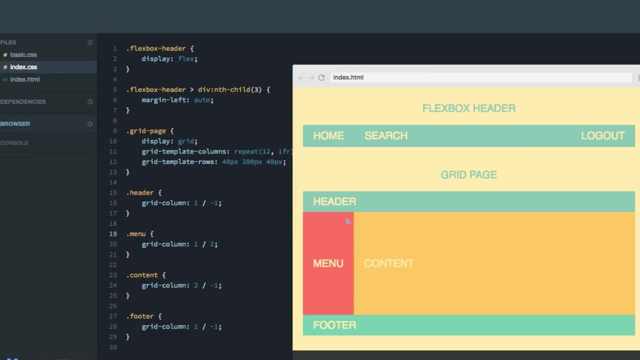 for example, this menu item here, this one which you can see on the left hand side here. we're not placing it here by giving it a margin on its right hand side, like we do on the logout. we're taking basis in the layout and saying that we wanted to span from the first column line to the second. 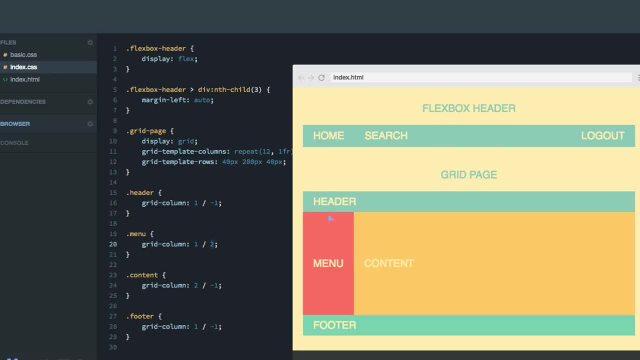 column line, and thereby it places itself how we want this layout first versus content first is a abstract, and it's not something you think about when you develop, though it's nice to be aware of it. so, finally, let's actually combine the two, because that's what you want to do. you want to 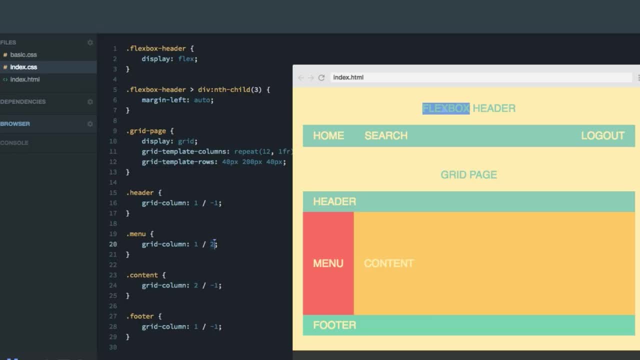 combine css grid with flexbox and then get the best of both worlds. so now what we're going to do? we're going to take this header here, move it down into our edge layout. so let's head over to the html and take the three elements here, copy them and add them here. 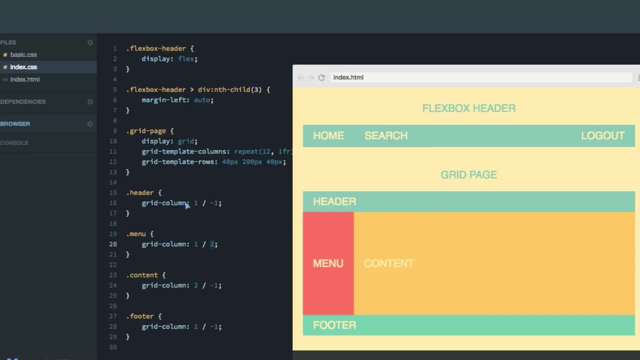 like that. so what we now will do is we'll turn the header here into a flexbox, giving it a display of flex. now let's run this code. as you can see, we have the items laid out like this. what we now can do is we can use, for example, justify content. 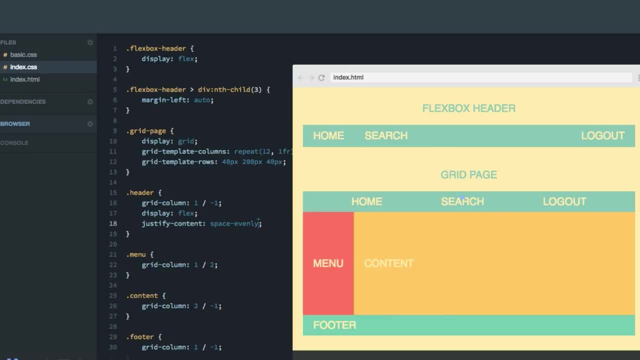 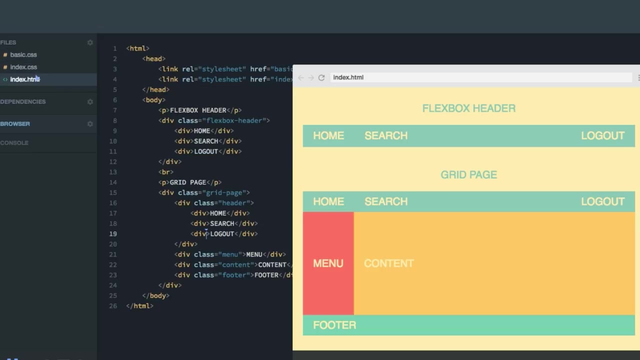 do, for example, space evenly like that. as you can see, they change accordingly. however, let's do a what we did in the flexbox layout: target the third child log out button, margin left auto. as easy as that. you've combined css grid with flexbox. now this header here, this item in the grid. 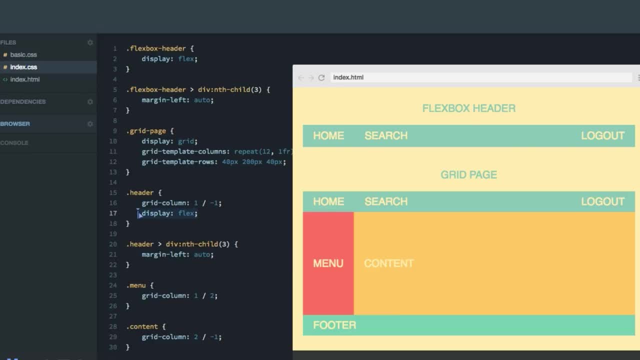 container is actually a flexbox header here. this item in the grid container is actually a flexbox flex container itself, which then again has three items within itself. so i hope you learned something from this and that you'll start using grid and flexbox together from now on. thank you. 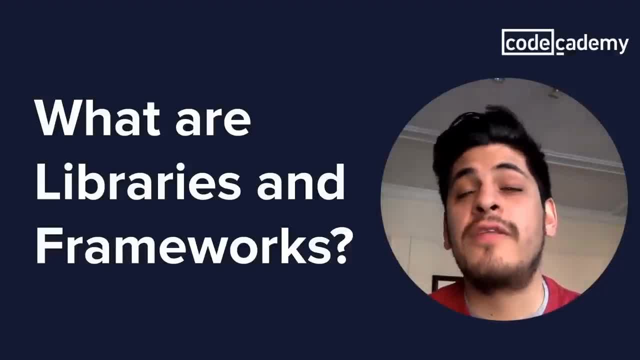 The terms framework and library are two terms that are used a lot in the tech industry. Many people use them interchangeably and don't really understand what they mean. So if you're on that boat, hopefully this video will help you out. So let's go ahead and get. 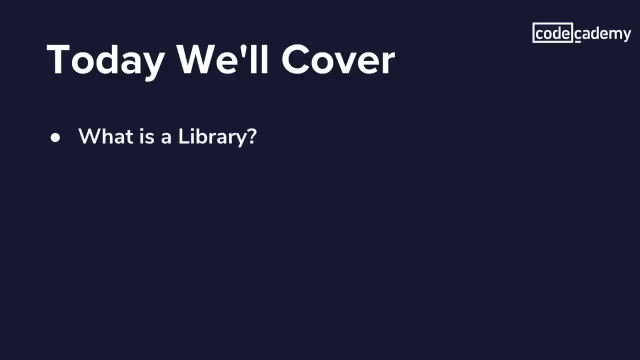 started. So today we're going to cover what is a library, what exactly is a framework, and then we're going to compare both of them and see what the actual difference is. So what exactly is a library? Well, in a gist, a library is a set of code. that was previously. 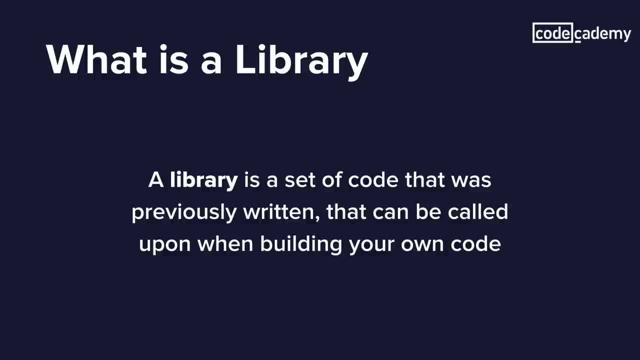 written that can be called upon when building your own code. So it's essentially a collection of code packed together that can be used over and over again, And it's a very good idea to put frequently used functions together and build yourself a library. One of those reasons is: 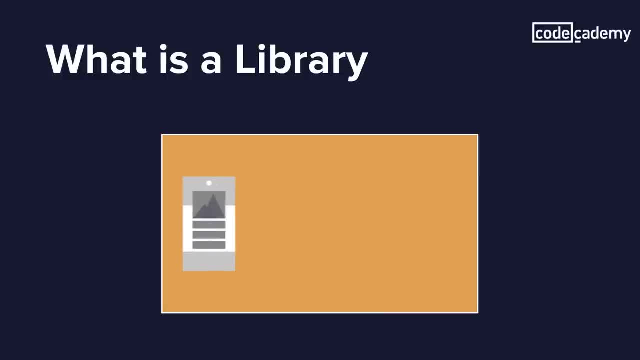 handling reusability. So reusability is one of the most important factors in software development. So whenever some method is used, you can simply make a method invocation using the library you just imported. So we can look at an example of how we import libraries and JavaScript. 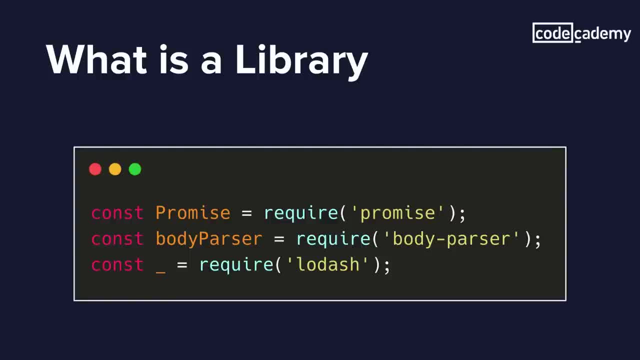 right over here. We're importing three different libraries- one called Promise, BodyParser and Lodash- And from there we can simply make calls to those libraries when they were actually needed. So let's go ahead and take a look at an example where we actually use a library. 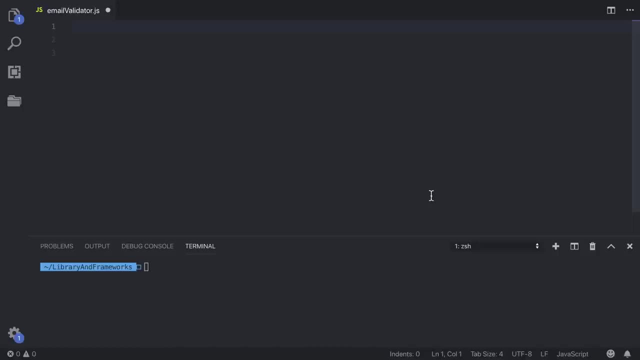 Now, let's say you're building an application where you need to register and sign up a bunch of users. In order to do that, the users must actually submit a valid email address when signing up. Now, there are many ways to do this, but most of the ways will actually involve using